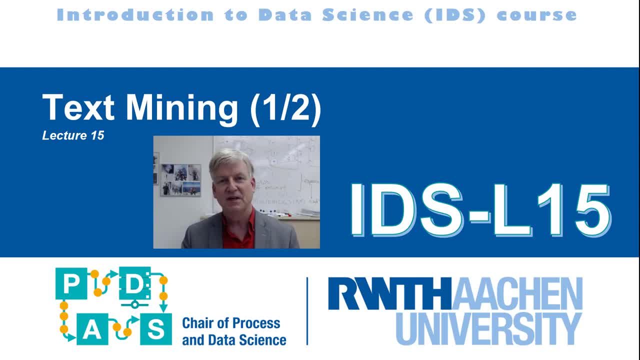 have specific characteristics. In this lecture, we are going to focus on text mining. There will be two lectures devoted to it And, just like process mining was focusing on temporal data, we now focus on textual data and try to use and exploit the specifics of text to create, let's say, a wide range. 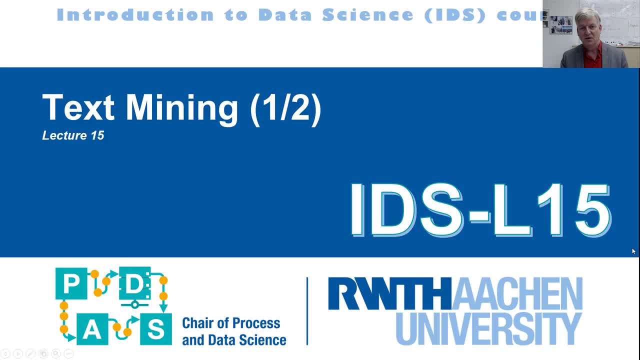 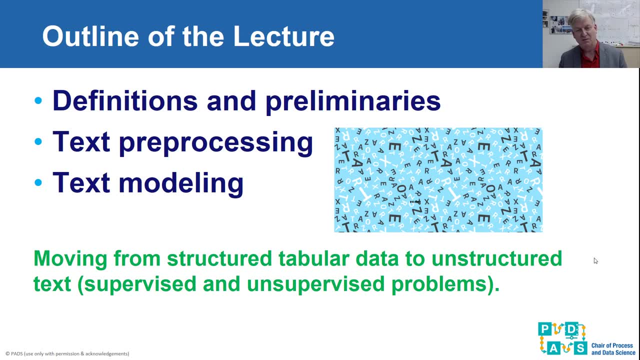 of data science problems. So what we will do today is that we will focus on the definitions and preliminaries- What is NLP, What is text mining? And then we will mostly talk about text pre-processing and we will end with the next lecture. Thank you very much for your attention. 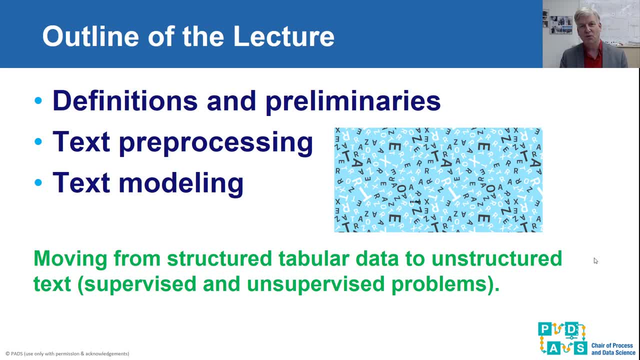 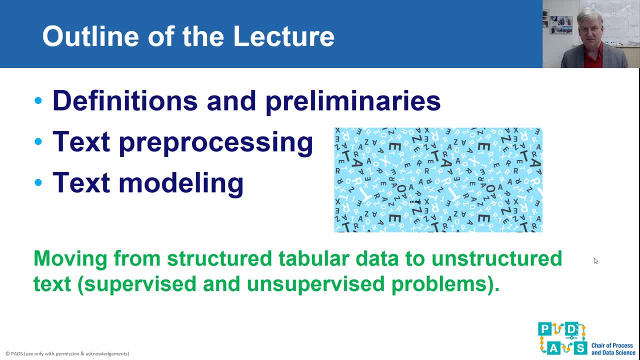 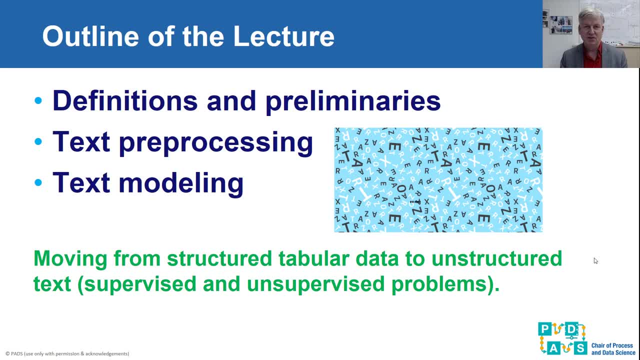 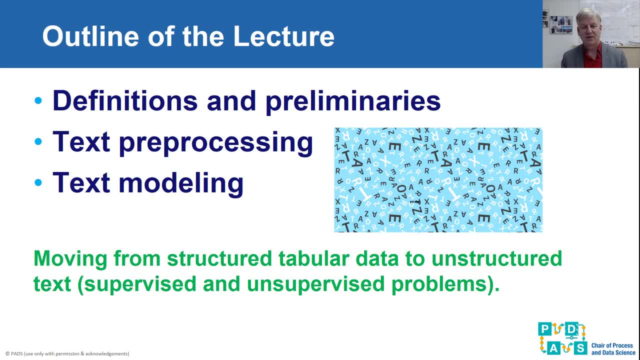 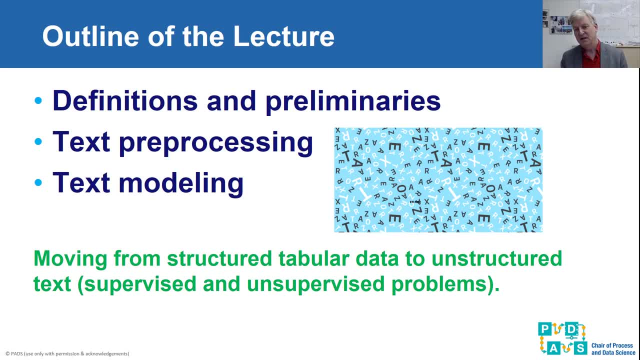 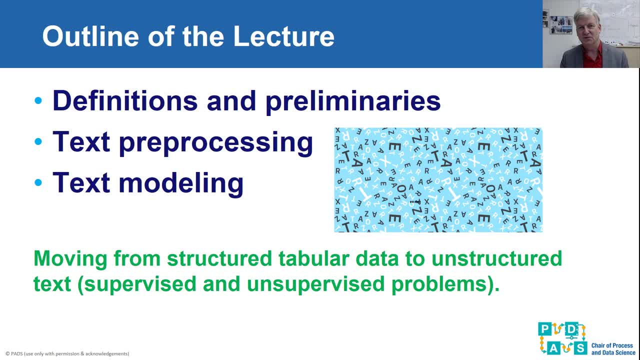 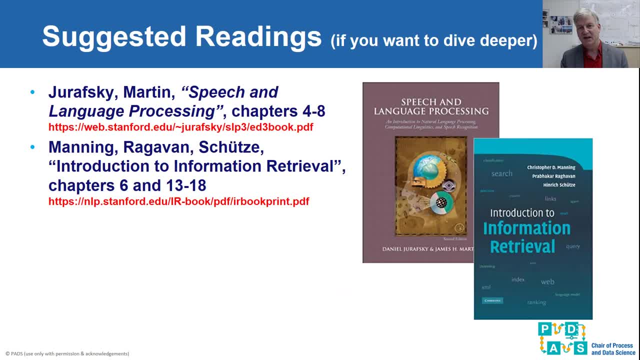 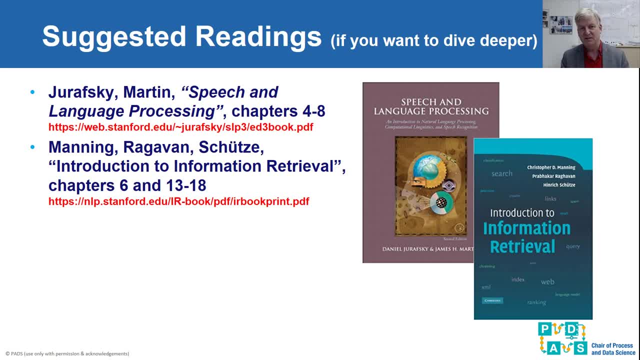 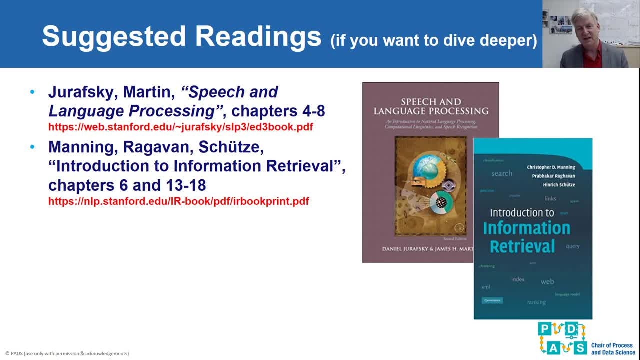 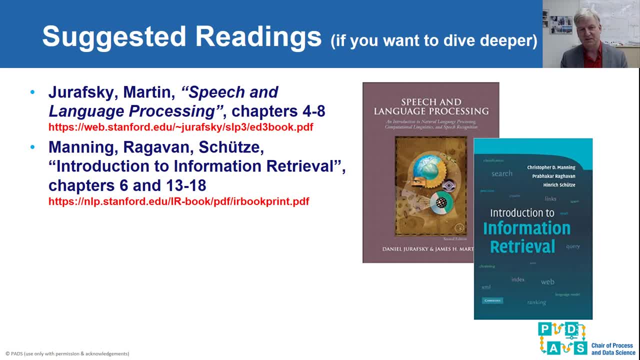 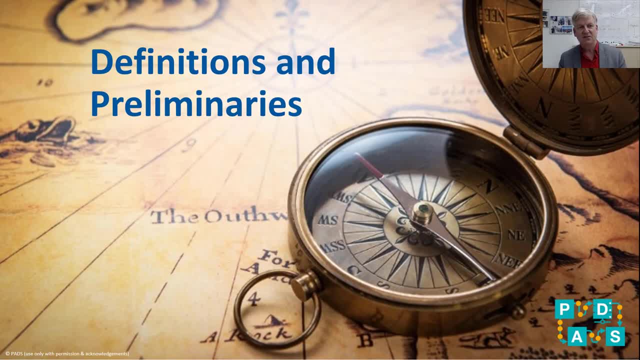 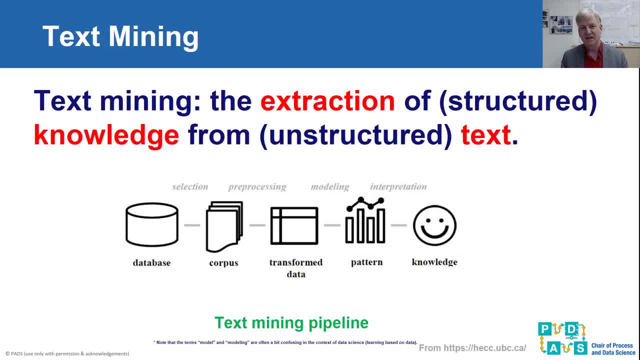 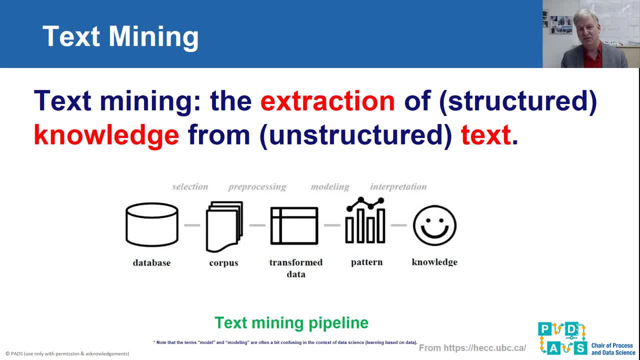 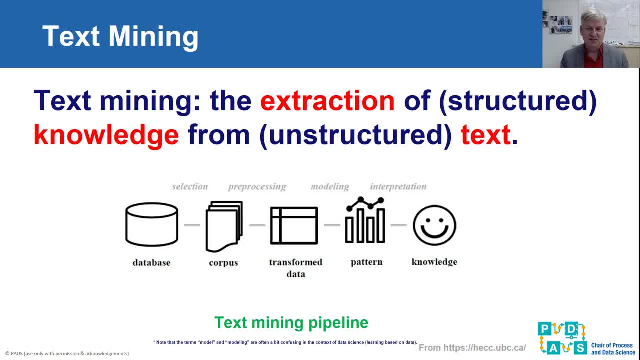 articles, that is what is on websites, that is what is in Trump's tweets. All of these things are text and we understand very well what text is, But text has specifics. For example, a text is composed of words. We have things like verbs and nouns, So we will exploit. let's say this: 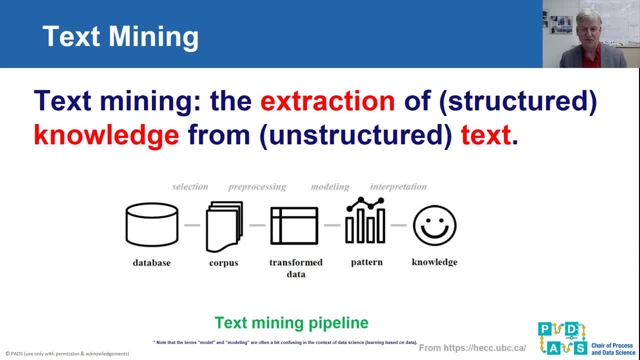 structure and, let's say, show how text mining is dealing with these things. So this is the text mining pipeline that we will use, let's say, throughout this lecture. So it starts with the database, with information, then we build a corpus. A corpus is an. 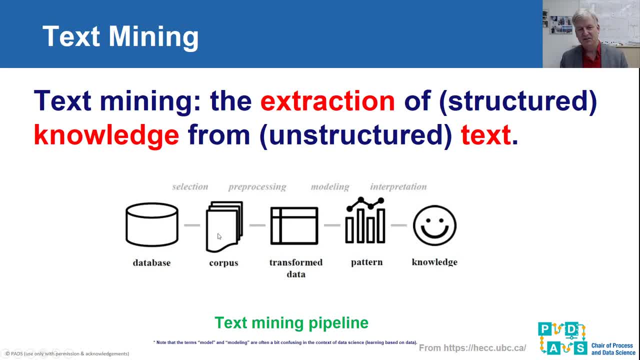 asset, For instance a set of documents, Then we transform these documents into data that we can somehow process And then we feed it to, let's say, many of the data science techniques that we have seen before. So, for example, once we have converted documents into vectors, we can, for example, use: 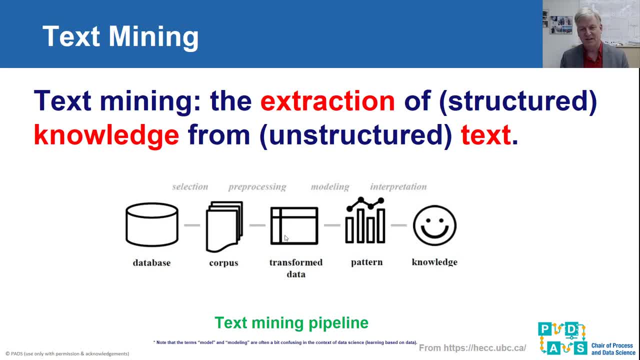 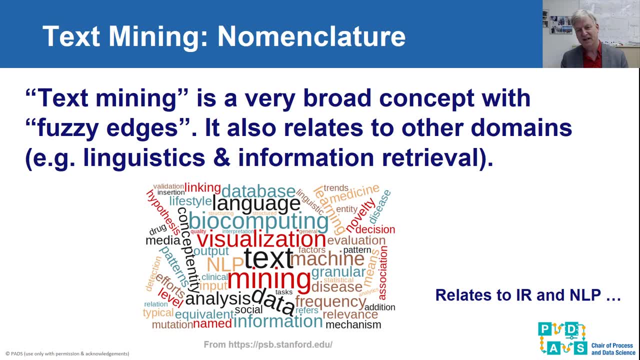 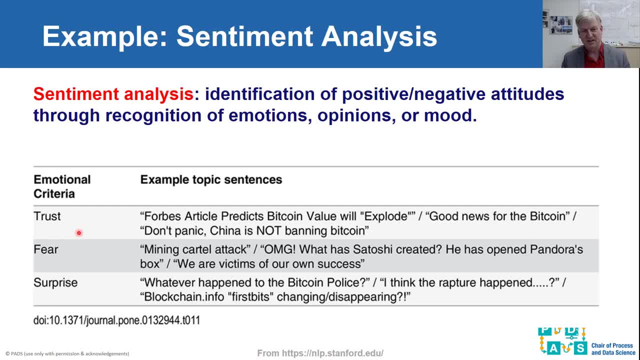 To, for example, once we have converted documents to a database, we can, for example, use neural networks techniques. This is a supervised learning problem. You can basically do that by training, for example, a neural network on these emotional criteria, And then, after that you've trained. 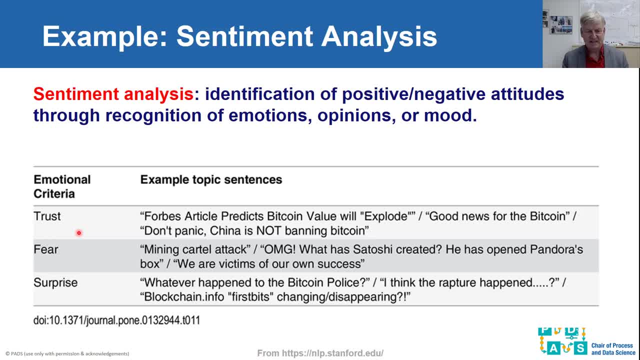 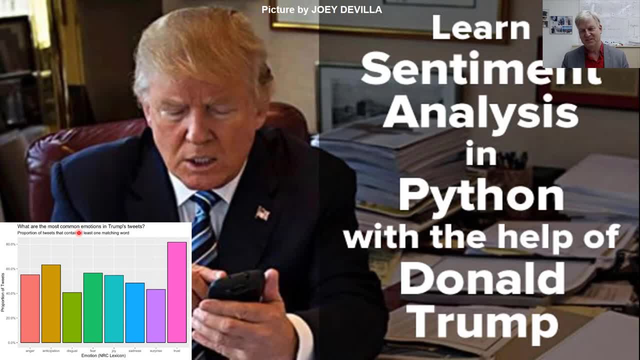 such a neural network, you can basically classify tweets in a particular way. Of course, a nice example would be the tweets of Donald Trump. So there have been, let's say, several research papers on analyzing Trump's tweets And of course, this is a nice application for sentiment. 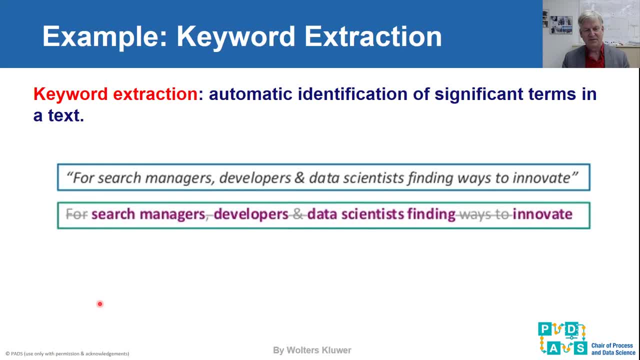 analysis. Then there is keyword expression. The language contains- and I will come back to that extensively contains- many things that are not so relevant. So D A, 4,, 2, these are all words that will appear in any document. 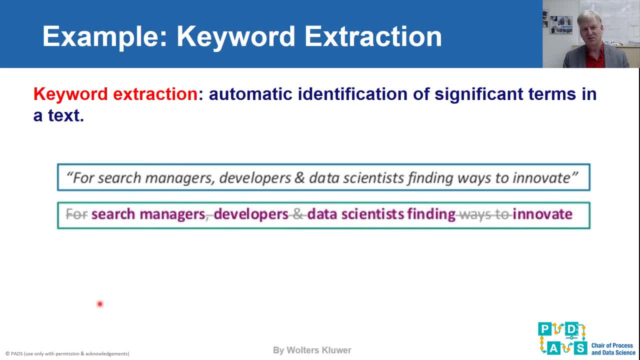 So D, A, 4,, 2, these are all words that will appear in any document. So there is no point in, for example, trying to classify a document based on words that appear in any document. Also, if we are extracting keywords, we are of course interested in 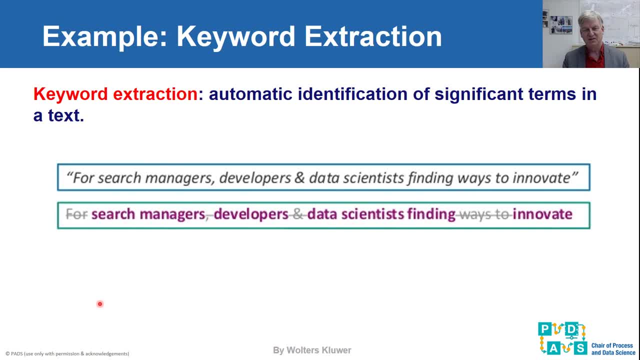 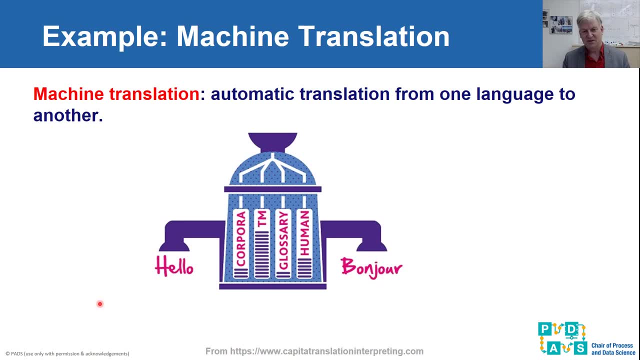 the words that really tell something about the underlying document. Machine translation. I think most of you have seen that that works pretty well today. That's another example of in the field of NLP and text mining, where we have sentences, we try to capture what 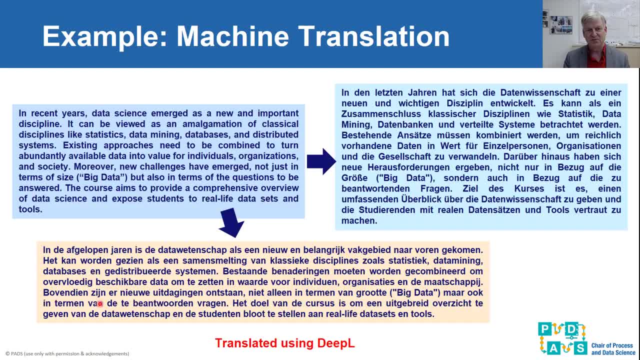 they mean, and then we try to convert that to another language. Here you can see like an illustration that these things work today, let's say, reasonably well. So here I started with the text in English and I'm showing the German and the Dutch translation And 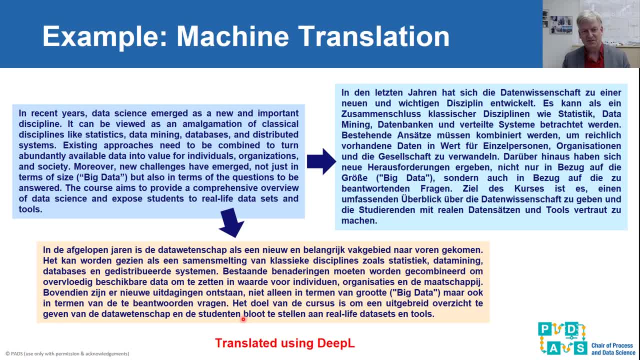 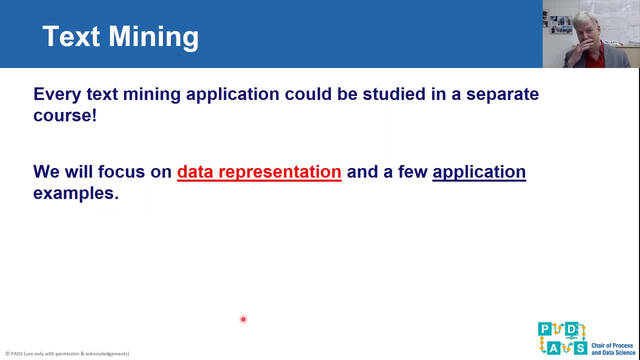 it's far from perfect, But it is somehow usable already And of course this will improve in coming years. So text mining is a very broad topic. I just sketched a bit the spectrum of things. I could have lectures on sentiment analysis, et cetera, et cetera. I do not do that because you would. 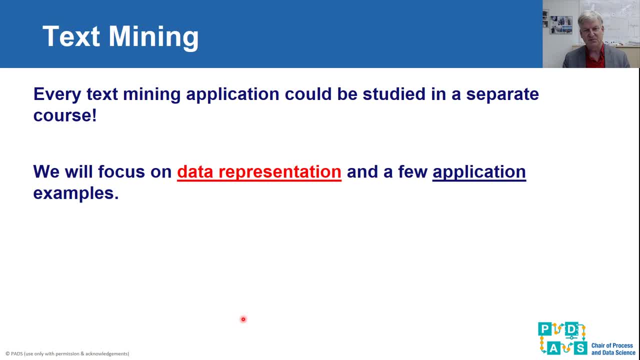 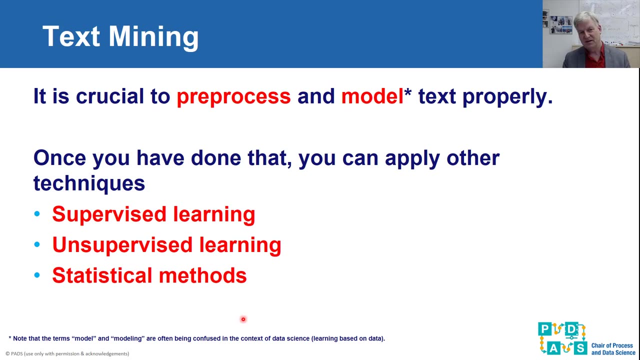 find these types of topics in a dedicated course on text mining. In this first lecture we will start with the basics, looking at mostly at the representation of data and the pre-processing of it. So we now start to slowly talk about the pre-processing of text in order to apply the various supervised 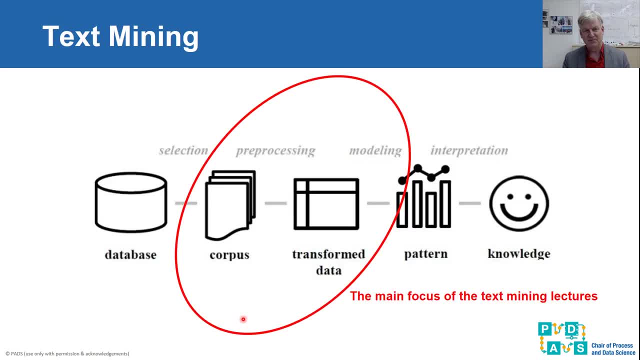 and unsupervised learning techniques that we had seen before. So the focus will be on this middle part And I will highlight it on this slide. Yeah, and the idea is- and I think you already get that after this first lecture- that once 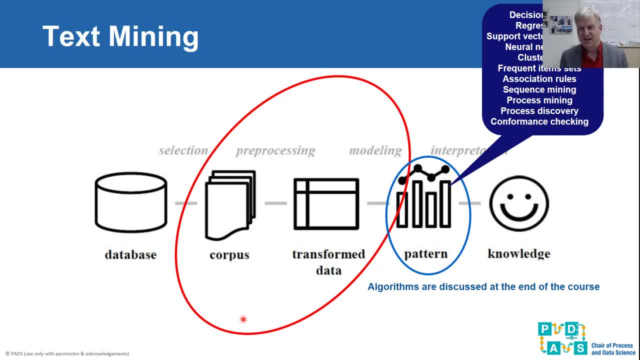 you have done that. you have representations And you can use these representations in conjunction with the techniques that we have seen before. So, for example, if we are able to translate every document to a feature vector, then I think all of you understand that once we have 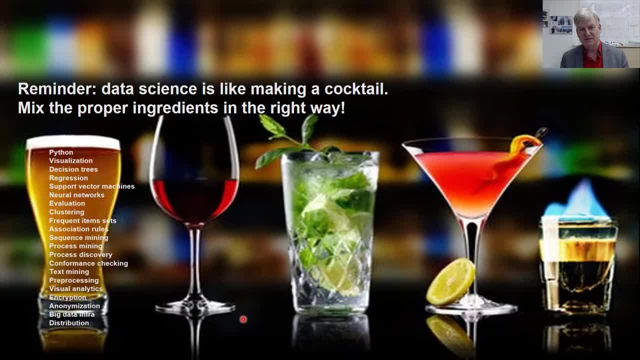 such a feature vector, we can do clustering And many other things, And I'm just going back to the slides that I showed already in previous lectures. We focus here on the pre-processing of text, And after having done that, we can use many of the things that we have seen before. 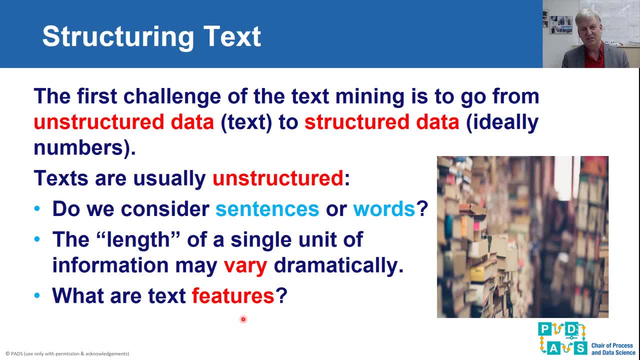 OK, let's start talking about text pre-processing, as I mentioned, And so text is, in principle, unstructured, And it's not that there should be a fixed number of words or words should be taken from a fixed small set of things. 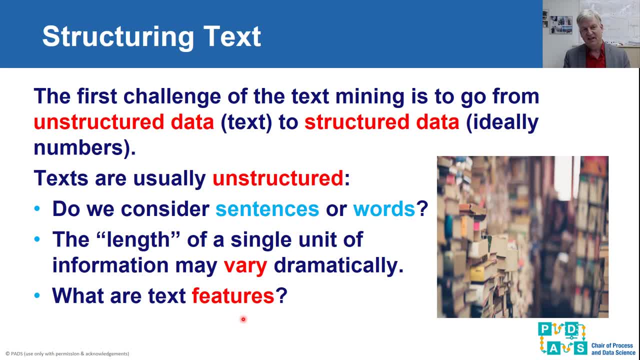 It's also unclear what the so it's unclear what the instances are And it is unclear what the features are. And for many of the, let's say, classical problems that we looked at, that was very clear And we had the columns corresponded to the different features. 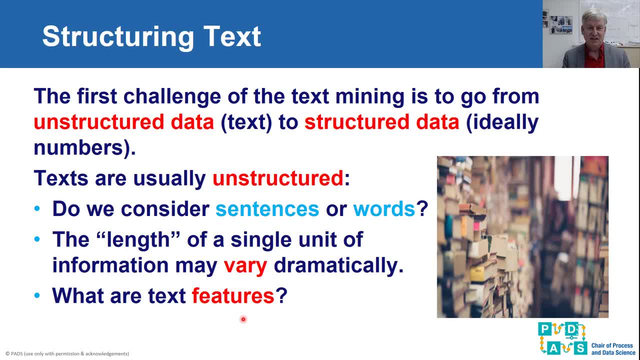 And the rows were corresponded to the features And the columns were corresponded to the different instances. If we are dealing with text, the question: what is this? So text is unstructured. What do we consider? We have words, we have letters, we have sentences. 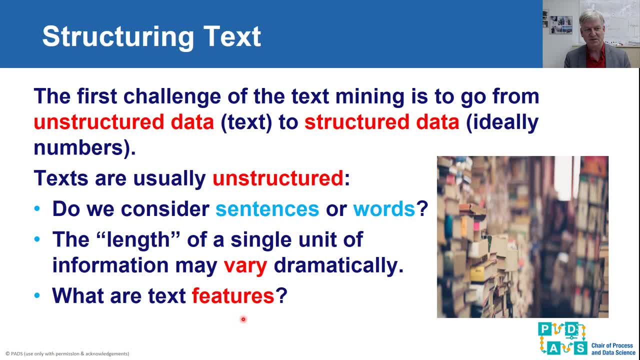 Sentences are in documents. Documents are in collections of documents. So what is the scope that we consider The length of a unit. The length of text may vary dramatically, So we may have articles of four pages, but we may also have articles of 100 pages. 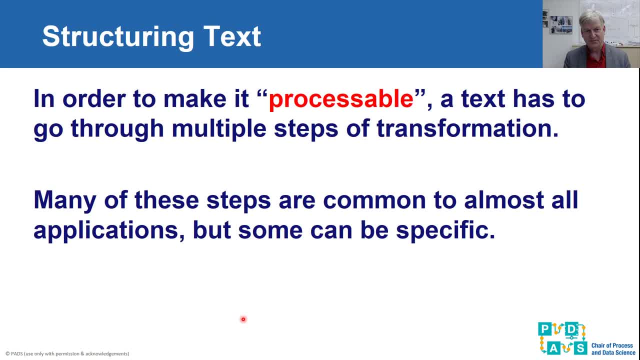 And it is not so clear what the text features are, And these are the things that we will answer in this lecture. So we need to pre-process the text, And I'm going to talk about the problems that you encounter when making the text ready to. 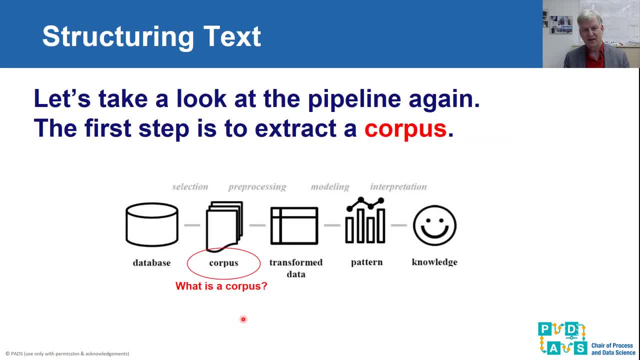 apply all of the features, All of these data science techniques. So the first question: I already mentioned that- What is the scope of the things that we do? So here I'm going to structure the problem a bit And you could still then interpret things in a different way. 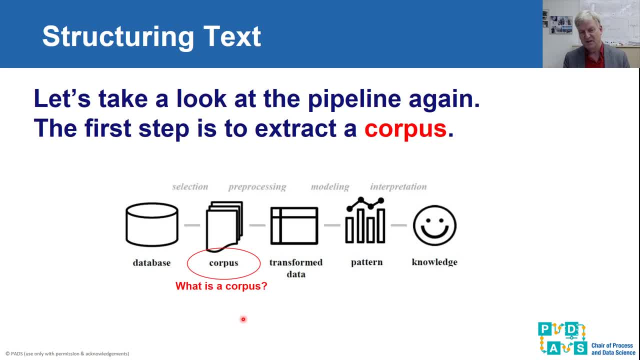 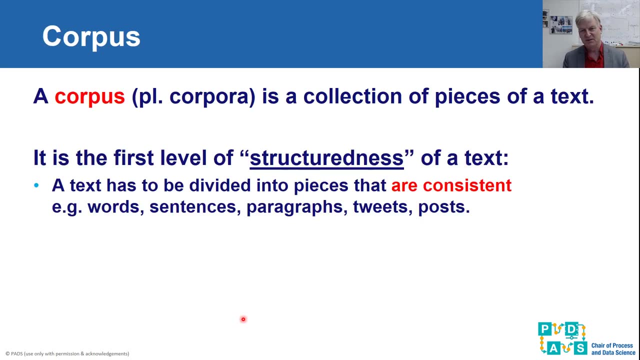 But the way that we view it is, we have a corpus that is composed of a set of documents, And we have a set of documents, And this set of documents is composed of words, And words are grouped into sentences. That's the basic structure that we will take. 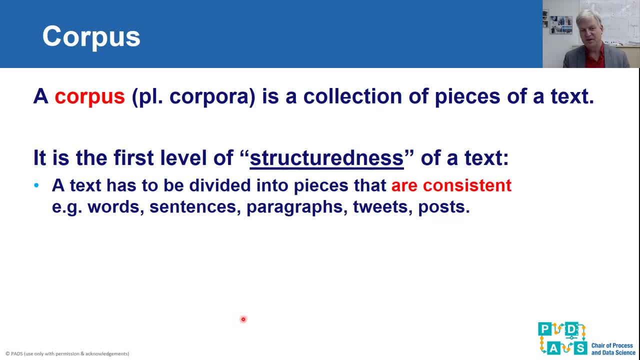 But in a way this is arbitrary. So if you look at Twitter data, then probably our corpus would be a collection of tweets And every tweet would be a document. So we have a corpus. That is the first level of structuredness. 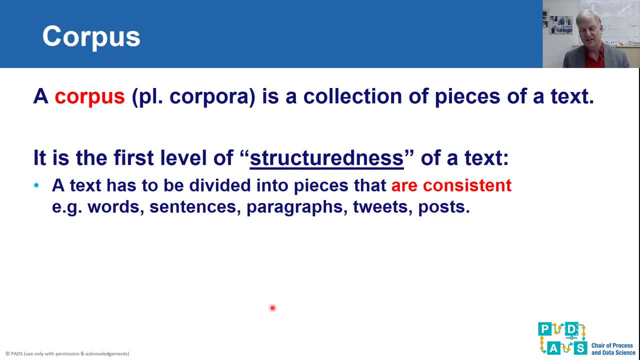 That we structure, That we somehow restrict our attention. Note that the world is, let's say, overloaded with text documents. So we always, when we do something with text, we always need to choose a particular scope if we want to do something. 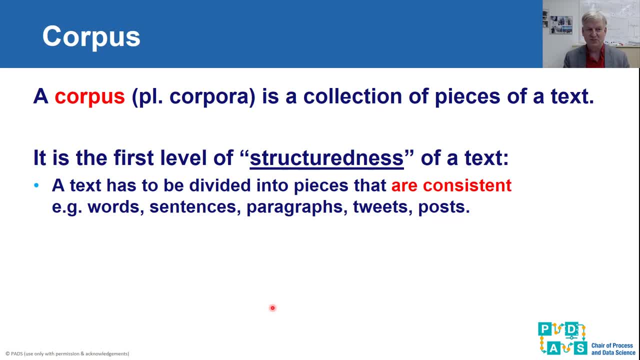 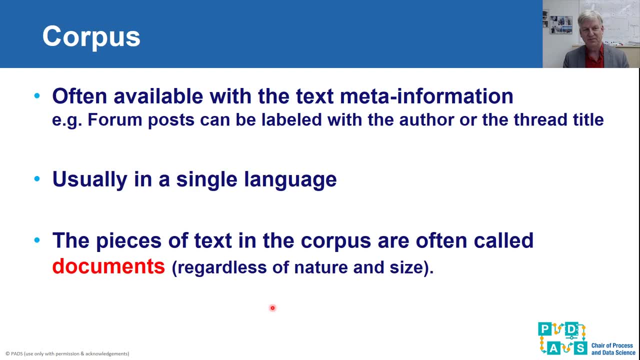 So we first need to scope it, And scoping leads to the identification of a corpus, And the corpus is further structured into documents. That's what is on this slide, And there may be metadata. Ideally, if we look at the corpus, it is in the same language. 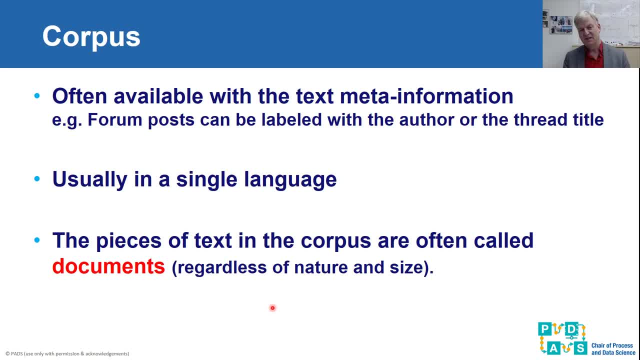 Because otherwise things are very, let's say, uncomparable. But this is a principle open. So we have a corpus, And a corpus is composed of documents. When I say the word document, you have an intuitive meaning with what it is. 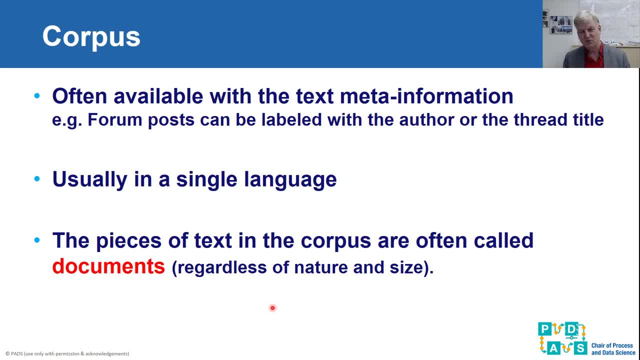 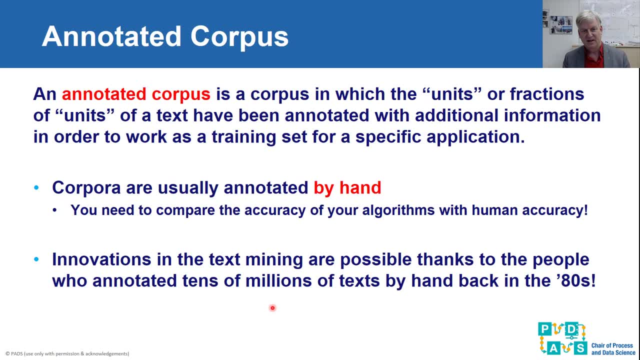 But it is a concept. It is a concept. It is a concept, But this could be, let's say, as short as a tweet, Or it could be an entire book. Such a corpus is then decomposed into documents, And these documents are consisting of, let's say, text. 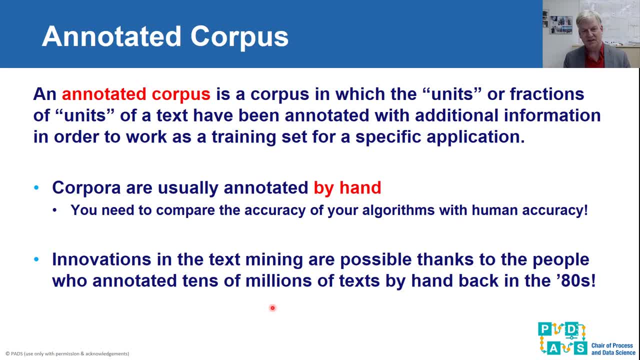 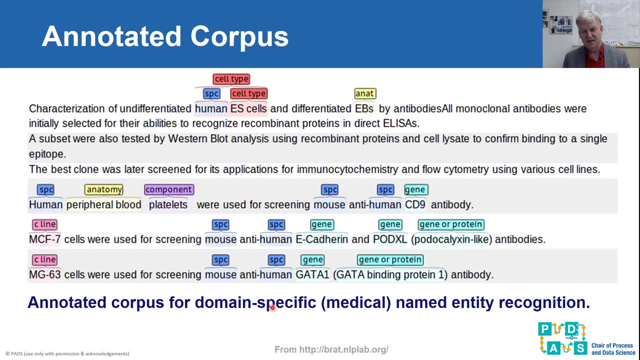 And typically these things have been annotated by hand, Both at the document level And also at the level of, let's say, the words inside such a document. So, for example, earlier I explained what named entity recognition is That when words or sub-sentences appear in a text that you say what they represent. 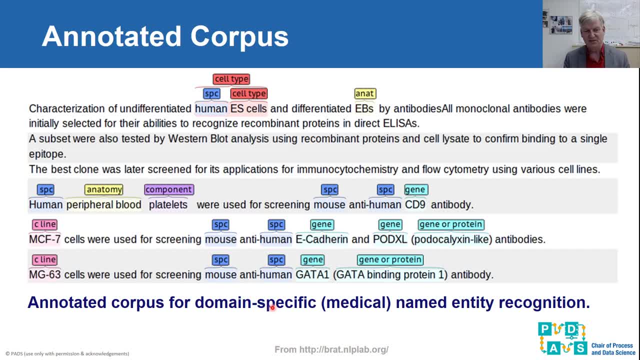 And here you see, for example, some example annotations. And here you see, for example, some example annotations. And here you see, for example, some example annotations. And these annotations are very important to do certain things with such documents. So lots of the text mining field heavily relies on humans annotating pieces of text. 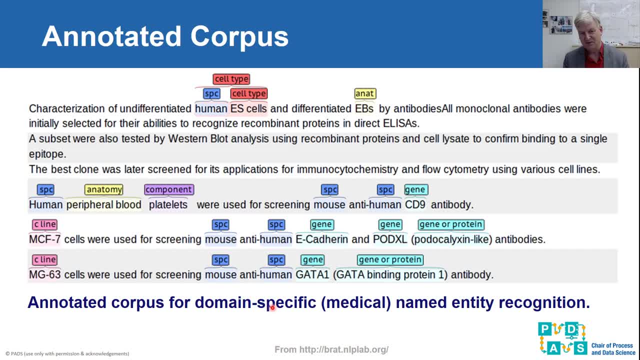 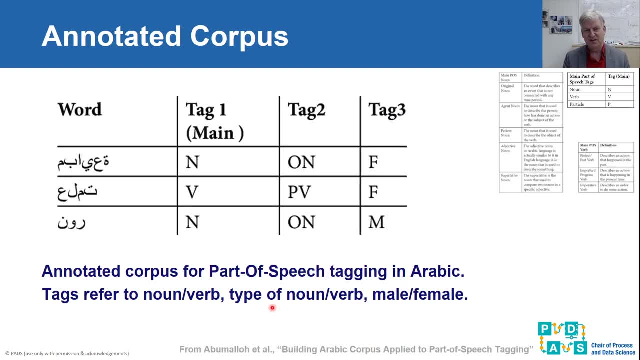 And ideally these efforts can be reused also for documents that have not been annotated yet, And so, for example, here you see an annotation at the word level. And so, for example, here you see an annotation at the word level. So here you see three words in Arabic. 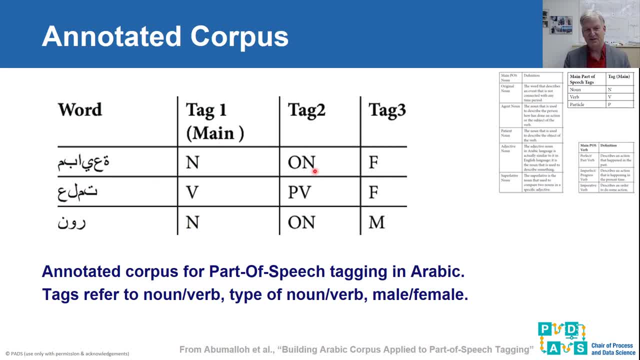 And then they are tagged with different properties, And so, for example, N stands for noun, v stands for verb, And so, for example, n stands for noun, v stands for verb. Then there are different types of nouns and there are different types of verbs. 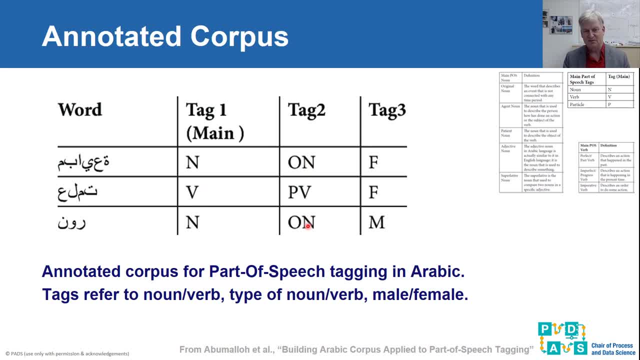 And words can be female or male. And so here we have words, We are tagging them with these properties, and if we have done that, then words would only be, you know, a preposition. we can reuse that later, independent in which document these words are being used. 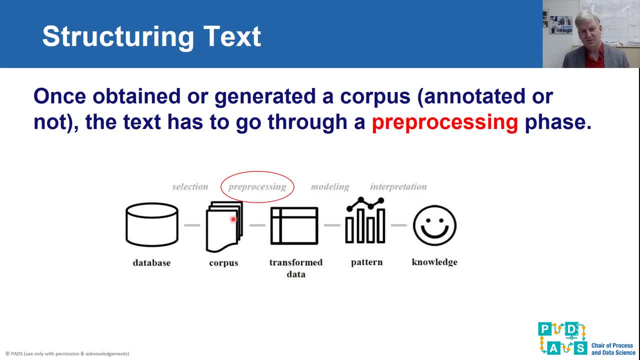 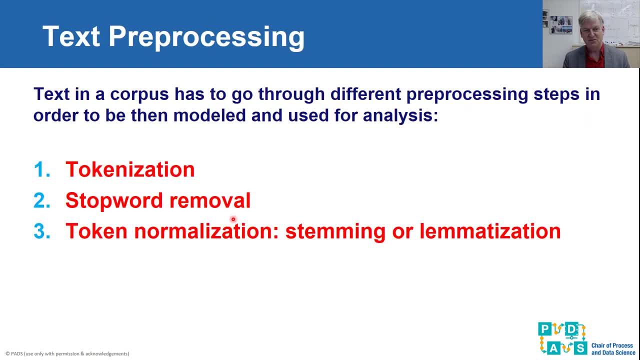 And so that is what we would like to do, And we need to pre-process that, because there are many issues, let's say, trying to do this. The pre-processing that I will explain will consist of, let's say, in first instance, 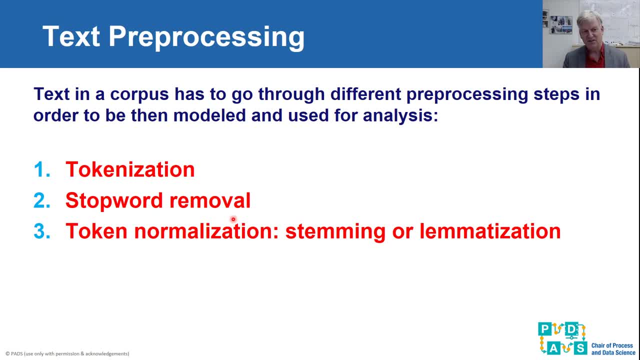 of three steps: tokenization, stop-word removal and token normalization. So tokenization means that we decide: okay, a document is composed of something, What are the units? let's say inside a document? Typically these will be words. 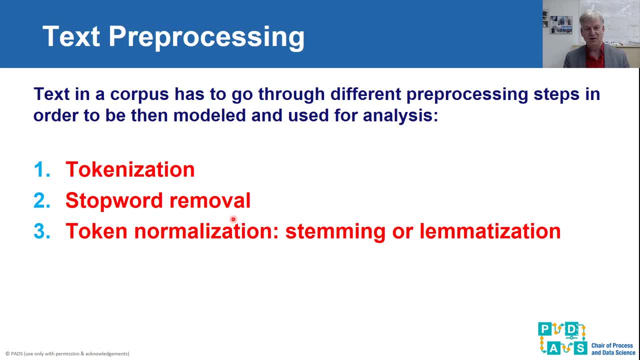 Then many of these tokens carry no information or carry only confusing information. We would like to remove them. that's stop-word removal. And there is the problem that there can be different words that actually refer to the same concept, And there let's say there are. later we will talk about more sophisticated techniques. 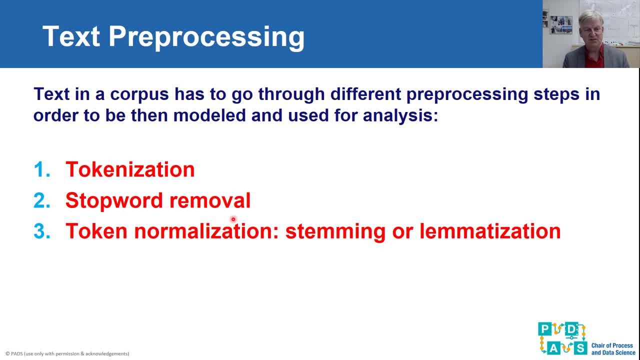 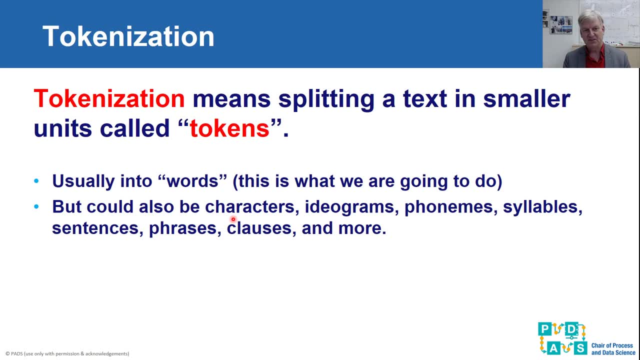 but initially we will look at stemming and lemmatization. Okay, tokenization, that is how we split a document. So, again, a corpus consists of documents and every document consists of tokens. Usually, as I said here, these tokens correspond to words, but that is not strictly necessary. 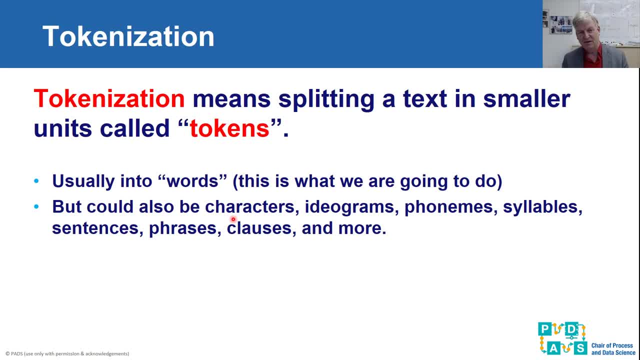 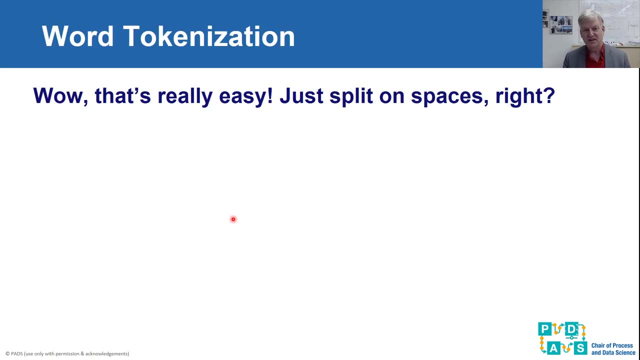 We could also look at lower-level structures like characters, But we identify tokens, so a document is now composed of a sequence of tokens, And that's the basic idea. So this is easy, you think at first sight. so when does the next word start? 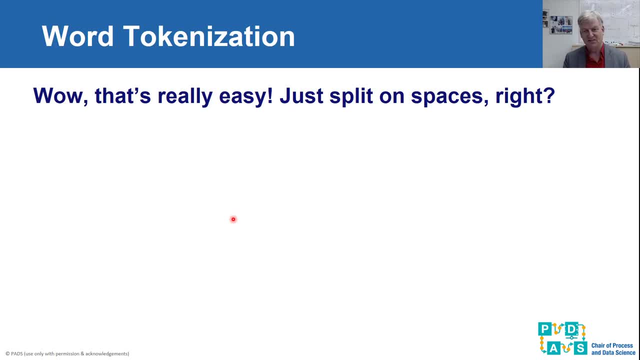 You could say: okay, that is when in a sentence there is a space, And if you do that, I could take a look at this sentence that we can all read. So this is a sentence, and now I'm going to identify what the token is, and I cut this sentence into tokens. 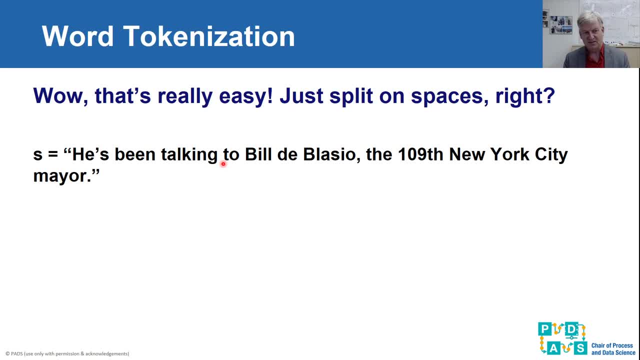 So in this example, a sentence is a document, as I explained it before. So we transform the document into tokens and basically at every space a new token starts. And if I do that, then you immediately see what the problem is. 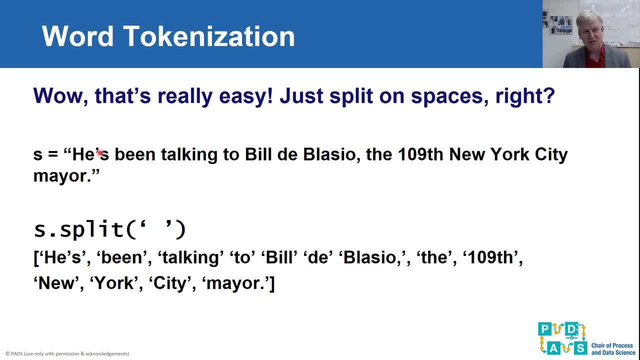 So I've applied some algorithm on this that breaks the document, So you can write such a function yourself in, let's say, five minutes, and then it will return this. But the question is: are we now happy? If you look, at first sight it looks reasonable, but then if you look deeper, it is not. 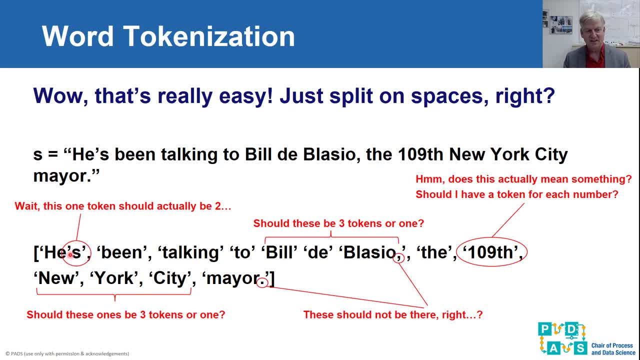 So there is no space here, but we all know that this actually means he is. So this should be two tokens, Using the philosophy that we also used in the rest. Then there is this name consisting of three words. The same holds for, let's say, New York City. 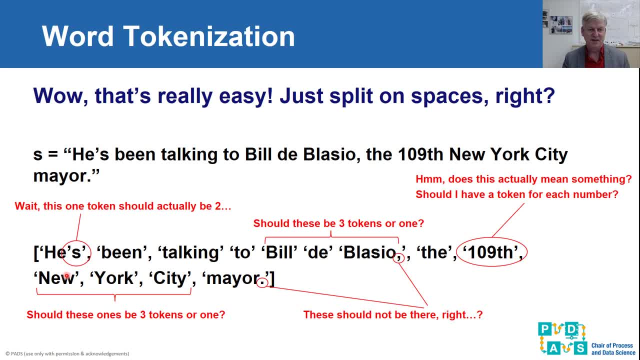 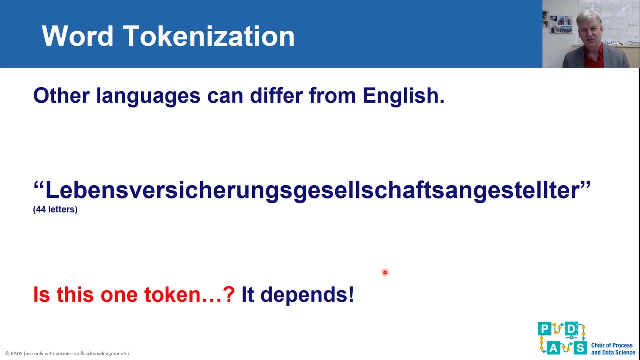 They refer to the same concept, either a name or a city. There are these punctuations that are not separated by spaces. So you already see that if we break a document down into tokens, that things get tricky Depending on the language. in some languages, like if you compose words, 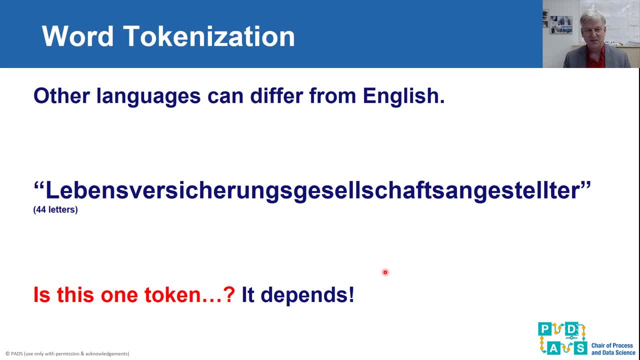 they still exist as, let's say, individual words. If you look at the German language, that is not the case. So you can kind of make these very long words that refer in a way to different nouns. So you can kind of make these very long words that refer in a way to different nouns. 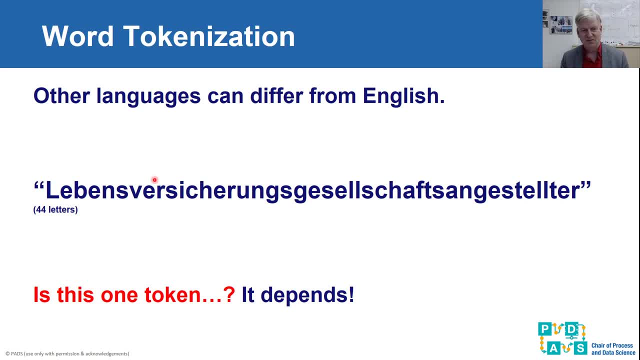 So you can kind of make these very long words that refer in a way to different nouns. So for example, here the first one is Lebensversicherung, So Versicherung is already insurance. This means life insurance, etc. etc. 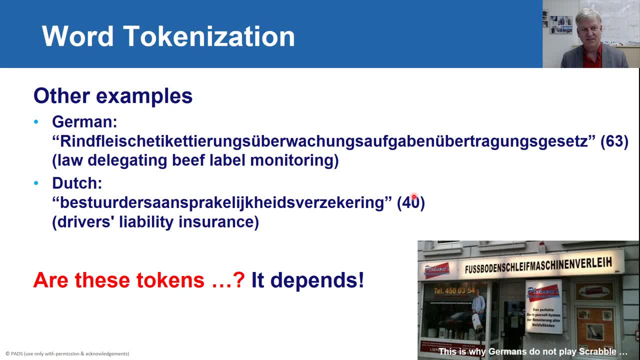 So it becomes very complicated. There are other examples. This is just funny to see that. You also see a picture here. For example, here we have a word of 63 characters. You also see a picture here. So, for example, here we have a word of 63 characters. 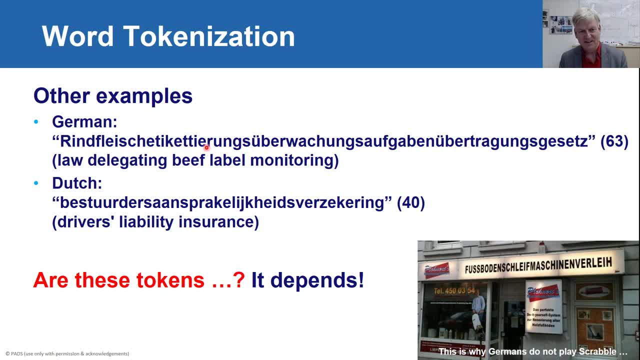 So for example here we have a word of 63 characters. So for example here we have a word of 63 characters. So Rindvleischetiketterungsüberwachungsaufgabenübertragungsgesetz. 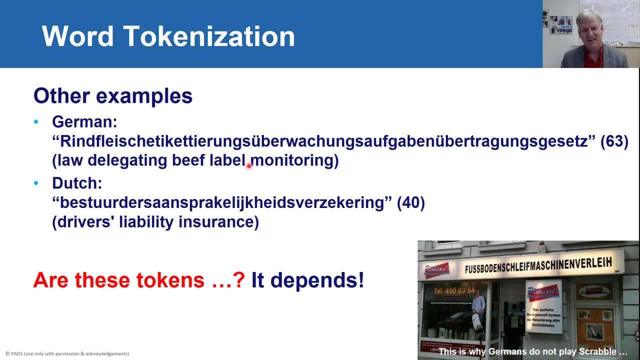 So that's a mouthful And there are, let's say, many. if you would go to English, this would be many separate words In Dutch. that's a bit easier for me. This is a very common word: Bestuurders-aansprakelijkheidsverzekering. 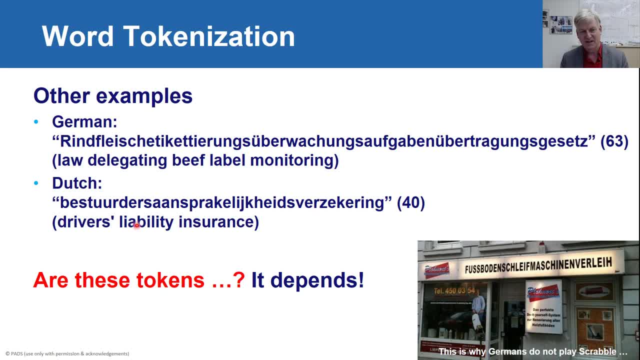 So that is driver's liability insurance. And so if we now have a sentence that contains words like this, what are now the tokens? So, for example, this Dutch word of 40 characters: is that now one token, or should we split it into three tokens? 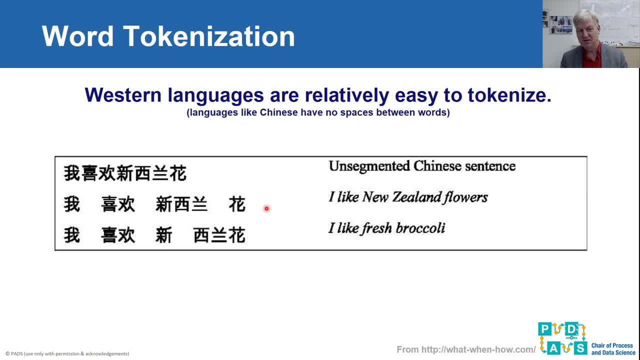 It all depends on the application that you have in mind And, depending on what you want to do, you need to make different design decisions. There are also, As we just compared, English and German, or English and Dutch, there are differences, But also if you go to, let's say, completely different languages like Chinese, 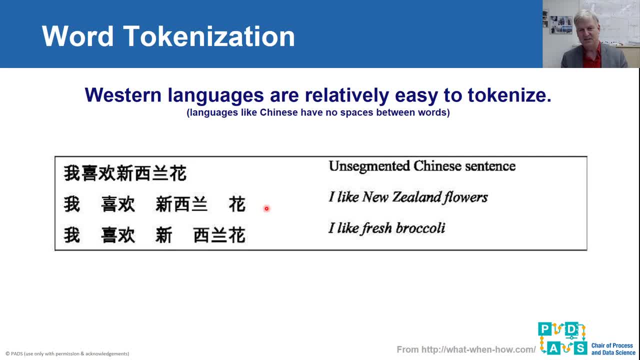 there are subtle differences that do not matter in one language but are very important in another language. So this is: if we look at these Chinese characters here, then depending on where we put the spell, the meaning changes completely, And so how we tokenize these things is somehow very important. 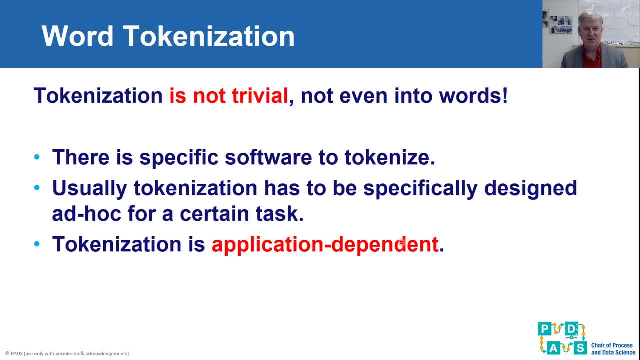 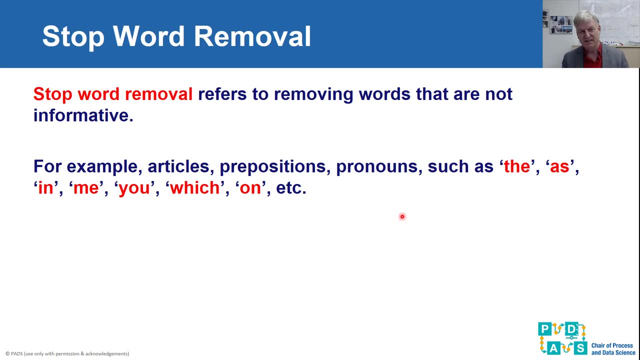 So this is showing that tokenization is not trivial and it highly depends on what you want to do and it also depends on the language in which the document is written. So that's the first step. We have identification, We have identified the tokens. 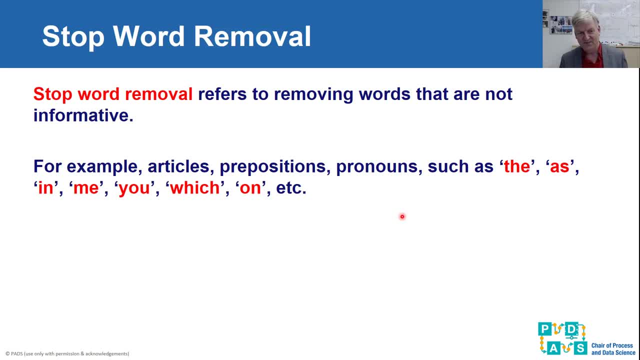 Let's just assume that that worked all well and that we somehow managed to use rules to break it up in tokens. Then the second step is that we would like to remove the tokens that do not have, that are not so meaningful and will only, let's say, hide the actual meaning of a document. 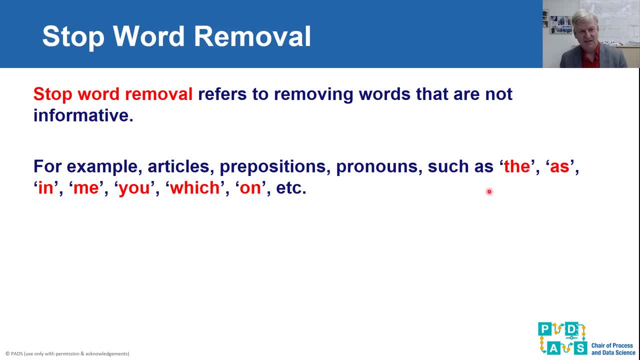 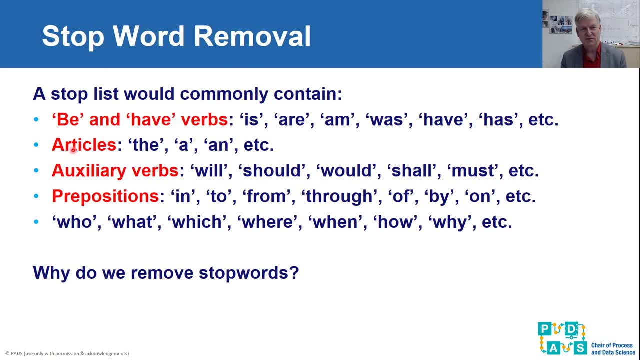 So these are words like, as in me, you, which on, etc. So what you do if you do a stop word removal? you make a list of tokens that you would like to remove, And here you see an example list. 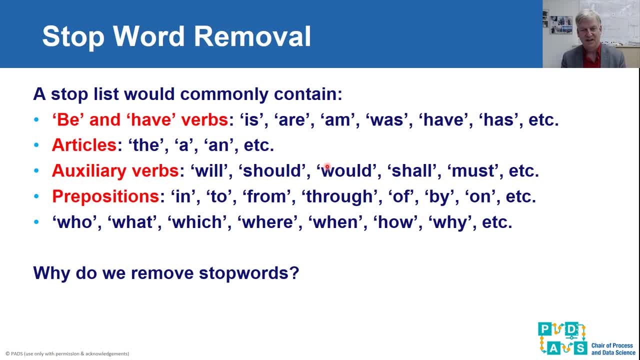 and again, this is highly application dependent what these lists are, And so in the remainder of this lecture, I will assume that this is my list, that I'm removing the types of words that we have here, So you may wonder. 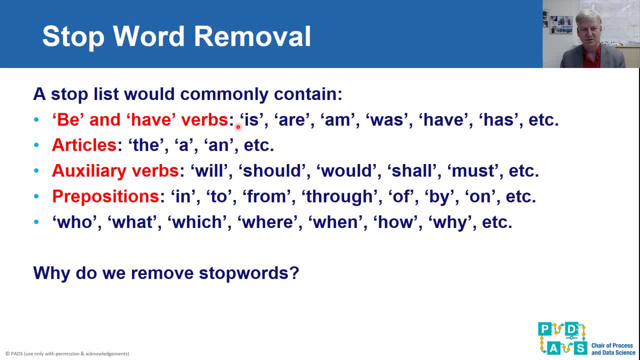 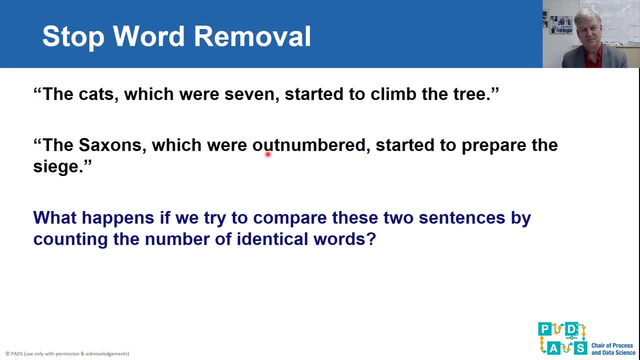 okay. yeah, this looks very dangerous. If we remove all these words, do we still capture meaning? Is this strictly necessary? Yeah, you need to remove stop words and I think these two sentences show that very nicely. So these cats- I think everybody agreed that they mean. 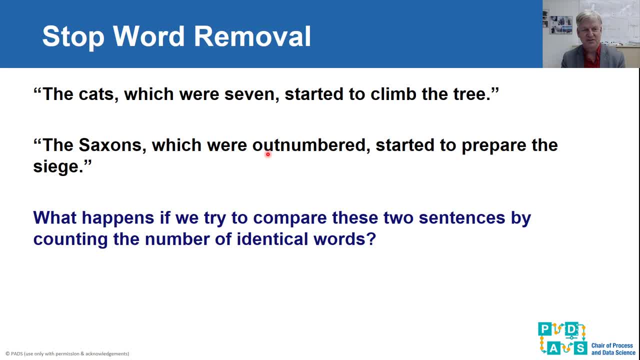 two completely different things. They are unrelated. Yeah, So if we now try to compare these two sentences by counting the number of identical words- and we did not do any. stop word removal- then I can highlight the words that appear in both sentences. 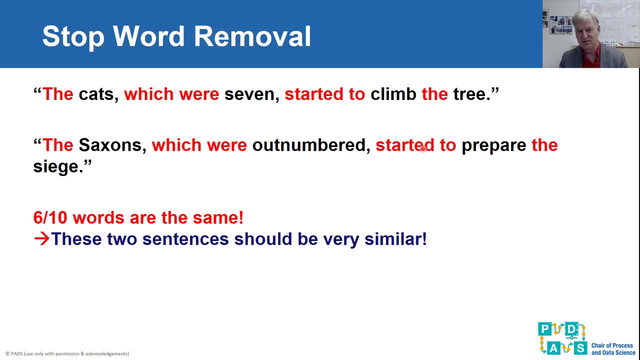 So two times two, which were started, two is appearing in both sentences, etc. So if we look at the, both sentences have ten words and six of these two ten words are the same. So only four words are different. 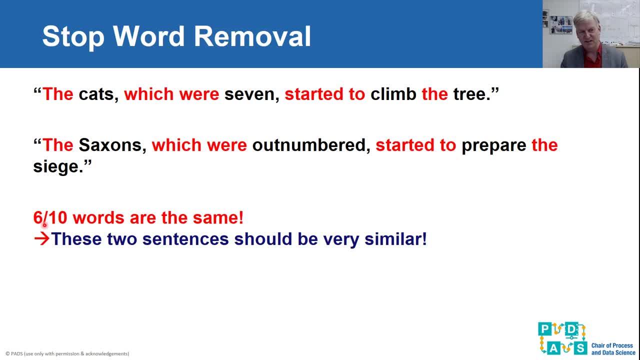 And so if you think about two sentences that have like a 60% overlap in words, you're tempted to think, okay, these two sentences are very close to each other. If you look at the sentences, you know that that is not true. 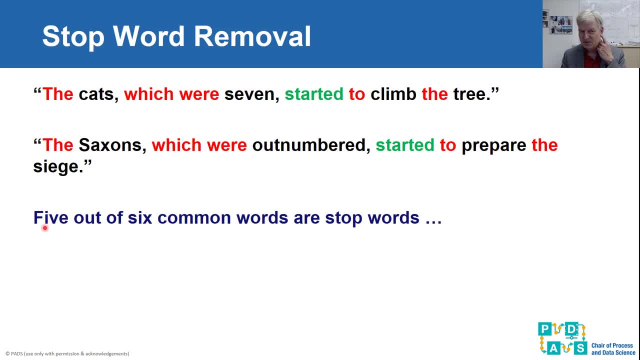 So if I know, look at of these words what are now stop words, then all our stop words, according to our list, except the ones which started, And so there was a huge overlap, And so six out of ten words were identical. 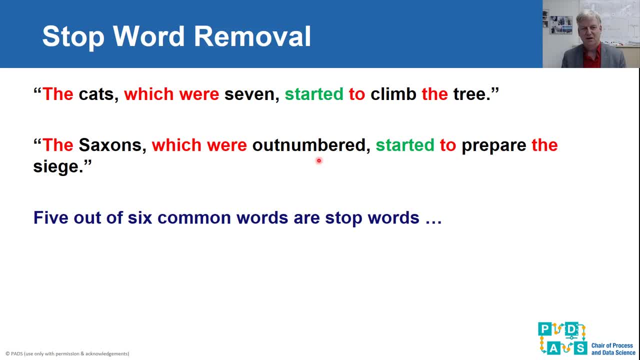 Sixty percent was exactly the same. But if we ignore the stop words, only one of these ten words was actually the same, And so then you would say the overlap is very small. So we are going from 60% overlap to 20% overlap. 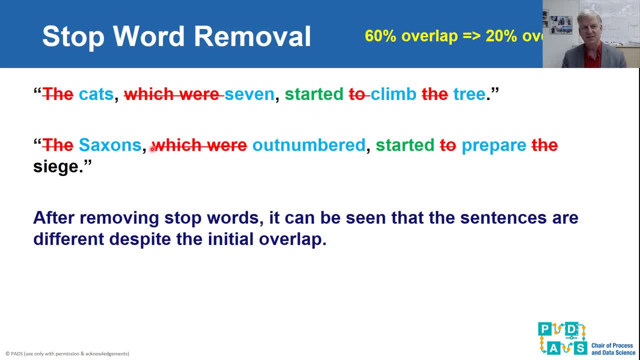 if we remove the stop words, And that is illustrated here. And so now we should compare, we should focus on the green and light blue after removing the red words, And now you can see that the similarity is actually closer to what our intuition. 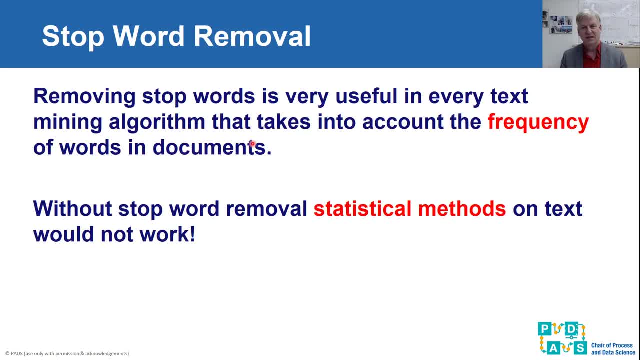 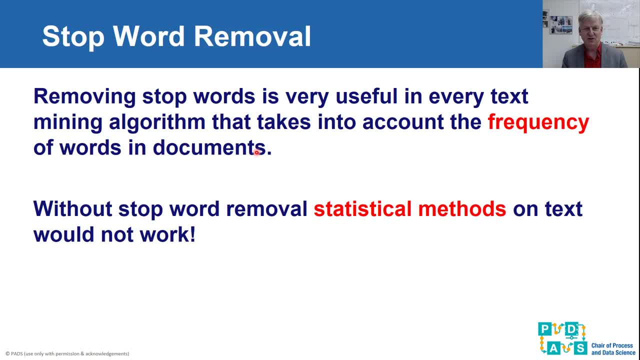 if you have mining algorithms that have a vector and you look how often does a word appear And it is counting the number of times that D appears, and that would have a heavy factor on how we deal with that document, You can imagine that this doesn't work very well. 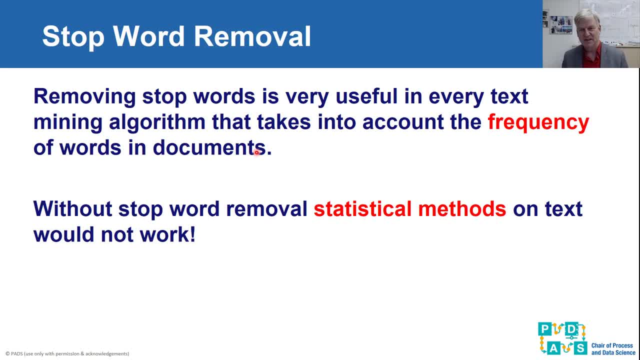 So, Because algorithms will take into account the frequency, we should somehow get rid of these words that have no meaning, and we will later see also how to do that kind of automatically. But, as I said, we kind of look at the stop word list that I indicated before. 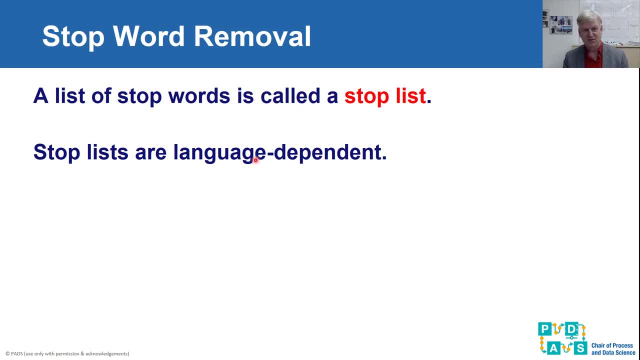 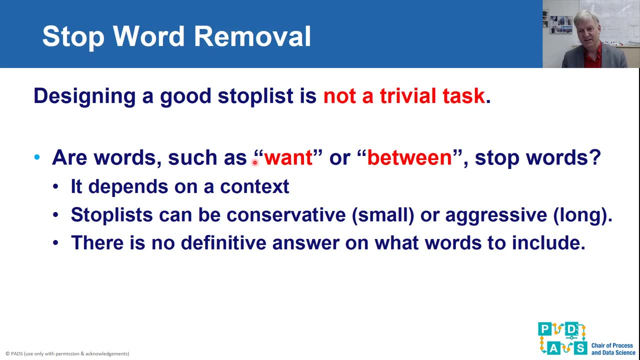 So we have a stop list and, of course, these lists are language dependent Also. this is again heavily application and language dependent. depends on the context and also, for example, we will talk about how to cut words to their base meaning We can have conservative approaches and aggressive approaches. 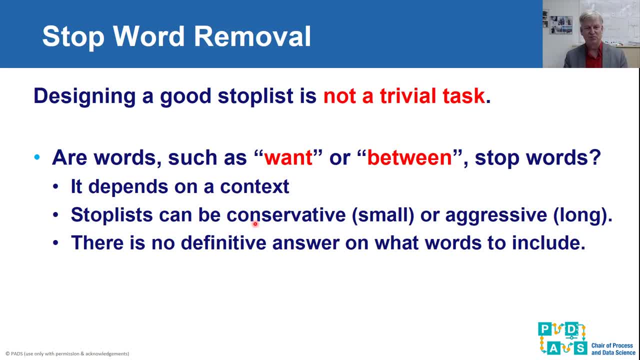 So conservative approaches: just remove a smaller percentage of stop words. aggressive techniques: try to remove many words And please, when I talk about text mining and NLP, do not expect very precise recommendations or very precise techniques. It very much depends on the application. 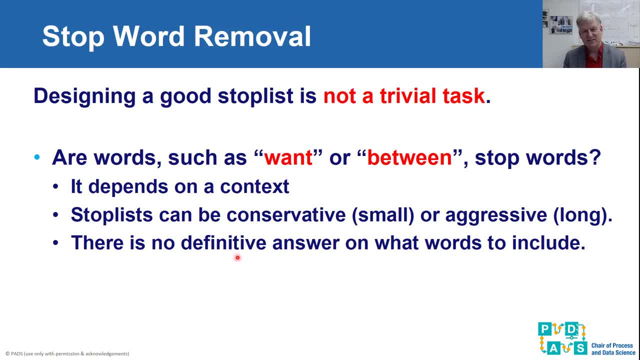 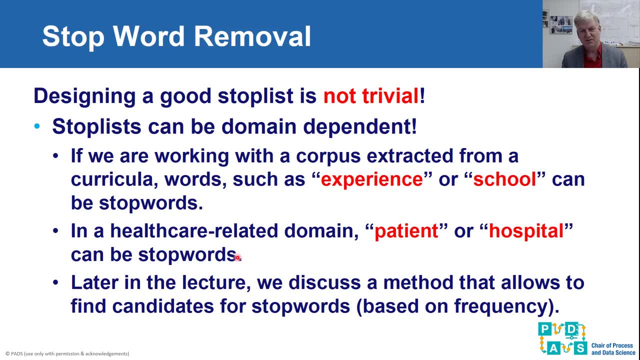 and one cannot give an objective answer to all of the questions that I'm raising here. So this lecture, This lecture is more about making you aware of the problems and that you see, let's say what are the design choices that one should make. 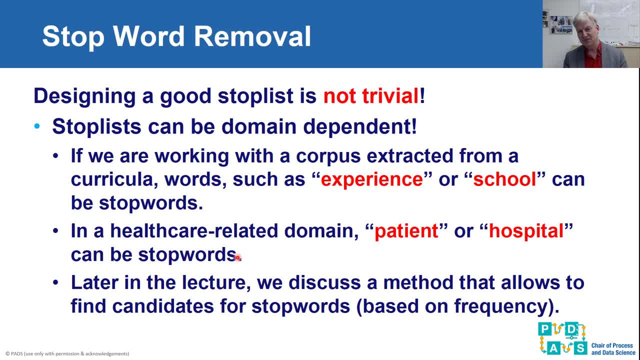 This is illustrating that stop words can be, let's say, context dependent. So, for example, working with the corpus extracted from curricula, words such as experience and school do not say anything, because they will appear in any of the documents. 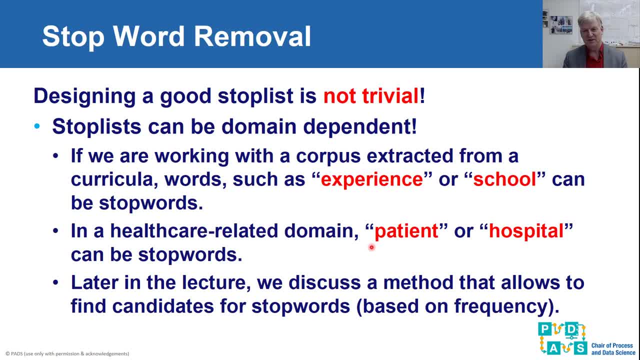 Similarly, if you would look at, let's say, a healthcare-related domain, it could be that words like patient and hospital can be removed because they don't mean anything. At the end of this lecture, we will look at, let's say, identifying candidates for stop words based on the frequency of words. 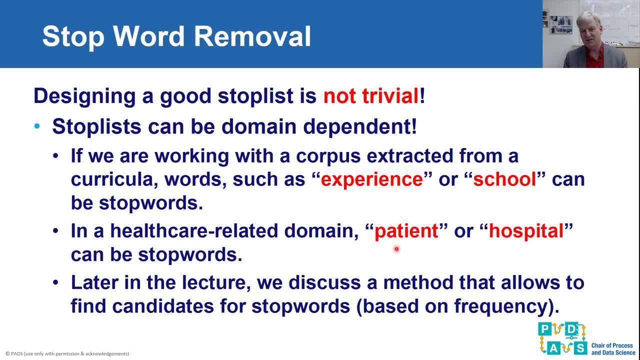 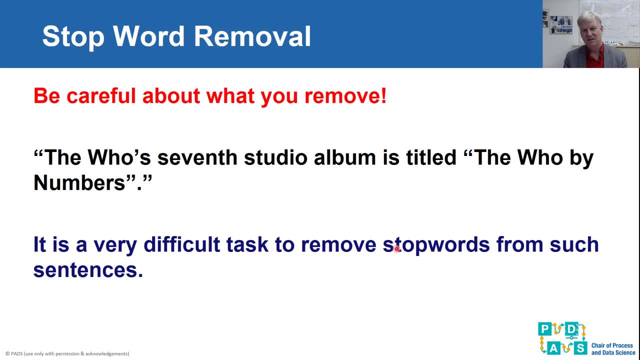 So if you have words that appear in any document, then they are not that distinctive, So we don't need to use them. We don't need to use them for things like love-string. At the same time, one needs to be very careful. 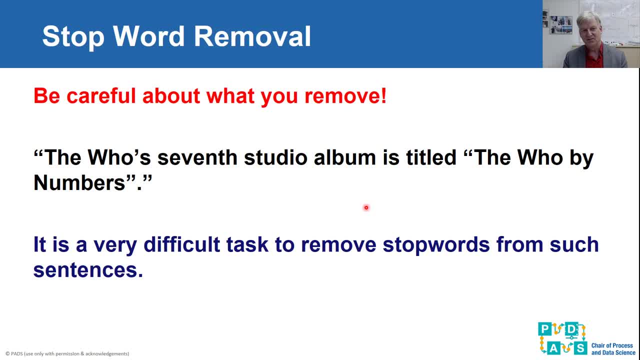 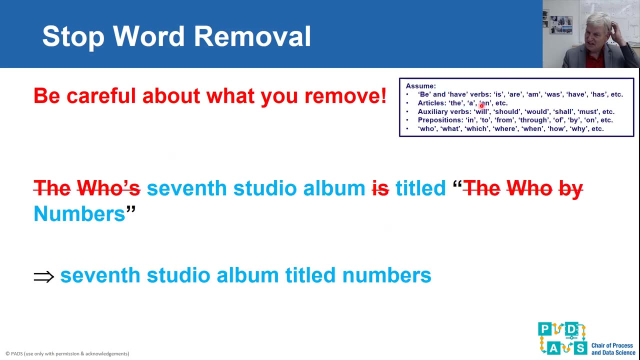 because sometimes in a sentence things syntactically look like a stop word, but semantically they are not, And so this is a sentence that has a certain meaning, If we now do stop word removal and we use the list that I highlighted before. 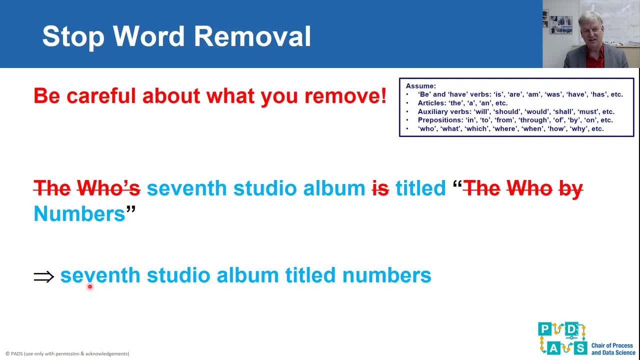 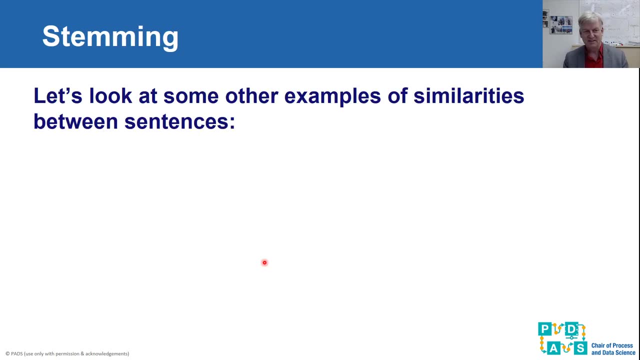 then we remove. we remove all the things highlighted in red and only the blue part remains, And somehow, by removing the stop words, we lost, let's say, what the actual sentence was about. So all of these things are, let's say, very tricky. 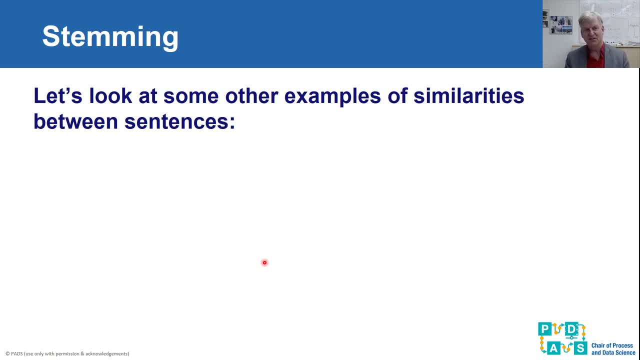 They require engineering, they require knowledge of the application domain, and there is no exact, precise answer to any of these questions. So we have all these words. Then we have the next problem: that there may be variations of the same word. So if you look at these sentences, 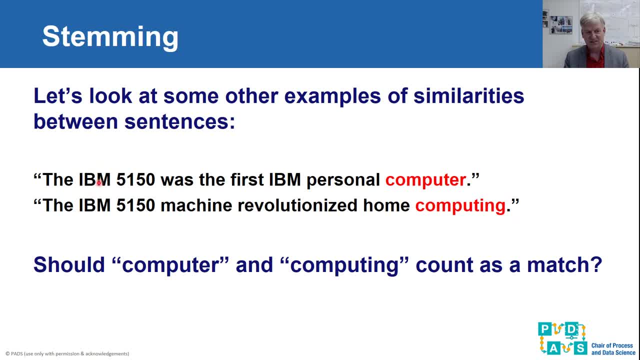 then it's clear that things that are, let's say, syntactically the same, you can say that there is a match. But how do, let's say, computer and computing relate to each other? Are they different or not? So if we now build a vector, 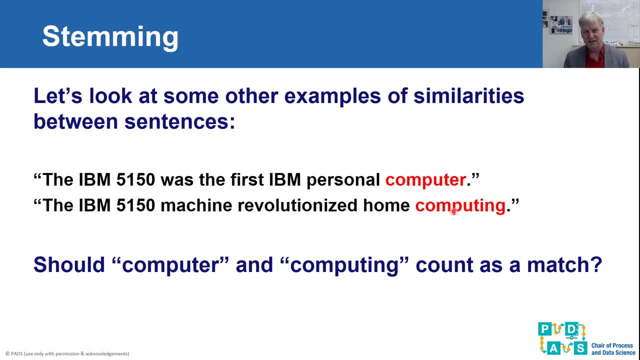 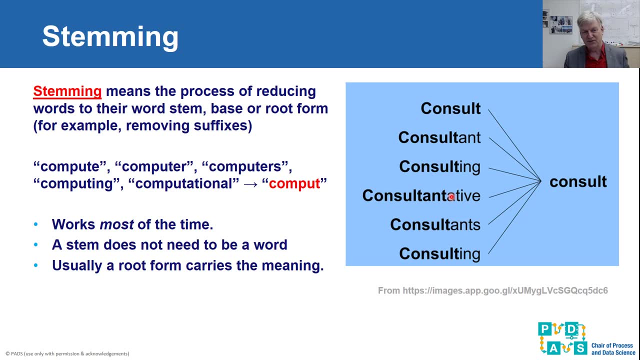 and we count how often a certain word is appearing in a sentence after removing stop words. do we count computer and computing as the same thing or as different things? The topic of stemming tries to address this problem by basically chopping off part of the word. 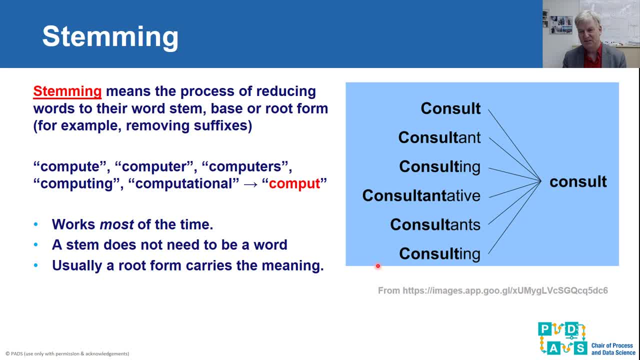 So what you see here is that, if you have these different words, there are, let's say, a limited number of relatively simple rules deciding on what to cut off a word. So this, as is indicated here, this works most of the time. 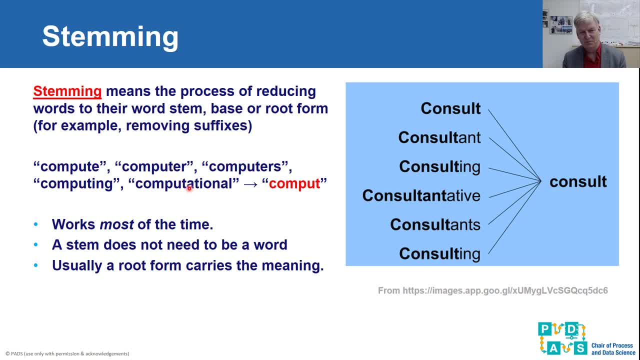 So, for example, compute, computer, computers, computing, computational using stemming could also all be reduced to compute, And then all of these things would be mapped onto the same, let's say, feature. This works most of the time. 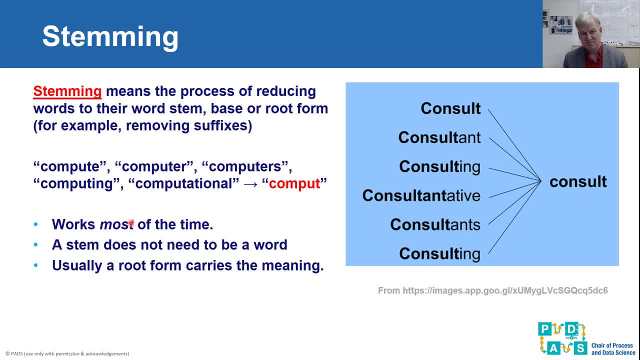 What you see is that a stem, so what remains after stemming is called a stem. It does not need to be an official word, as you can see here, And the idea is that the root of the word, so this stem, captures the meaning of the word. 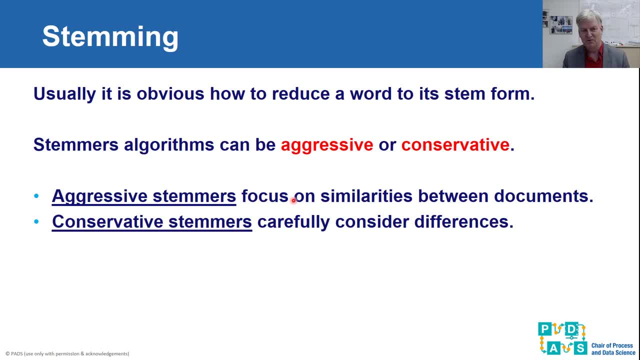 These techniques can be just like stop-word removal. They can be aggressive in the sense that they want to chop off, let's say, lots of words, Or they can be conservative and that they do not want to, let's say, map two different words onto the same word. 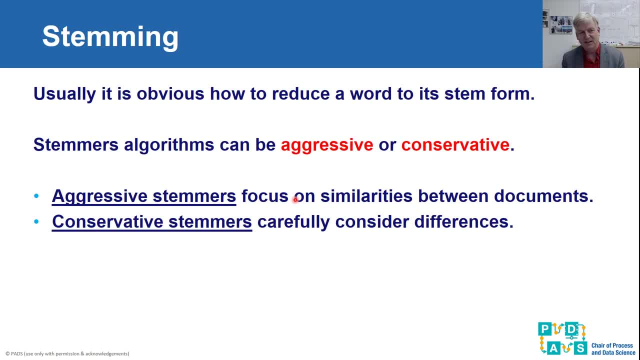 although they have nothing in common. This is very similar to stop-word removal: You can be aggressive or you can be conservative, And so these aggressive stemmers, they want to find, let's say, similarities between documents. Conservative stemmers are afraid to kind of lose subtle differences between documents. 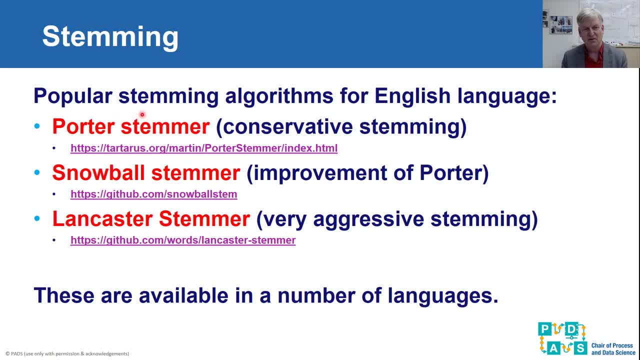 When you go online and you look for software and you look for papers, you will find, let's say, various stemming algorithms that automatically, automatically do this, And here I've listed three, And so Parter developed one of the first techniques. 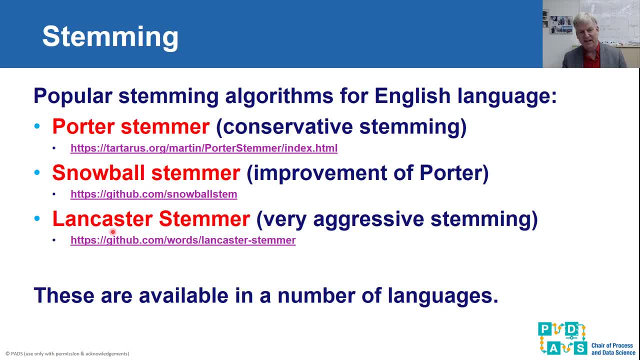 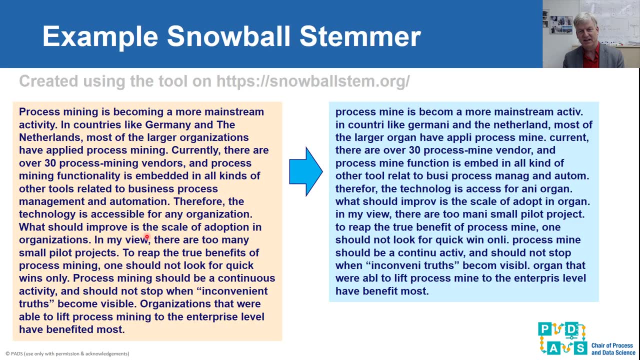 that led into the Snowball stemmer. The Lancaster stemmer is something that is being more aggressive, And so more words map onto the same stem. These are available in various languages, And so if you go to this website, I can take a piece of text that I wrote. 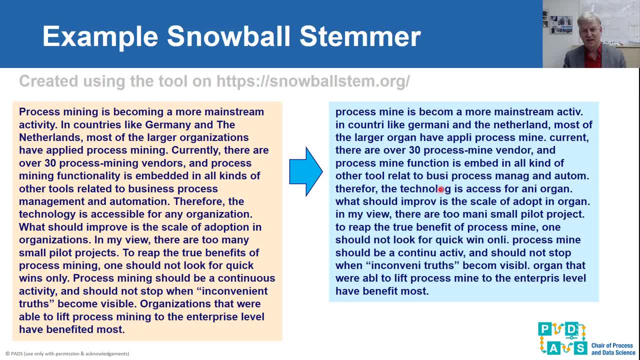 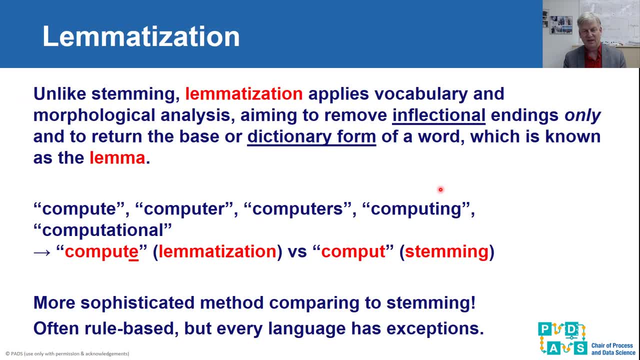 and I can map this piece of text onto, let's say, the text that remains after stemming. So stemming is basically chopping off the last part of the word, But the word that remains does not need to be an official word. Let me show you an example. 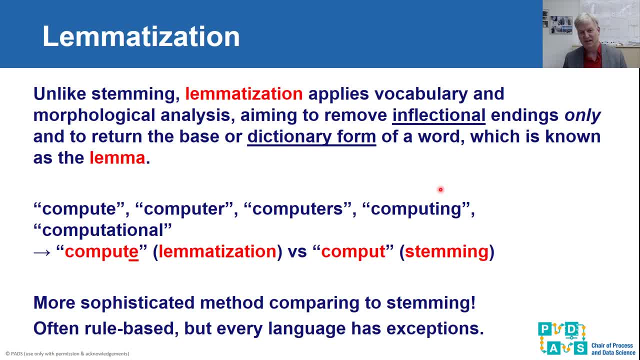 Lemmatization works different. You can kind of look at it that you would take a dictionary and that you try to reduce it to the, let's say, core dictionary form where you would look it up. So, for example, if I take the verb work, 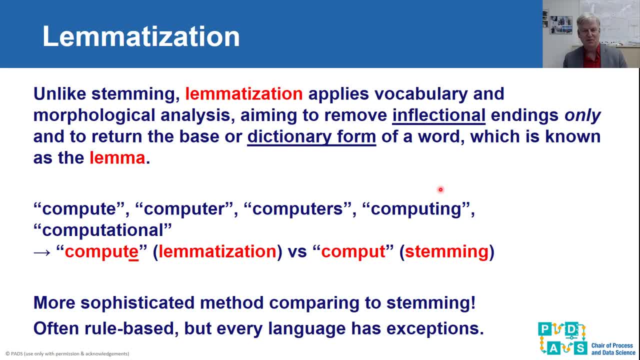 there's work, walking, walked, etc. etc. And you try to. So all of these things correspond actually to the same verb. So when you do something like that- of course you can also do that with nouns, similar things And the base form- you call that a lemma. 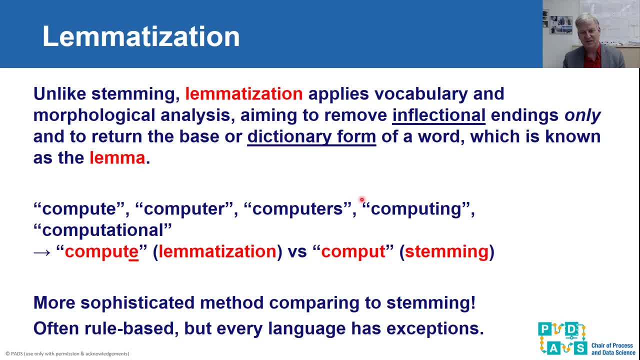 So if we take the examples that we had before, so using stemming, we were chopping off the last part and we ended up with this non-existing word. If we look at this, then it would be mapped onto compute. So this is more sophisticated than stemming. Lemmatization tries to identify the base forms of all of these words. 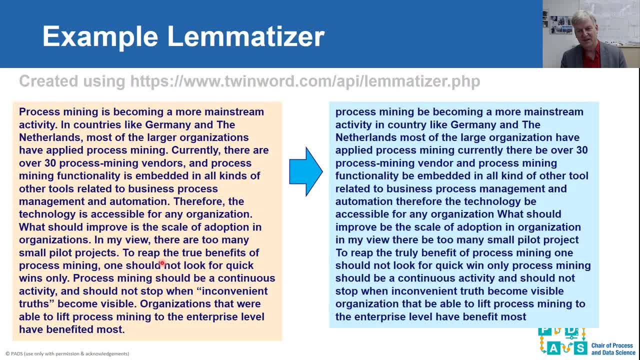 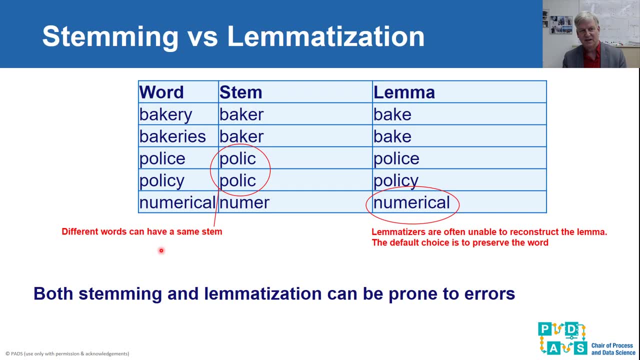 And also there there are various, let's say, techniques to do that. This is more refined And here you can look at a piece of text, the same piece of text that I took, and I look at the mapping. So here you see some examples. I will also show the text that I just showed to also compare the difference between stemming and lemmatization. So here you see some examples. I will also show the text that I just showed to also compare the difference between stemming and lemmatization. So here you see some examples. I will also show the text that I just showed to also compare the difference between stemming and lemmatization. 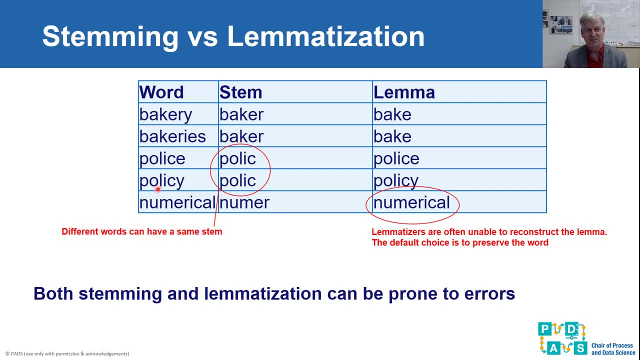 So here you can see that if we chop off the last part and police and policy become the same thing with stemming, That is of course nonsense, because they refer to two completely different concepts. Lemmatization is, of course, limited by the ability to map things onto common things. 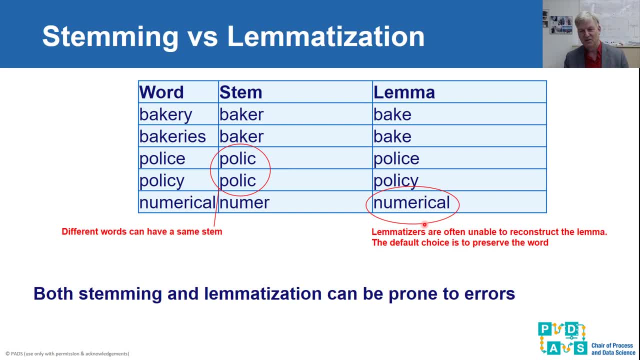 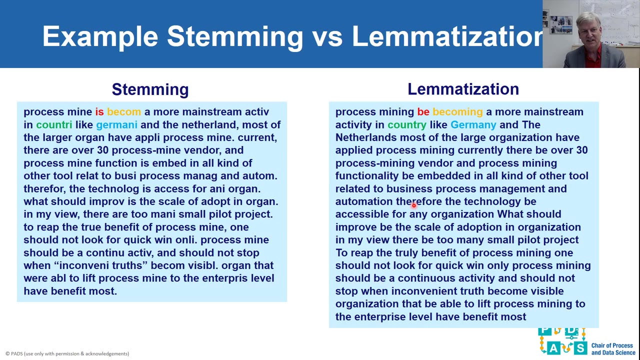 And it all depends whether there is the ability to map things onto common things. there is the ability to do so, so that is typically less aggressive, but that means that it may be impossible to to map things that are actually the same onto the same lemma. so this shows the text that I showed earlier. so you, for example, 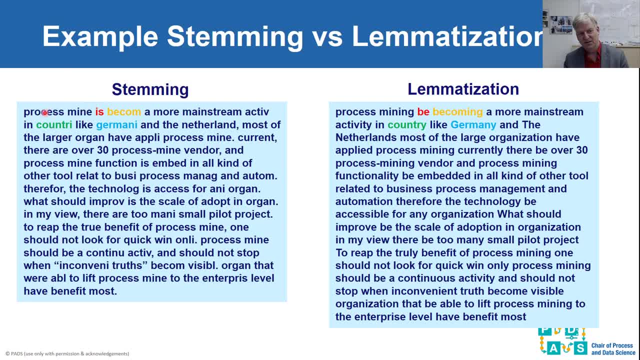 see that in the original sentence it was process mining is becoming, and then you see here is become, and here you see be becoming. so this is the lemma: is: be is just remain, because nothing could be chopped off. become is of course, not like, like a word, so basically the last part was chopped. 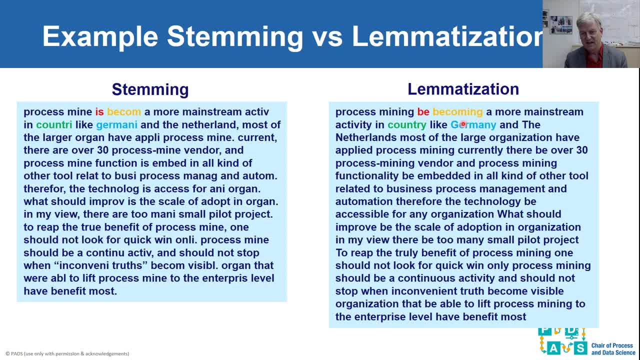 off here. this is still a verb country, and see it here on this side. you can see that, that it is translated in this way here, etc. etc. as I think that the differences are clear, the question is: can you know still read these sentences after applying either stemming or lemmatization? 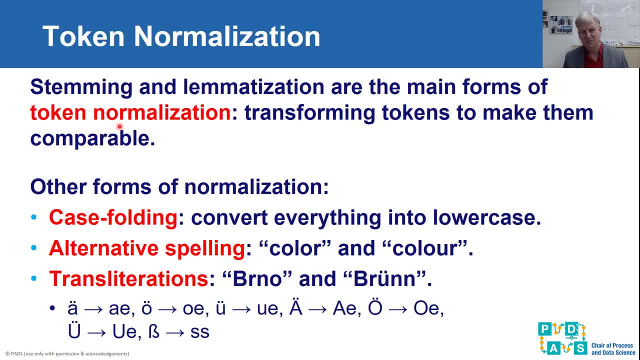 what we see is that, although these texts may become incomprehensible, if we later feed it to things like neural networks, they are able to do surprising things with these pre-processing texts. So stemming and lemmatization can be seen as normalization techniques You want to have. 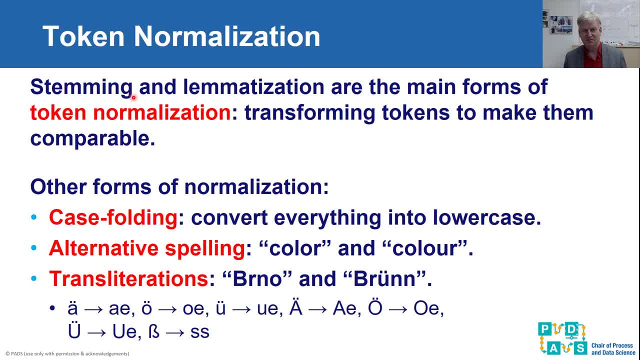 tokens that are syntactically different. If they are semantically the same, you would map them onto the same thing. Of course this applies to removing punctuation types of things. It also makes sense to convert everything to lowercase. that doesn't make a difference. 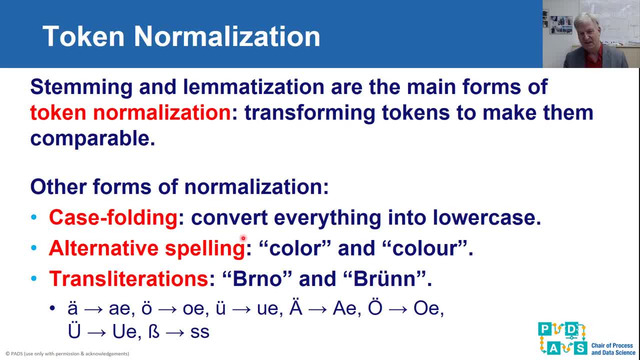 anymore. You may have British and American spelling, like color with O and G Or modeling with either one L or two L's. There may also be these words of cities that sometimes are translated to the language, sometimes not, And of course you have this. 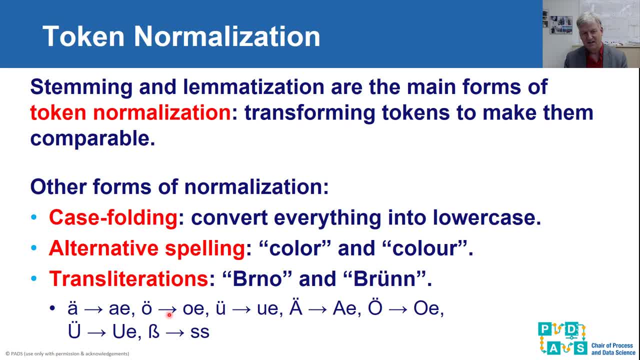 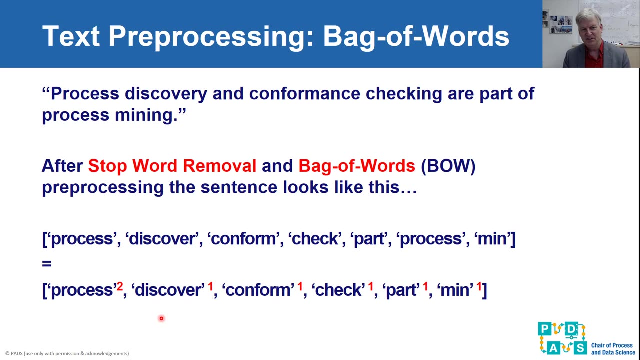 translation of certain characters, So Oumlaut can be converted to that And sometimes when people are using an editor or a device where they cannot type Oumlaut, they will write OA, but they actually mean exactly the same thing. So these are things that we can do and I think that is pretty clear. 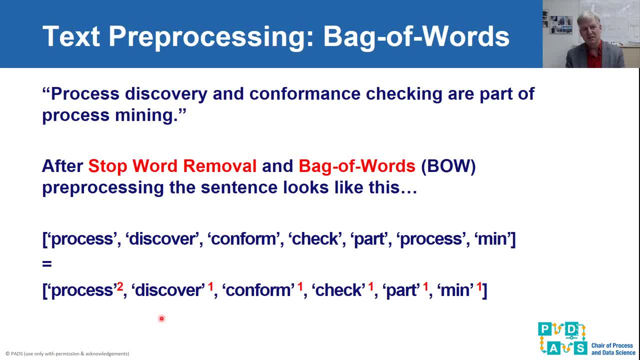 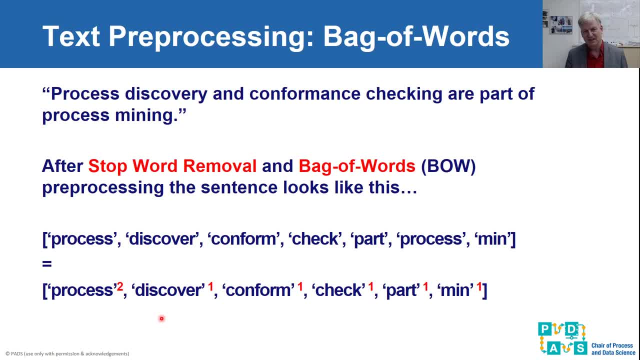 So we have sentences in documents and we do stop words, We do stop words removal, we do things like lemmatization, and then we would like to translate it into a vector of a fixed length. Please bear in mind: the goal is to be able to apply the techniques. 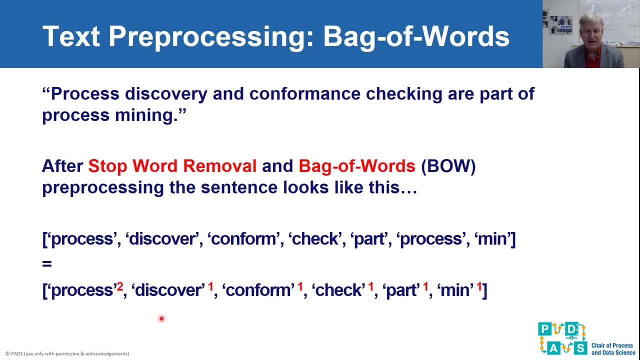 that we had seen before. So if we then use the bag of words- and we come back to that in a minute in more detail- we can basically in this sentence: we remove the stop words And then these are the things that remain. 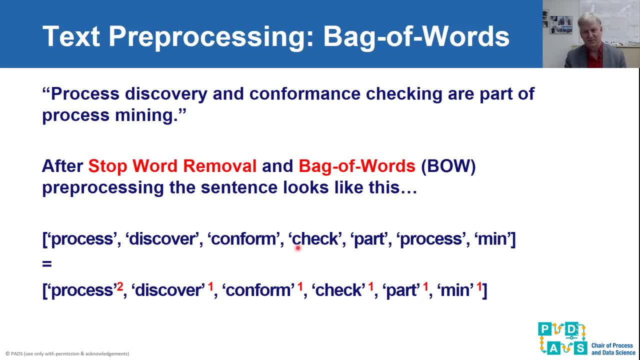 So we also applied, we chopped off the last parts of words. For example, checking has become check. And then we also do not consider the order to make it a fixed length representation And we indicate the frequency of each of these, let's say, remaining tokens in the document, ignoring the order. 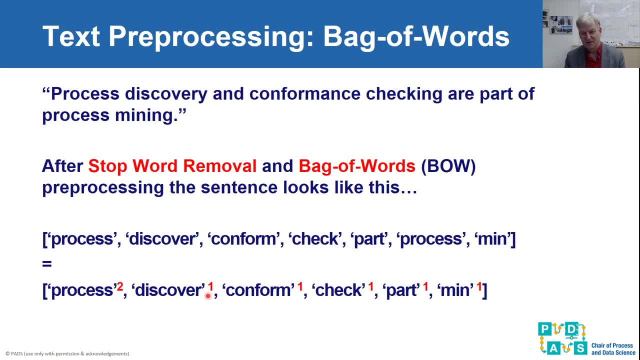 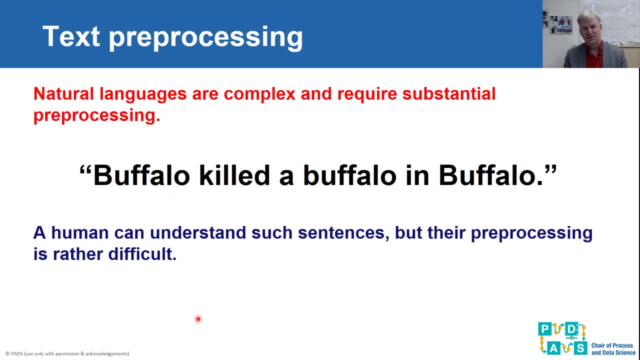 So this is called the bag of words model And bag refers to the notion of a multi-set that are sometimes called a bag And we indicate the token frequencies. So All of this is very tricky And, as I said in this lecture, I would really like to make you aware of the difficulties. 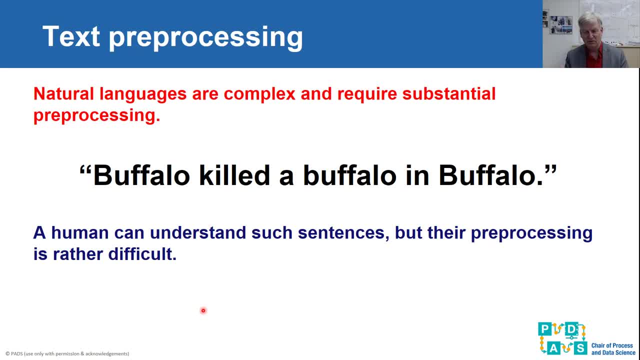 In the next lecture we will be much more technical, assuming a certain input And that all of the things that I've talked about now has been done already Here. in this sentence you see the word buffalo three times. You, as a human, understand what this. 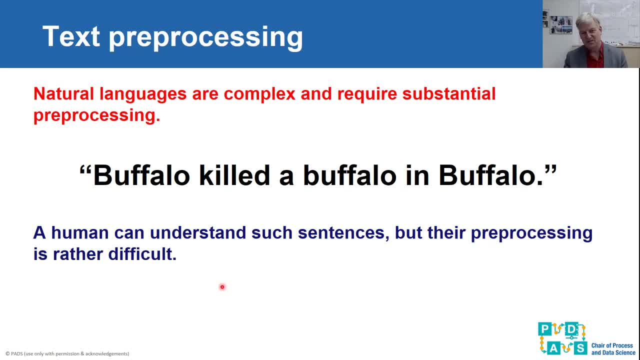 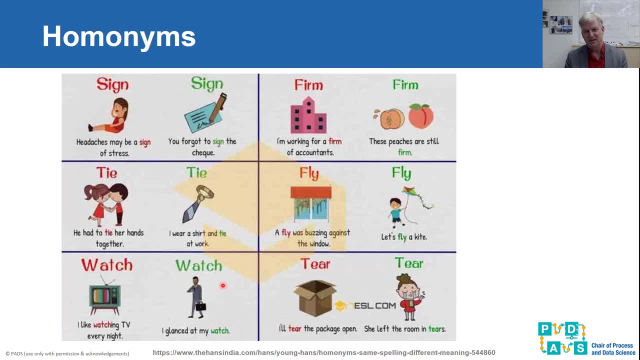 means. So there is a person, There's also a location, etc. So you can understand it, But for a machine it's very difficult. And so in the previous example we had buffalo. That in three times in one sentence, and each time buffalo appeared it meant something different. 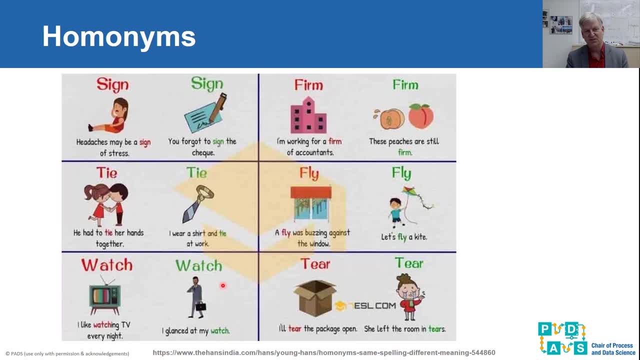 Of course, there are many examples of hominins, So these are words that can have completely differences meanings like so head edges may be a sign of stress, but you can also sign a check tie, watch, and watch like the verb, watch like the noun firm, like an. 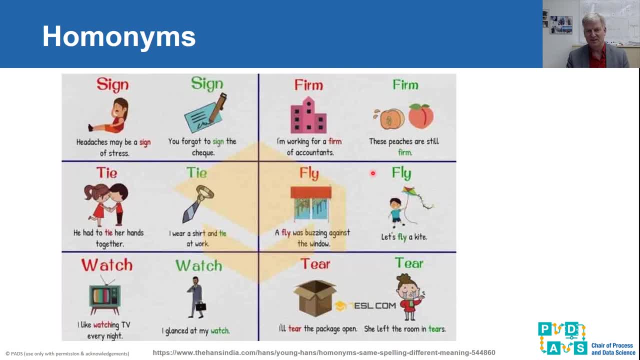 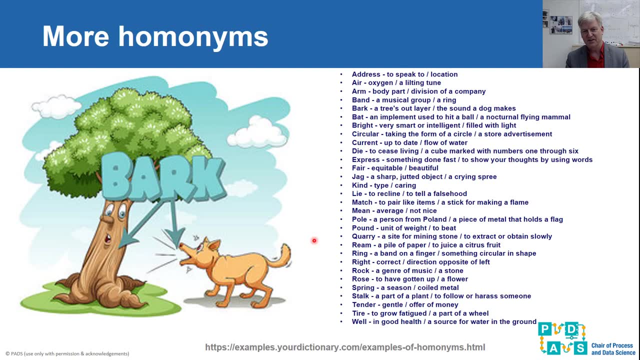 organization versus fruit that is firm, etc. etc. so there are many of such examples and if you, let's say, study that in more detail, you will actually be surprised how often the same word is used for completely different things and that you don't even think about it because it's in the context for a human. 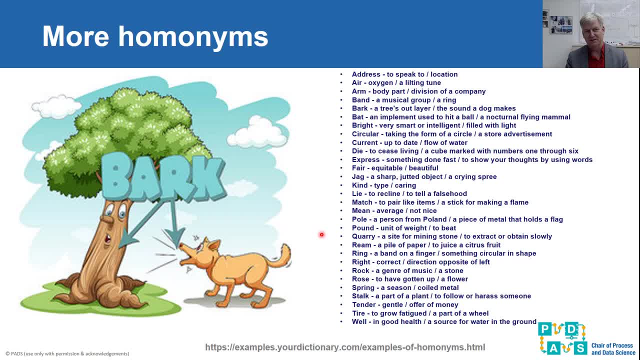 it is always completely clear, but of course for the machine this is very difficult and that the machine, if the machine cannot distinguish between different words, then it is difficult to distinguish between different words. and if the machine cannot distinguish between the bark and so the outside of a tree and a dog barking and dog making sound. 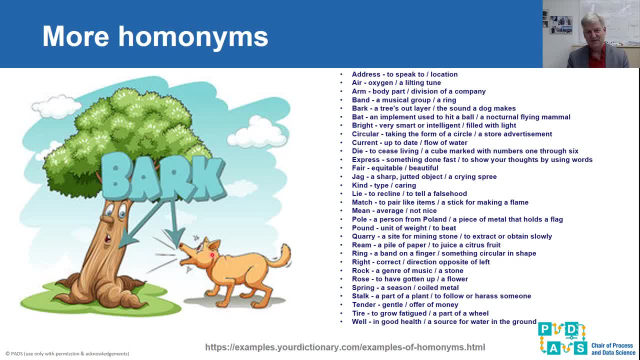 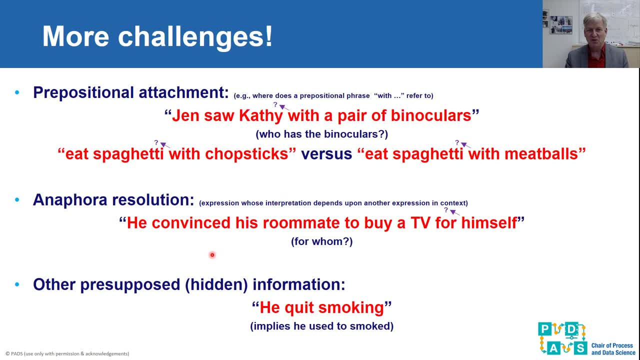 you can see that it may lead to very, let's say, odd conclusions if you then apply data science techniques on top of that. but there are many more challenges. so in sentences often there are references and showed an example at the beginning, and they are like a few of. 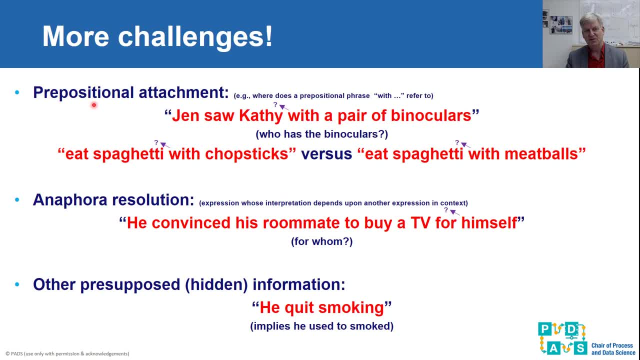 them are listed here, and so here we have the prepositional attachment, so we have like a phrase, for example, starting with: with: and so with a pair of binoculars, this part refers is attached to a person. is it attached to Jen or Kathy and you? 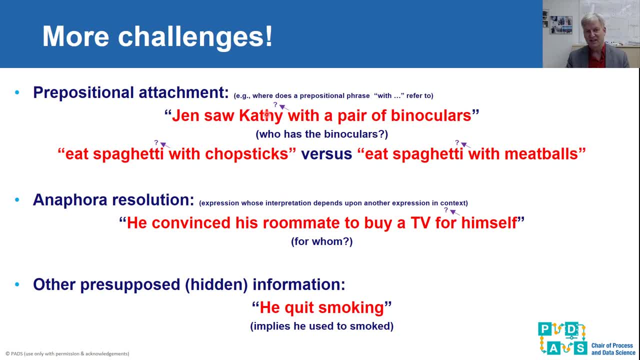 as a human, know that this with is linked to Kathy, to demonstrate that. and so for human, this is clear, but how would the machine notice? to make it clear, so here I have the sentence: eat spaghetti with chopsticks, eat spaghetti with meatballs. and now we focus on the part with: 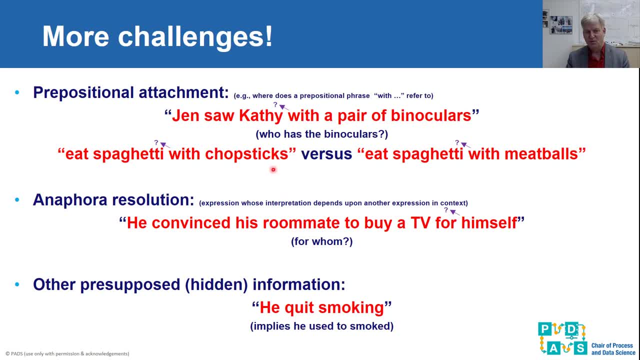 meatballs or with chopsticks? what does it refer to if we look at with chopsticks? it refers to eat. it does not refer to spaghetti because otherwise that would mean that the chopsticks would be in the spaghetti and you would have to eat them. if we look 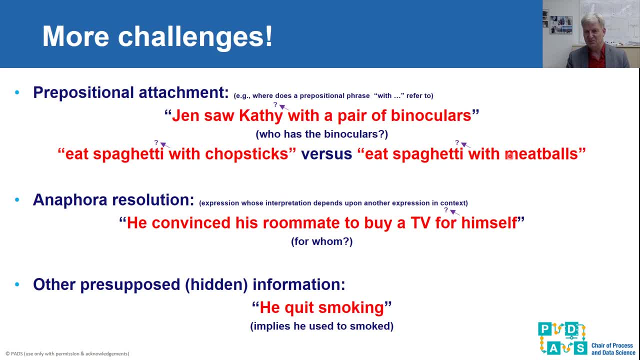 at each spaghetti with meatballs, then this with meatballs refers to the spaghetti right, that is, the dish that the person is eating. there are many of such, let's say, linking uncertainties that for human are obvious, but for a machine are incredibly difficult. and so he convinced his roommate to buy a TV for himself. so now the question is: where does 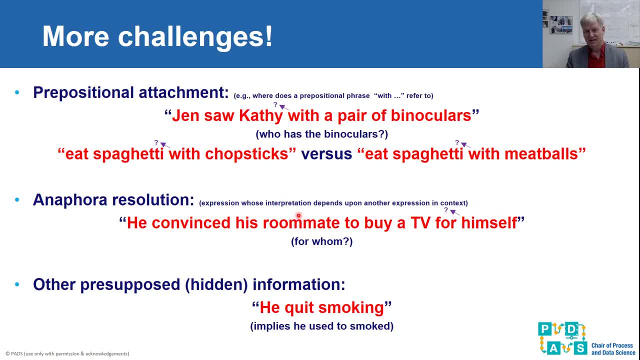 himself refer to. it doesn't refer to he, he, it refers to the roommate, and so you know that there are also, let's say, phrases that by stating something, there is an implication that could be used when you're applying data mining techniques, but that is implicit. so in the sentence he quit smoking, we. 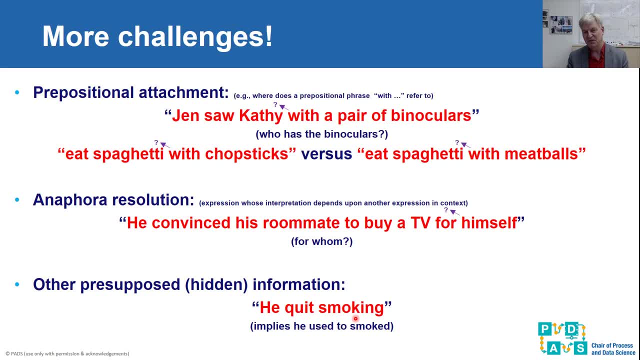 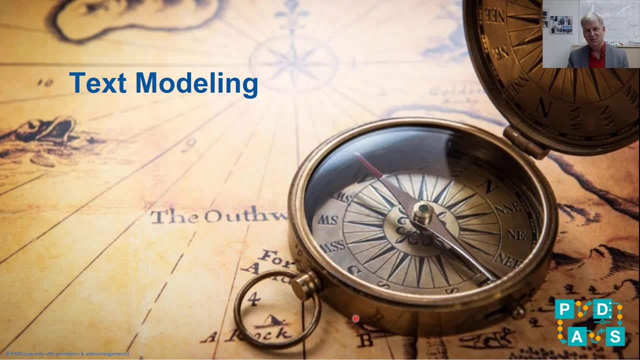 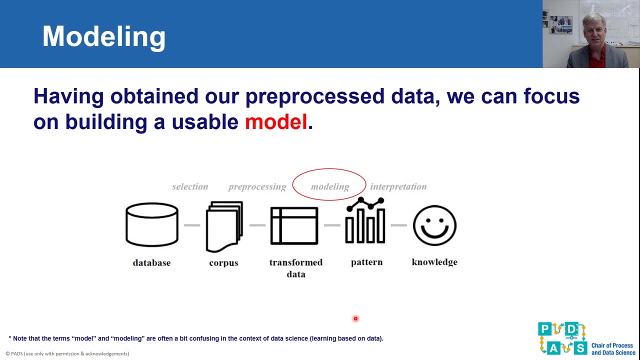 gained the knowledge that the person was smoking before. so so these are, let's say, many of the challenges. what is really really surprising is that if you apply, let's say, a reasonably crude methods to text, that sometimes it works surprisingly well. that is, and we will see some examples of that. so we are now coming, we have now done the. 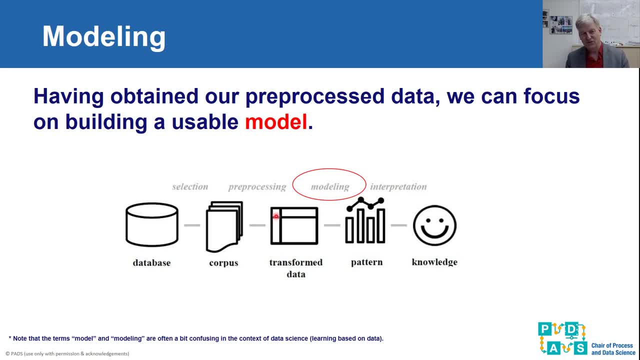 pre-processing, so assume that we have solved all the problems. so we have a corpus, and the corpus consists of documents and each documents consists of tokens, and we have done all the things that were necessary, and now we would like to start with the modeling. what is a bit? 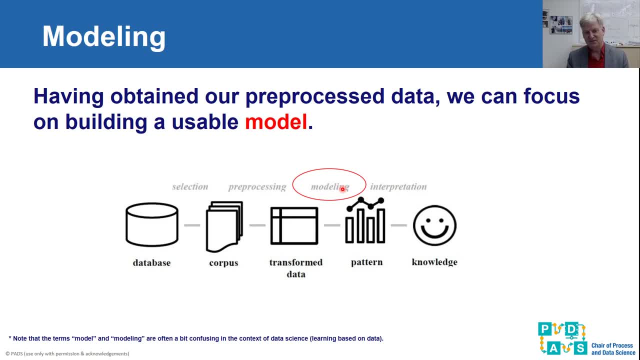 confusing in the field of data science is that how the words modal and modeling are being used. sometimes the model is the thing that comes out, so you could think of a decision tree or process model as a model, and sometimes it refers to the process of, let's say, 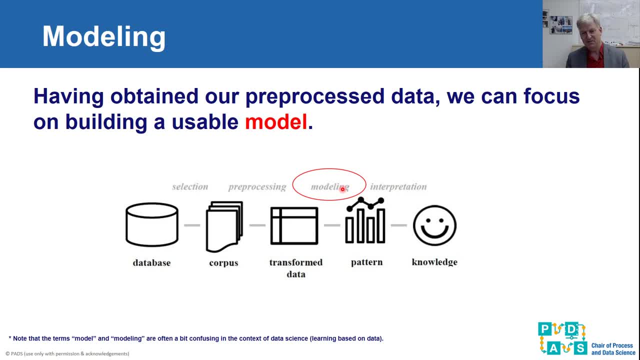 engineering, the learning technique, for example, setting parameters, deciding what the representation is, etc. etc. as the modeling. So sometimes it's more about the process of coming to some kind of artifact like a decision tree, and sometimes it is used for the artifact itself. 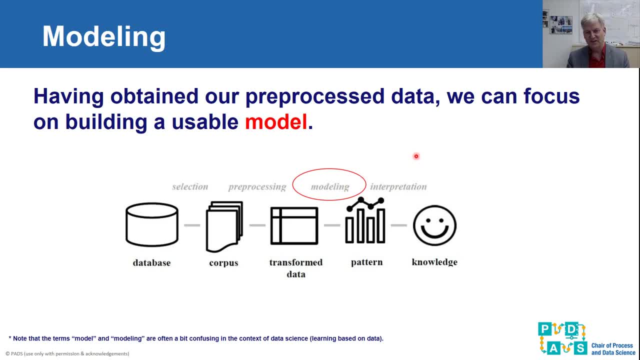 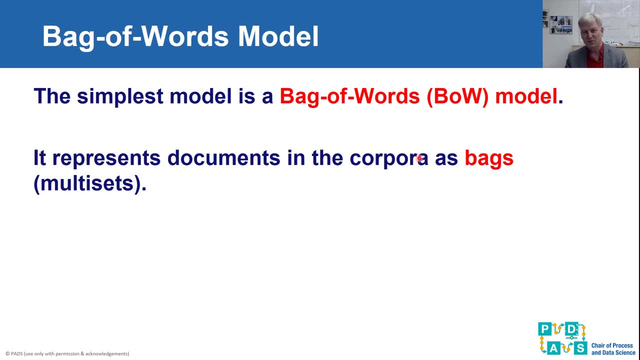 So I will be sloppy when I use this term, but it should be clear what I mean. So we want to work towards the bag-of-words model as a starting point. So the bag-of-words model represents each document in the corpus as a bag of tokens. 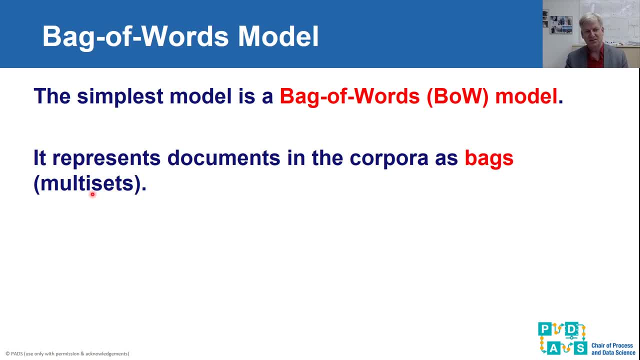 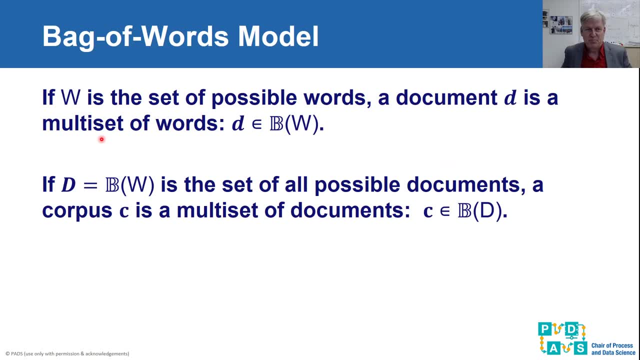 Tokens correspond to words in this setting and the word bag refers to the notion of a multiset. So here I can find- So I will normalize this Note- that when I'm using words in this setting, these words actually correspond to the remaining tokens after doing all the preprocessing. 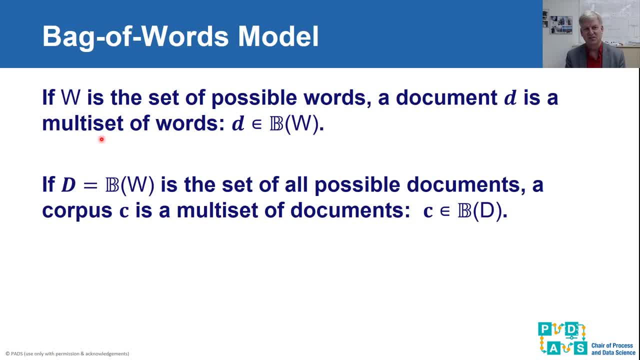 But because they often are words, that is easier, It's common to call it like that. So W is the set of possible words, Then a document is a multiset of words. Note that we know how frequent each word appears in the document, but we do not know the order, because that's now the abstraction that we have chosen. 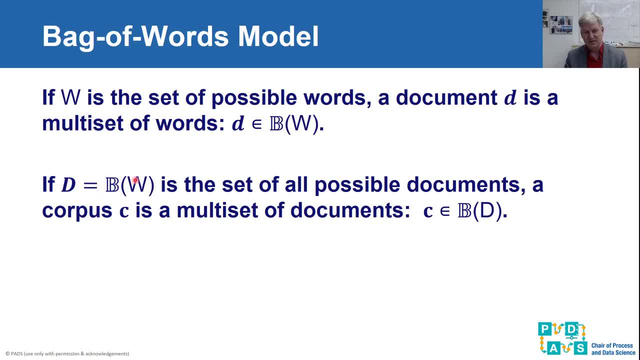 D is equal to the multiset over. W is the set of all possible documents, And so these are basically now. so every document is like a vector indicating how frequent each word appears, And a corpus can be seen as a multiset of documents. 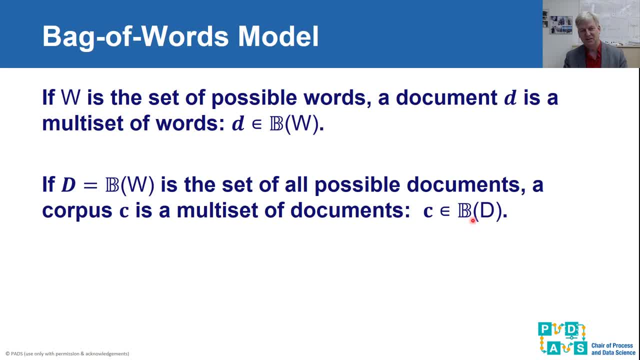 So D is equal to that. So now we have a multiset of a multiset of words. Why is there a multiset here? We are using a multiset here because in principle- I don't know- two tweets could be completely identical. 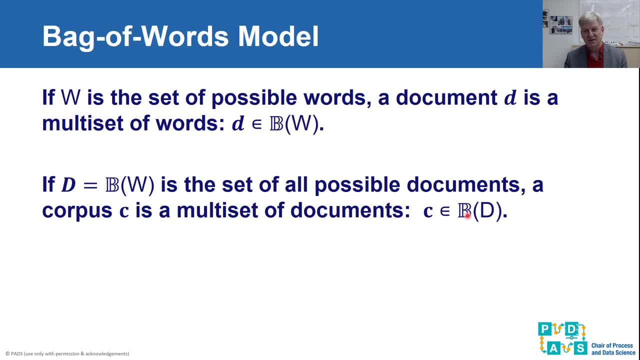 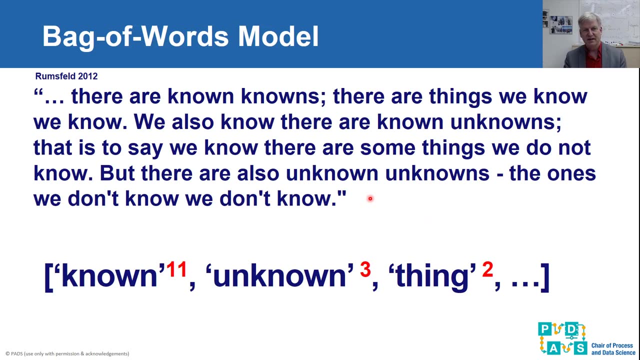 Although they are different, the text is exactly the same And that's why you can think of them as as a multiset of a multiset of words, That is, a corpus C. So if we look at the bag of words model, I already explained it before, but because it's a key concept, I show some more examples. 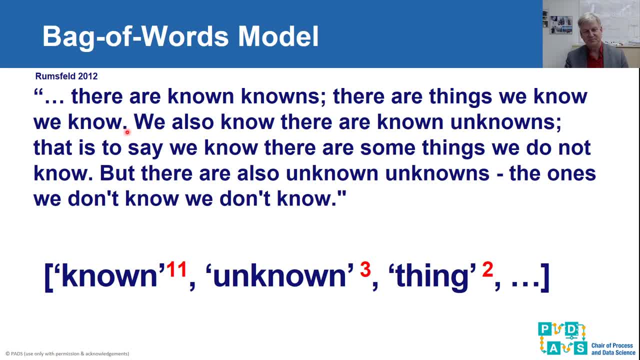 So this is, let's say, a piece of text of a statement made by Rumsfeld about like in the context of the weapons of destruction. he was saying these nine sentences where he talks about known unknowns, unknown unknowns, et cetera, et cetera. 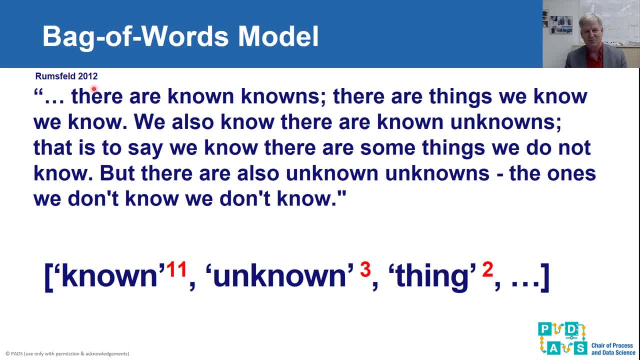 If I translate this to using the bag of words model, we get known unknown and thing and many other words that happen only once. So this is the bag of words model. So this is the bag of words model. So this is the bag of words model. 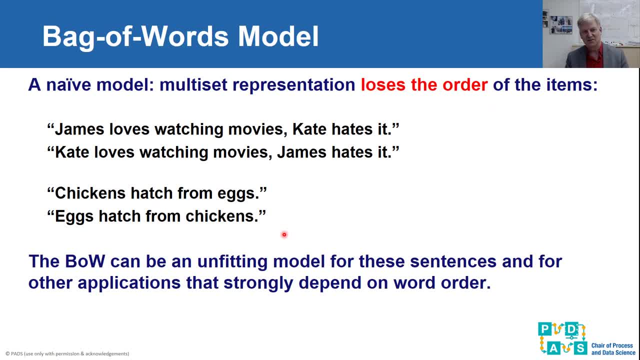 So this is an example of the how this works. Of course, there are many sentences that have the same bag of words representation. So these two sentences here, where I basically swapped the role of Kate and Jones, if we look at them through the bag of words view, they are identically. 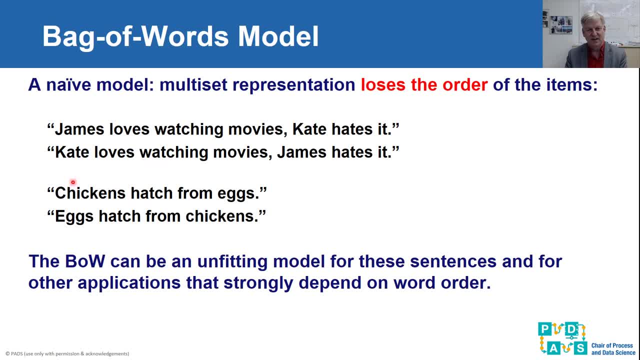 So their abstraction is exactly the same. The same if we look at these two sentences. The same if we look at these two sentences, but also if we use the bag of words model. the same if we look at these two sentences, but also if we use the bag of words model. 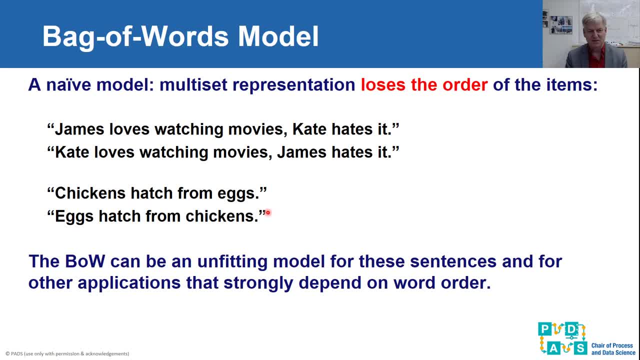 they map onto the same multi-set of tokens. they map onto the same multi-set of tokens. Of course, this becomes problematic when the order of words is incredibly important, And this will be a topic that we will cover. And this will be a topic that we will cover. 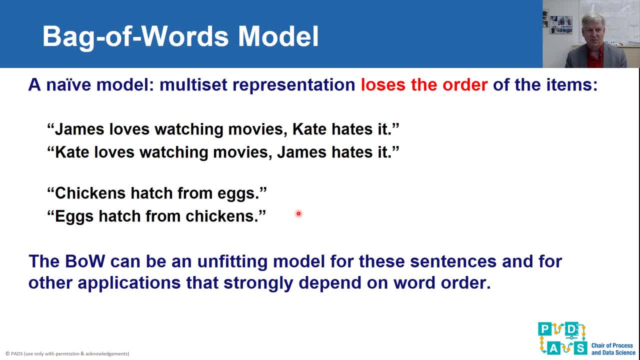 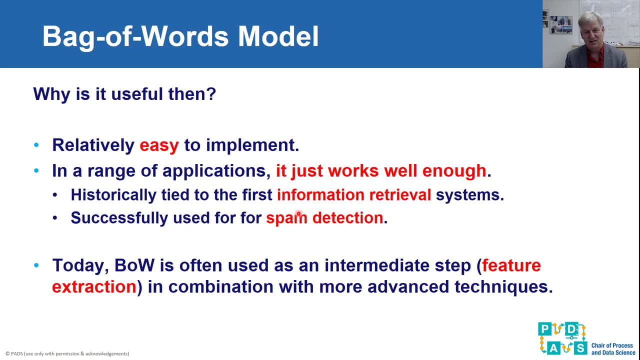 let's say in a lot of detail in the next section. But here we assume that we have these two sentences, that we have this abstraction. why is this abstraction working? as I said, sometimes it works surprisingly well, it is easy to implement. it has been. 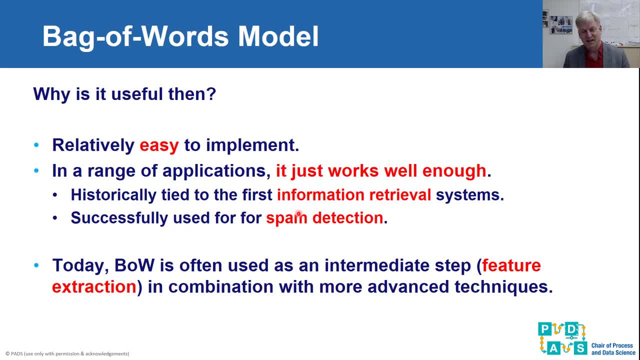 successfully applied in all kinds of domains. as I said, later we will look at more refined representations, where we are also taking into into account the ordering of words, but now in this lecture we just use the bag of words after we have done all the pre-processing that I talked about. 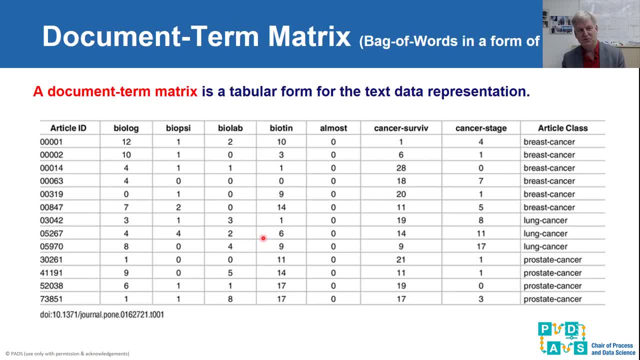 before. so if we do this, then we get a representation that should look very familiar to you. so we can see every document as an instance. so every document is now mapped on to a document as an instance. so every document is now mapped on to a document as an instance. so every document is now mapped on to a. 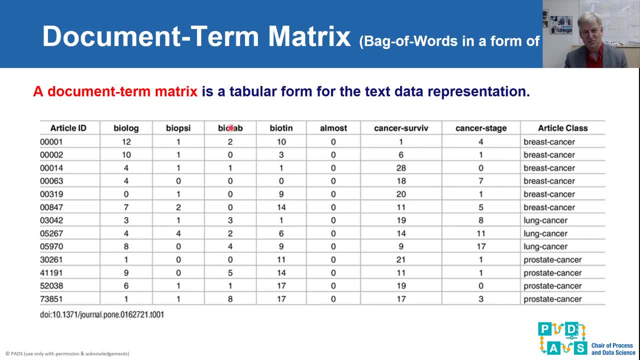 row and we can indicate for each word what their frequency is, because we are using the bag of words model. and there could be other attributes like, for example, a certain target variable, like the article class. so if I look at the representation that I just showed to you, you can already imagine that you can. 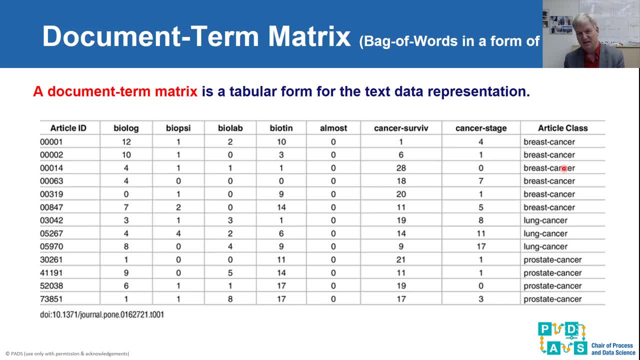 use such a representation, for example. so if I would look at that, I hope that you immediately see: okay, we can do logistic regression, we can apply support vector machines, we can apply neural networks based on on this, and then the goal would be that we would learn a predictor model that predicts what the article class is. I 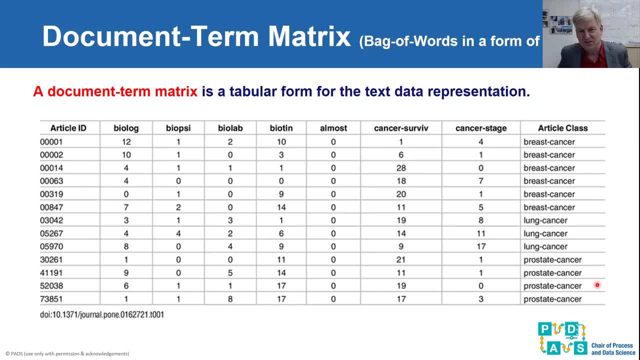 think everybody can see that the article class is a model that predicts what the article class is. I think everybody can see that you can use these types of input. if I for a moment forget about the article class and I just look at the vectors indicating the frequency of each, 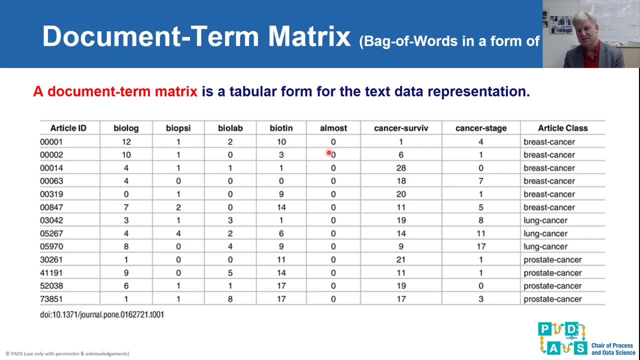 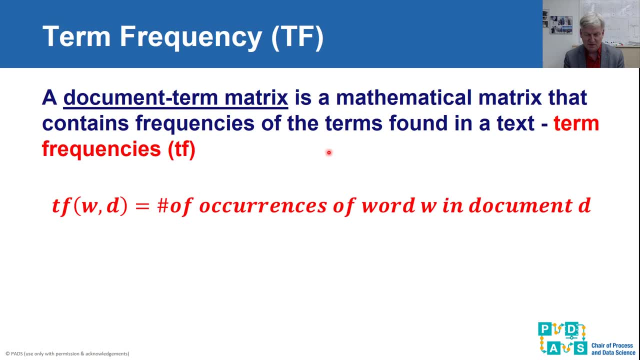 word. I think everybody can see that. okay, this can also be used for clustering, for example. so we are getting close to where we want to do, to want to be. however, we have the problem that looking at the absolute frequency of a word in a document is not such a 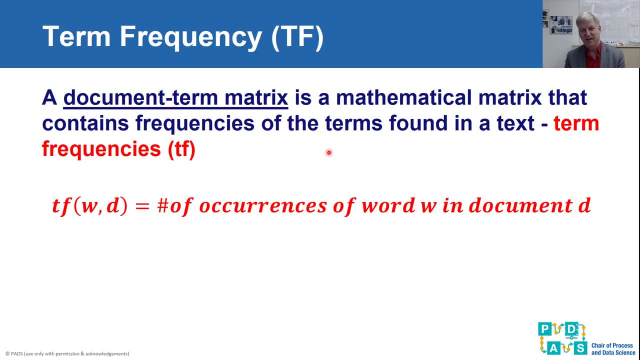 good idea, and so documents may vary incredibly in length, and it could be that there could be birds that are super frequent but that appear in almost any document in the corpus that we are considering. that is why we compute two metrics that we combine. the first is term. 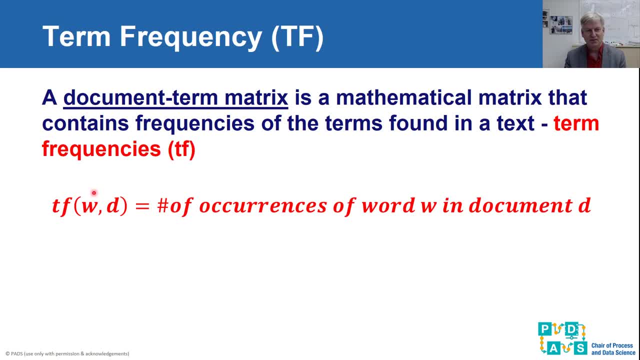 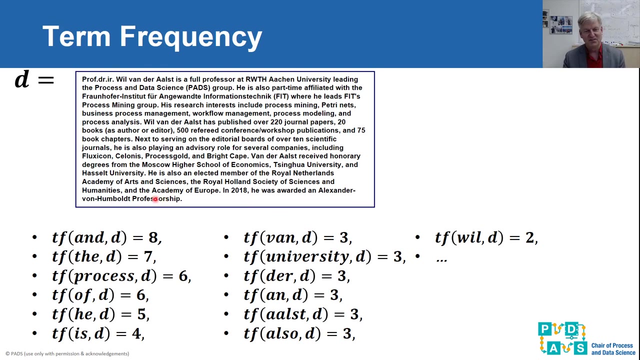 frequency and turn frequency of a word in a document. as a w refers to a word or token and d refers to a document, this expression simply counts. how often does that word appear in that document? that's super simple. so here i took, let's say, an older version of my cv and i apply, let's say, 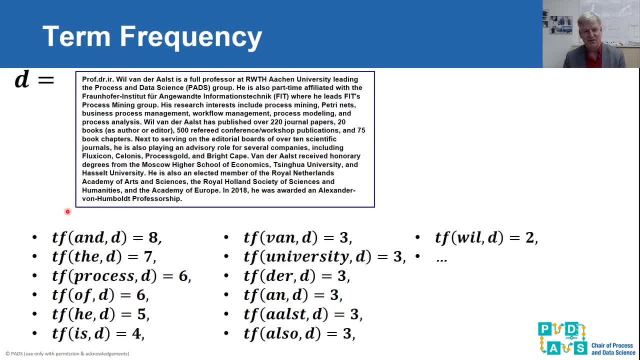 uh, i compute this tf function and if i do that, i see that, for example, the word and is appearing eight times and my first name is appearing twice. so you already immediately see that the problem with the fact that things like and, and are frequent, and if we did not remove them already? 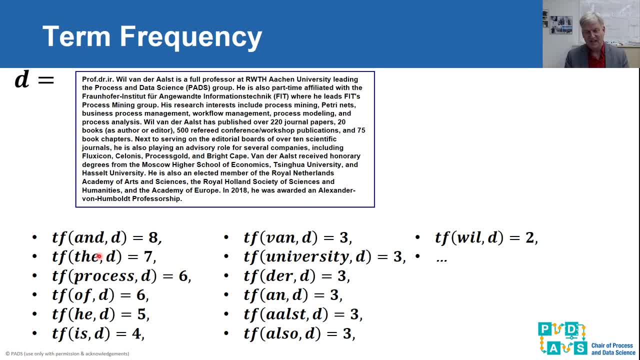 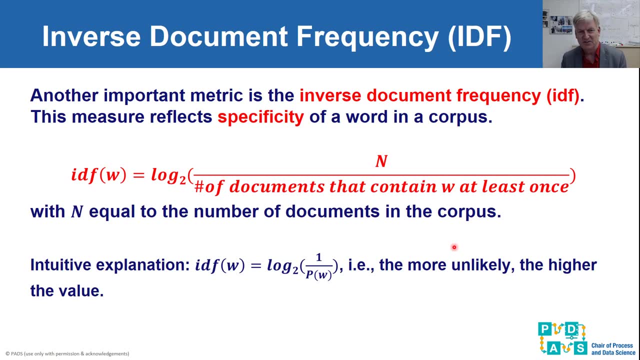 using when we were considering stop words. they have a relatively high weight and, like my first name, uh, has a relatively low weight. so, because the absolute frequency does not say everything, we also look at the inverse document frequency, and this refers to how specific is a word in a certain collection of documents. so in 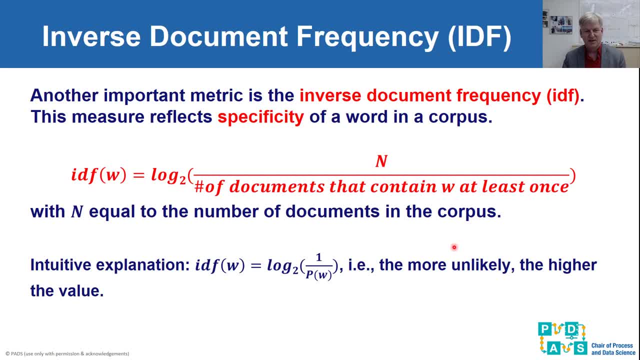 a particular corpus. so the formula is as follows. so if we look at the uh inverse document frequency of a word w in the context of some corpus that consist of n documents, then this is the logarithm of n divided by the number of documents that contain w at least once. so what is the maximal number of documents that may contain? 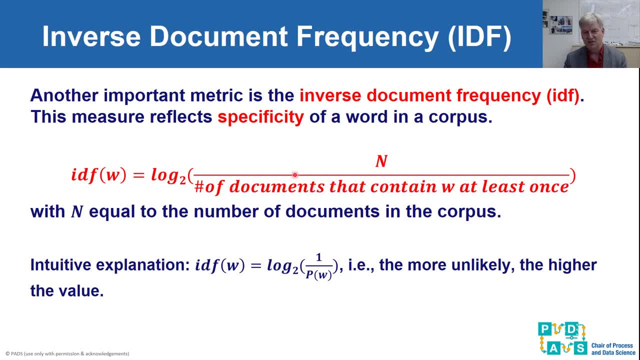 this word w. that means that there is j. that means that we have some number of documents That can only be n. So it can be that we have n divided by n and that is equal to 1.. And if we take the logarithm of that, it's equal to 0. 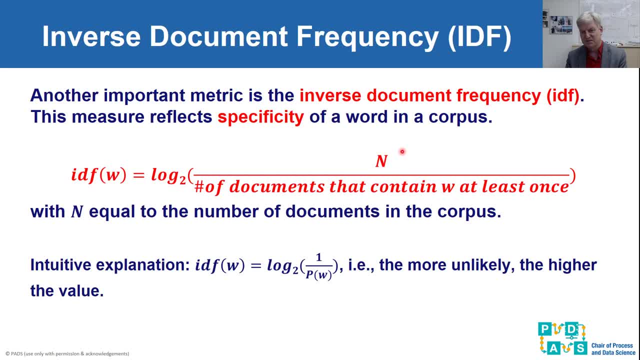 If we now have a large number of documents- so let's say n is 1,000 or 10,000, and we look at the word and the word appears only in, let's say, 10 of these 10,000 documents. 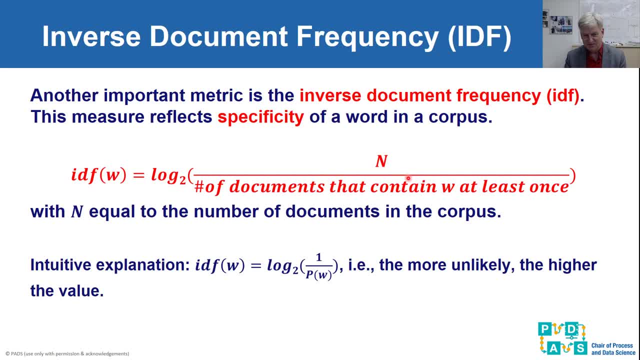 then we have 10,000 divided by 10, and then we take the logarithm and then we have a higher number. So the more rare a word is, the higher the inverse document frequency gets. So the intuitive notion that you should have is that 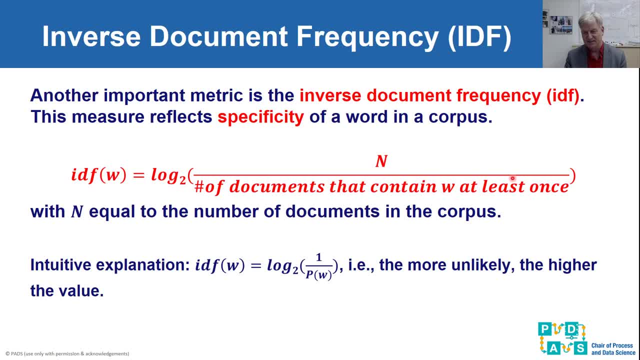 this is the number of documents that we have. So this is the number of documents that we have, And so n divided by this, I can basically take 1 divided by the number of documents that contain w at least 1, divided by n. 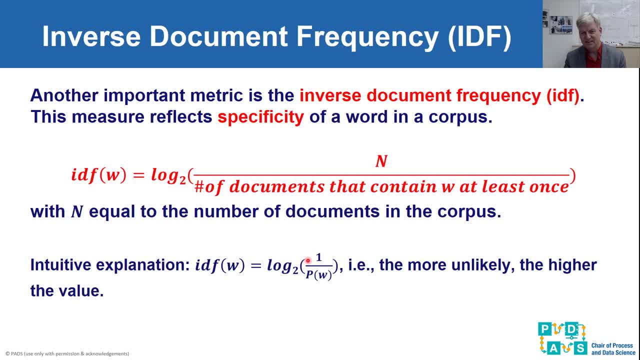 And if you write it like that, then you realize that this actually corresponds to this, where you can interpret pw as the probability that a word appears. So pw in this example corresponds to the number of documents that contain w divided by the overall number of documents. 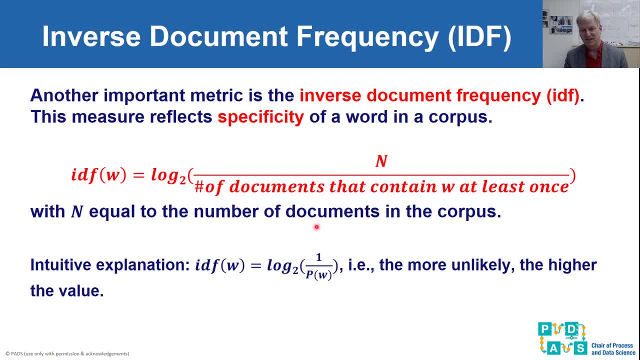 And these two terms are then, of course, exactly the same. We are using the inverse of this as an estimator for the probability that a word w is present in a random document in our corpus. So that is the intuitive notion, And just like a number example to help you a bit. 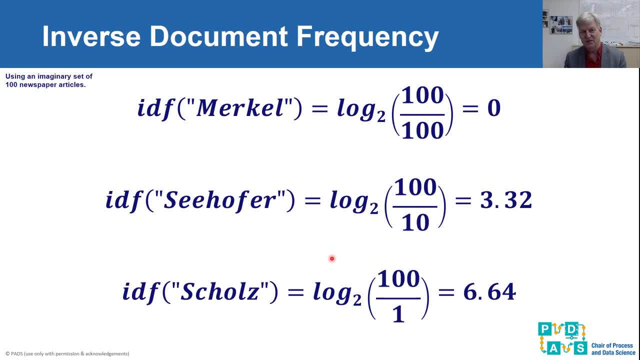 So this is based on an imaginary collection of newspaper articles where we look at these three words- so Merkel, Seehofer and Schultz- and we look how frequent they are. So there are 100 newspaper articles and we divide it by the number of news articles. 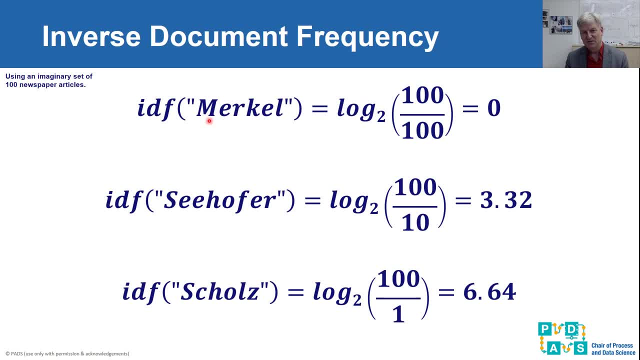 where a particular name appears. So if if Merkel appears in all of these 100 documents, then this is equal to zero, so it carries no information. It doesn't make the document special in any way. If we look at the IDF of Seehofer, then he's appearing in 10 out of these 100 articles. 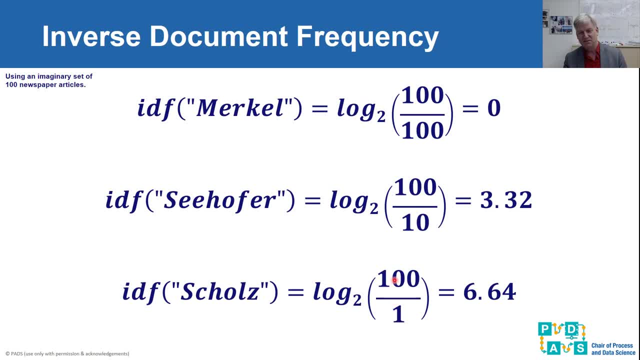 then we have this. and if Schultz is only appearing in one of these 100 documents, then we have this. and if Schultz is only appearing in one of these 100 documents, then we have this. and if Schultz is only appearing in one of these 100 articles. 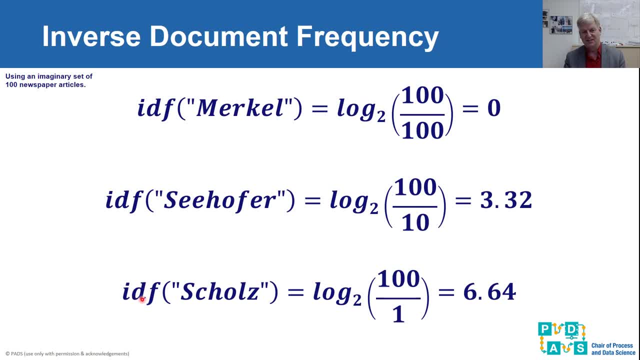 documents, then it has an ID f of 6.6.. So now we have two forces. We have one force. that looks okay. if a certain word is highly frequent in a document, it must be very important for the document, a very characteristic. but if it also appears in many other documents, 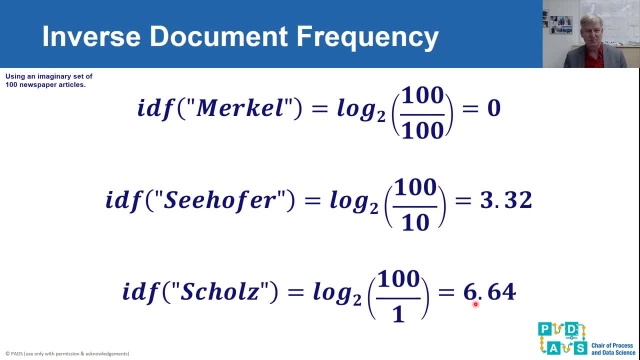 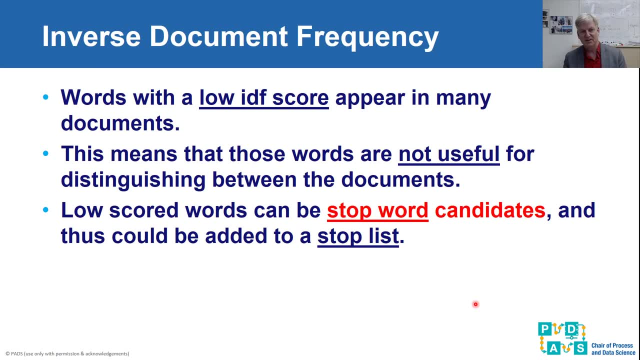 then it becomes less important. So we are now simply going to multiply the two things that we just had. So this is summarizing a bit what I just said. And so words with a low ID f score appear in many documents. If it appears in every document, then the score. 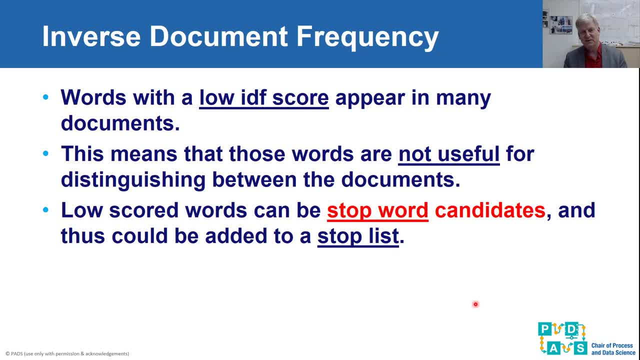 is even equal to zero, And that means that these words are not useful to distinguish between Between documents. You can use this as an approach to identify stop words. In the text that I showed earlier, we could see that D was the most frequent word, So if D is appearing, 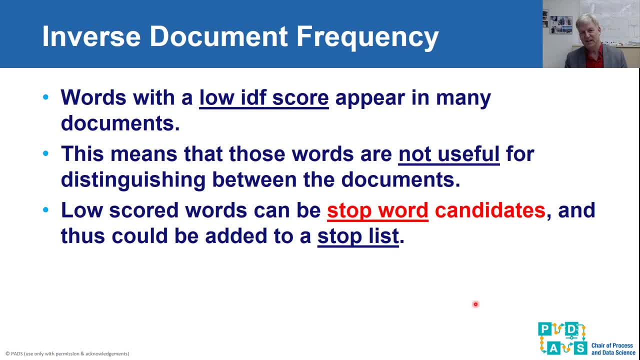 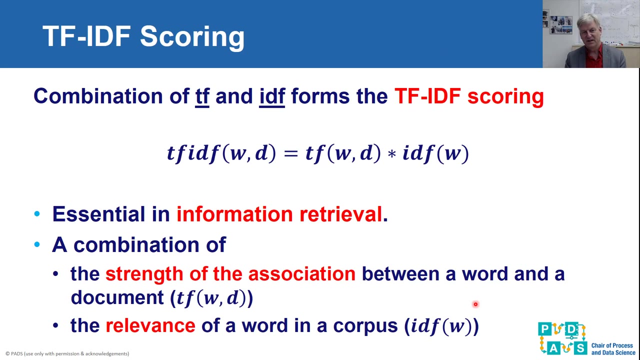 in every document, then it will automatically have an ID f score equal to zero Right, And if the token has an ID f score close to zero, then we could add them to the stop list and remove them because they carry no information. As I said, we would like to combine these. 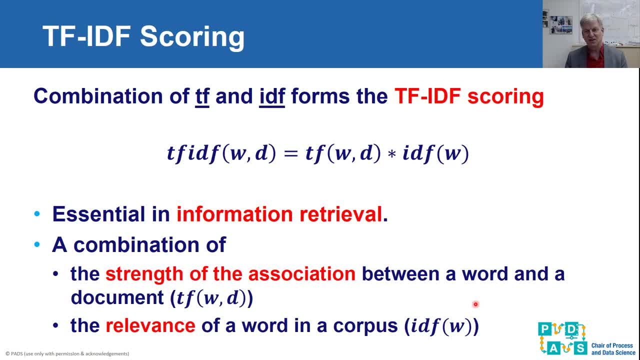 two forces that we have and this is called the TF ID f score. So the TF ID f score of a word and a document in the context of a particular document is equal to zero, And particular corpus is tf. so how many times does the word w appear in document d times? 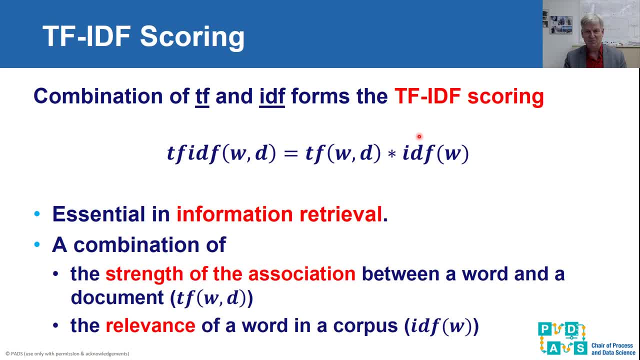 idf w, And remember that idf w is equal to 0 if the word appears in any document, and this value becomes higher if the word is more rare, because it's a logarithm of 1 divided by its probability. And this combination seems to be a good combination, Like many. 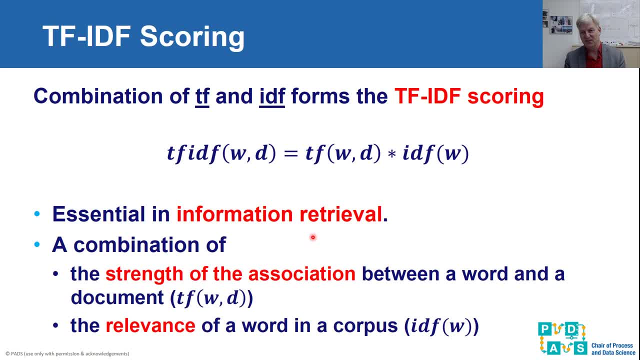 things, let's say, in the setting of text. mining is that it is all a bit vague and you could ask: okay, why do you take the logarithm here and not something else? but this is based on experience. but there is no logical reasoning why this would be the best measure, and one. 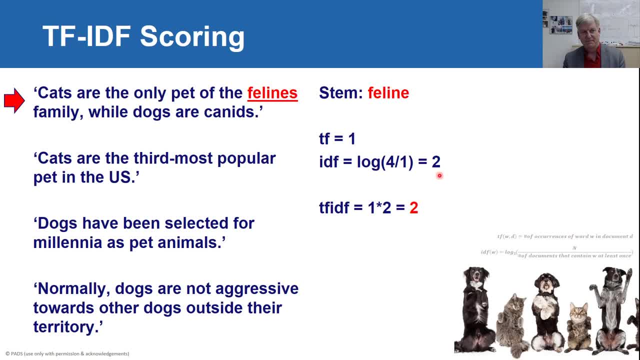 could not? Just to illustrate the principle a bit, suppose that we look at this word right, and I'm assuming that we are also doing the pre-processing a bit on the fly. So now we are interested in the tf, idf score of this word, feline. then we look, okay, where. 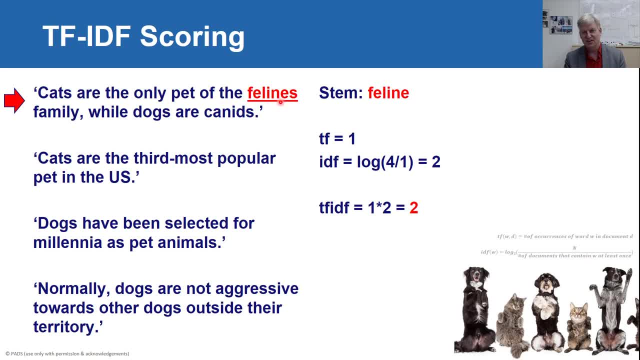 does it appear, and in this document. so the focus is now on this document- it appears once and it doesn't appear in any of the other documents. So the tf score is once one, because in the document that we look at it appears precisely once, and then we multiply this by the idf score. 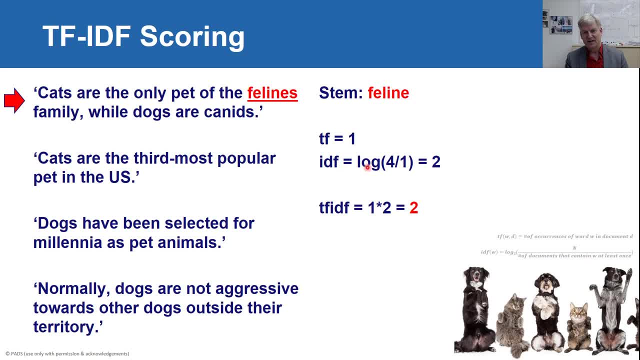 of this word and the word is: there are four documents and it's only appearing in one of them. So we get a logarithm of four is equal to two. so the tf idf score is one times two is two. Now we look at the word cat as another example. 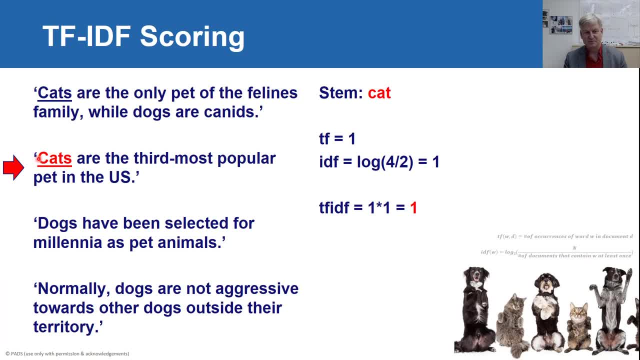 So we look at the word cat and we now look at this document. So if we look at, what are the documents where cat is appearing, That is, in the top two, and in both of these documents is occurring once. Our focus is here. so the tf score is equal to one, the idf score we basically look at. 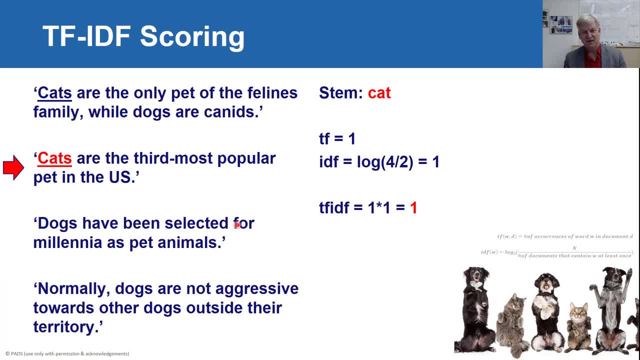 all the documents- there are four of them- divided by the number of documents that contain cat in some way, and that leads to an idf score equal to one. So we take the logarithm of two, Cat is equal to one. And then we do the tf: idf score of cat in this document is equal to one. 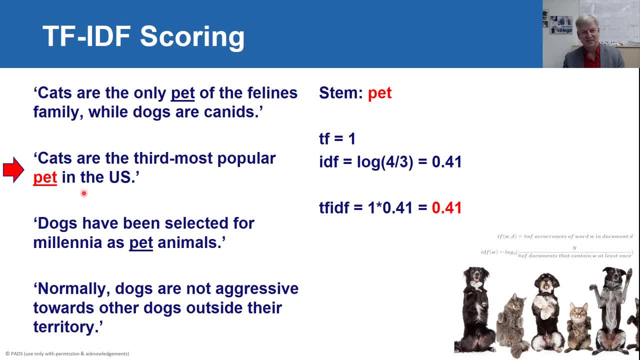 Now we look at pet. but I think you get the idea. Pet is appearing once in this document. it is appearing in three documents, So its tf idf score is 0.41.. So both cat and pet appeared once. But you can see that the tf idf score is here 0.41, and in the previous setting it was equal. 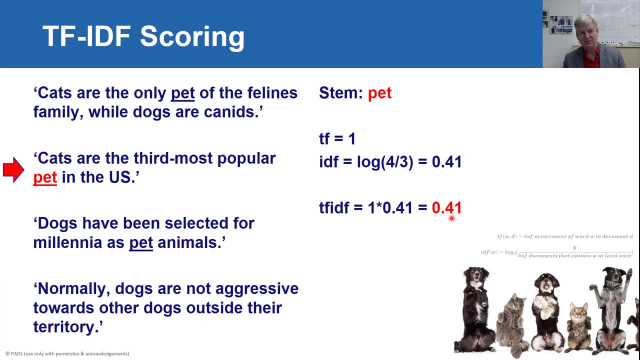 to one. So we see that it is dropping because the word pet is appearing in more documents, which is the effect that we would like to have. Here's an example of a text where, let's say, the same word or the same token is appearing. 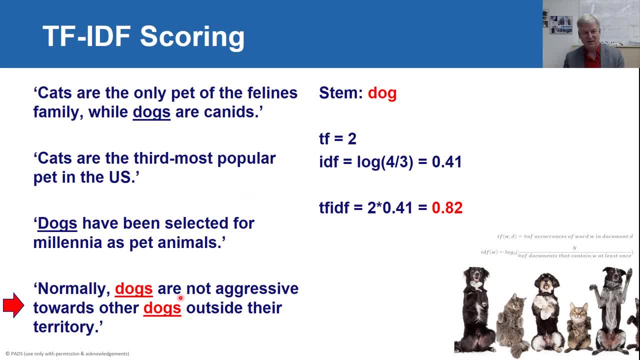 twice. So note that we are doing stemming. And then we look at the tf idf score. So we look at dog. Dog appears twice in this piece of text. We would now like to compute the tf idf score for this document and the token dog. 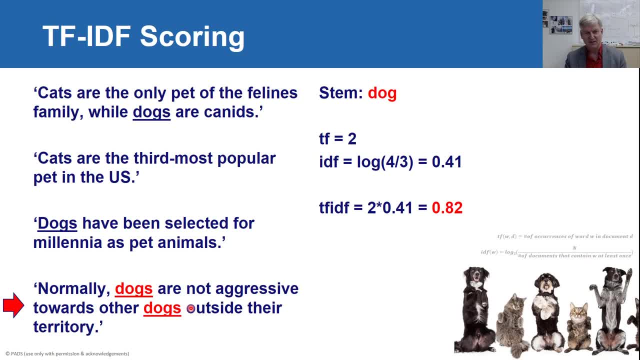 Then the tf is equal to two, because it is appearing twice in this document- And the idf score. And then we look at four divided by all the documents that contain the word dog, And there are three of them. So we get this score and the tf- idf score is the number that we get by multiplying these. 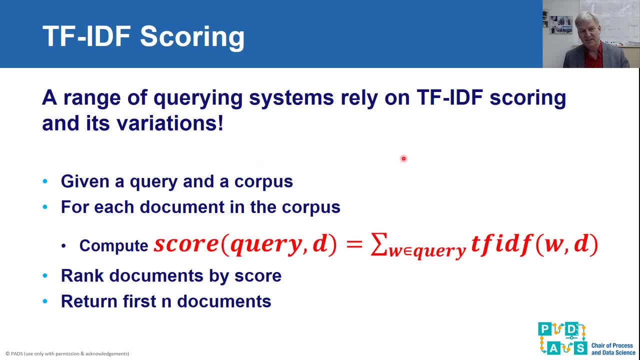 two values. So this hopefully gives an idea of how to score these things. It is super simple, but these are the things that can be used, for example, in querying. These are the things that we can do to preprocess our data, to apply any of the data science. 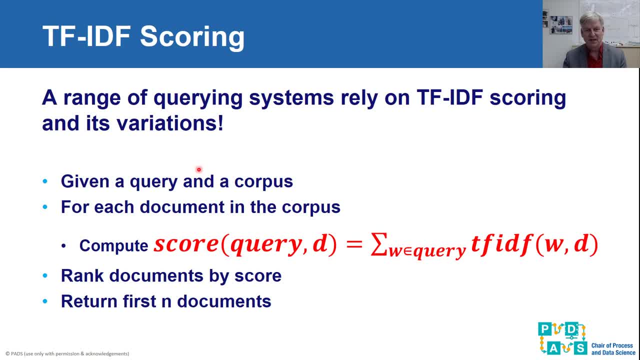 techniques that we have looked at before. So here is the example of information retrieval. So we have a query, The query is just, let's say, a bag of words, And we have a corpus, and the corpus is a set of documents, and every document is represented. 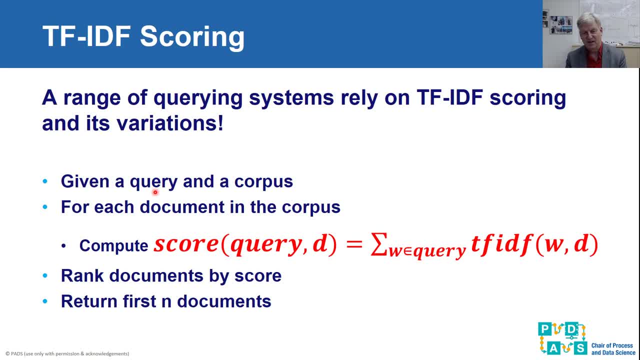 by a bag of words, And then we can compare the query with respect to each document. So the query is a set of documents. And then we can compare the query with respect to each document. So the query is a set of documents. So this is a bag of words. 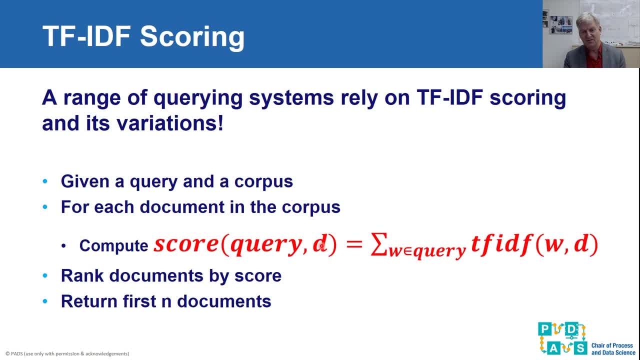 D is a particular document, So that's also a bag of words, And what we do is that we sum over w. That's our query- And then we compute the sum, summing up all the tf, idf values of all the words in. 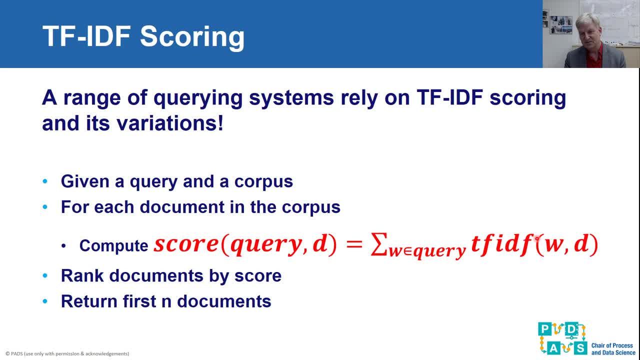 the query over that document And note that this tf idf computation is taking into account how rare this word w is. so if there is a search term in the query that is a word that is very infrequent and it appears many times in a certain document, then it will get a very high score because of that. 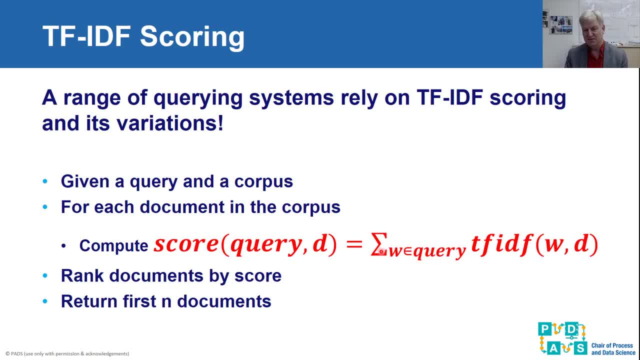 word. So we sum that like what the absolute value is is not so important, because we can simply rank the documents based on this score and we can return the first end documents. so, using this principle, you can build your own, let's say, primitive search engine based on just looking at the 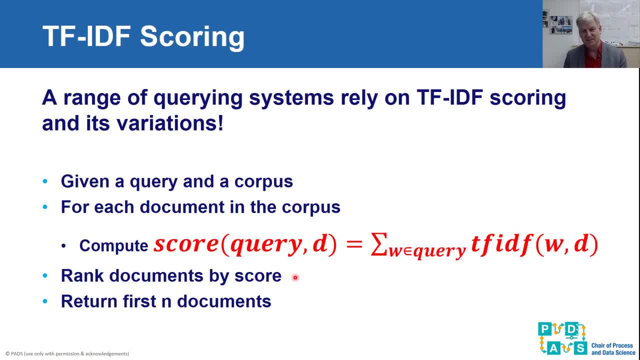 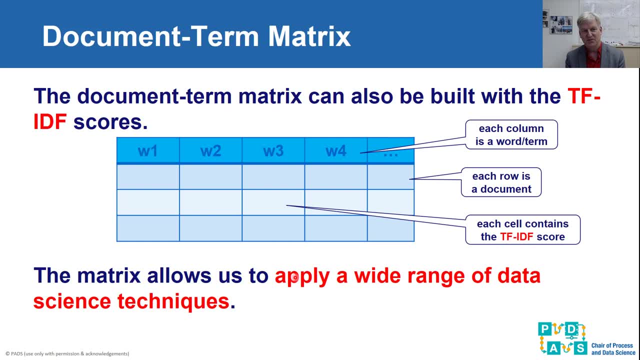 text itself and not at the links. so so so we already had a document term matrix illustration before, but before we were considering the numbers for every instance- and an instance corresponds to a document- the numbers were indicating the absolute frequency of a word in a particular document. So here, 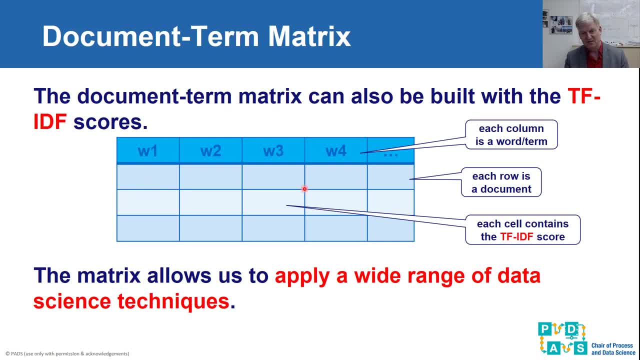 every column is a word, every row is a document, so an instance is a word and we can write the number and we can call it the absolute number. So we have our absolute number and we can now replace this absolute number by the tf-idf score, and that typically works much better. 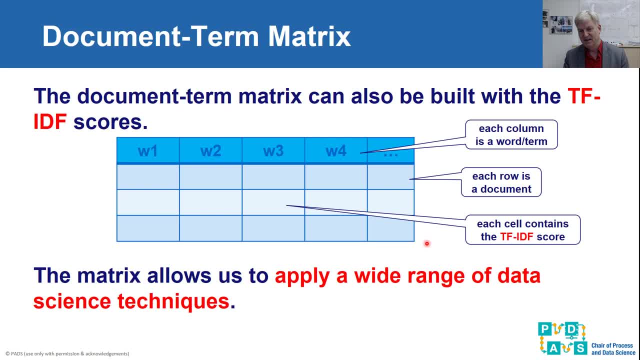 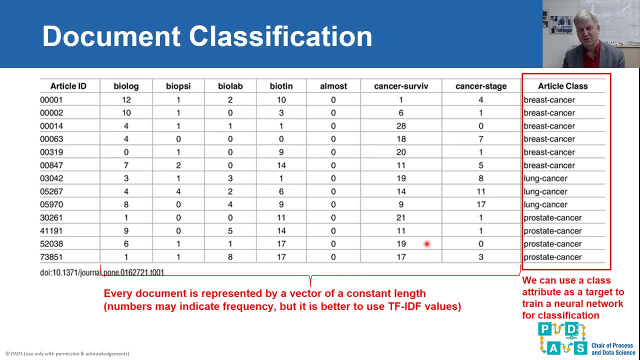 because the rare words that happen frequent somehow have a bigger weight. So this is what we showed before, so now these numbers that are here could be could either refer to the absolute number of a word appearing in a document, or it could be based on the TF-IDF score. 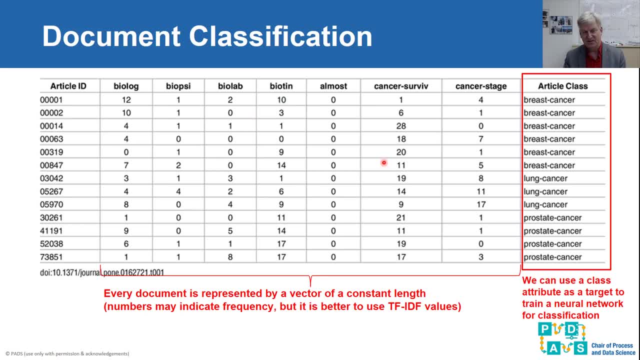 In both cases what we get is a vector, and if every document also has a label like a target feature, and the target feature is called here article class, then we can generate supervised learning problems. So what we often see is that the same documents or the same instance can have different types. 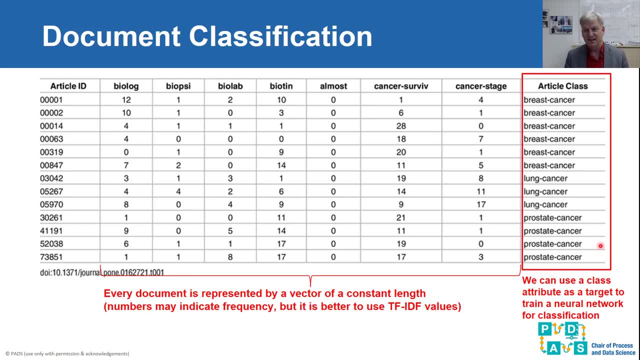 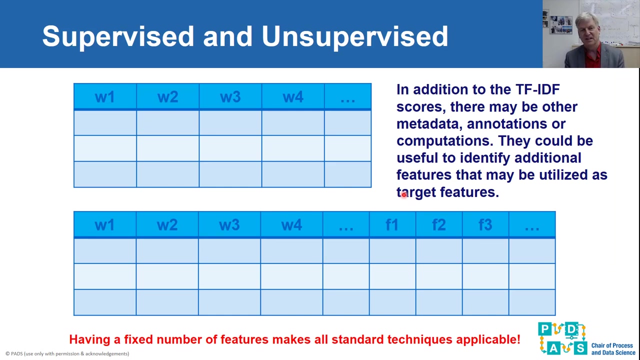 of target features and we can generate different- let's say, supervised learning problems based on the different target features. As I mentioned, it's better to use TF-IDF values in such a matrix rather than the absolute frequency- And this is what I just said- is that through these transformations we get the problems. 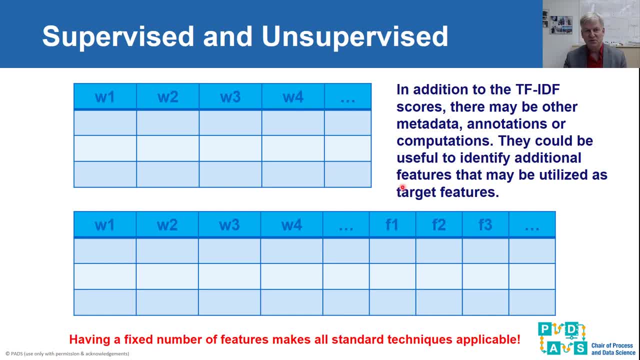 that we have been looking at before. So if we do not have, let's say, target features, clearly identified target features and, just, let's say, the TF-IDF scores, we will be able to say that the value of the target feature is not a problem. 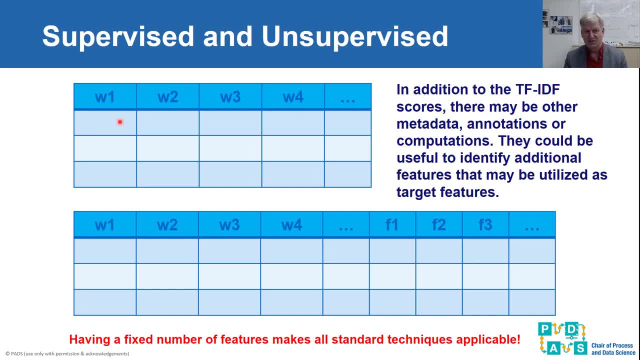 It's just that it's not a problem. But the problem is that if we do not have a certain target feature, then some of the other elements, like the target features, we can generate a supervised learning problem and in addition, we can use a bit of other things, such as the LIVS, the 하면. 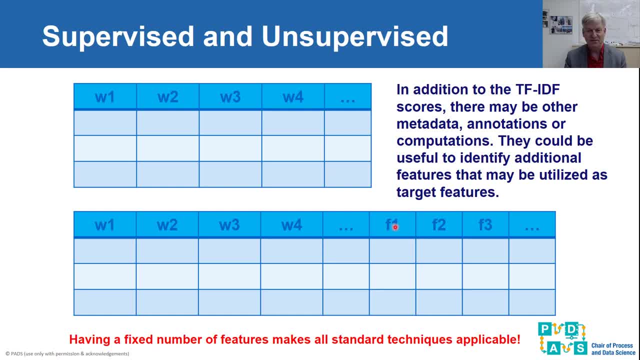 so we just pick a target feature, for example f1, and then we have a supervised learning problem. so we can use decision trees. we can use logistic regression, depending on the, so whether the target feature is categorical or numerical, we may use normal regression or logistic regression. if it's categorical, we can also use, let's say, support, vector machines and 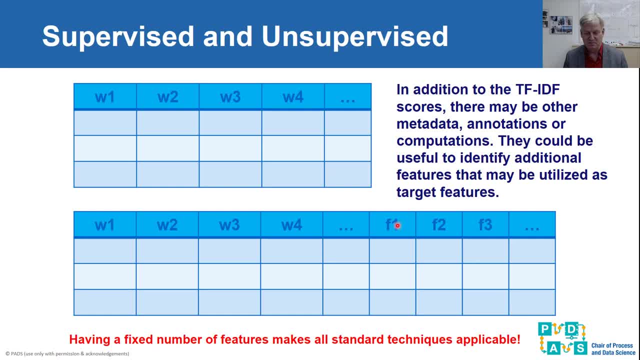 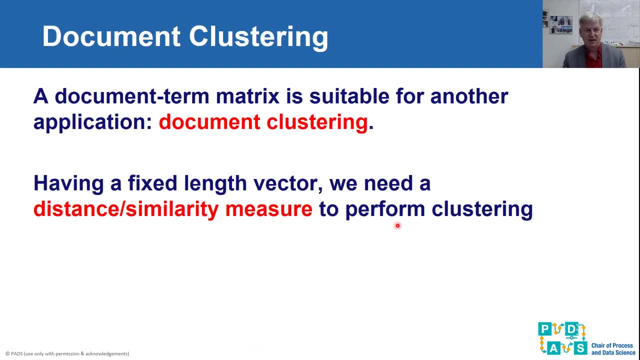 in both cases we can apply neural networks, and so this is the bridge with all kinds of techniques that you have seen already before, so we can use it for for clustering. if we look at clustering, then we need to, of course, look at distance measures. in principle, you can. 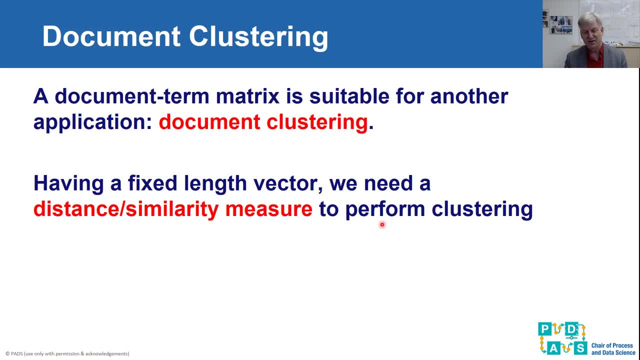 apply anything that i showed to you before. if you are using, specifically, if you're using, let's say, the frequencies of words instead of the tf idf score, then if i have a document that has twice as many words as another document, it becomes a bit tricky to compare them. 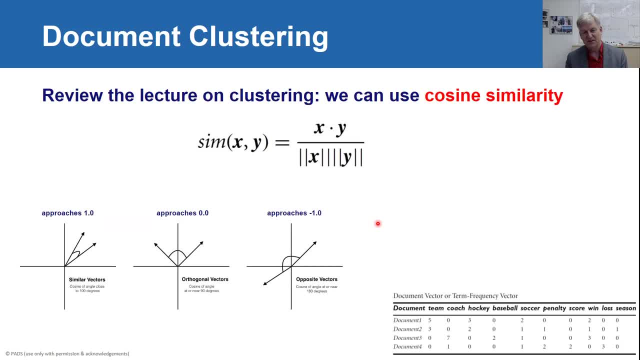 because if you think of that in terms of a vector, then i have two vectors that are, in principle, pointing into the same direction, but because one document is is twice as long as another document, the vector is twice as long. so there would be a big difference if we would just use things like the euclidean distance between these vectors. so that's why 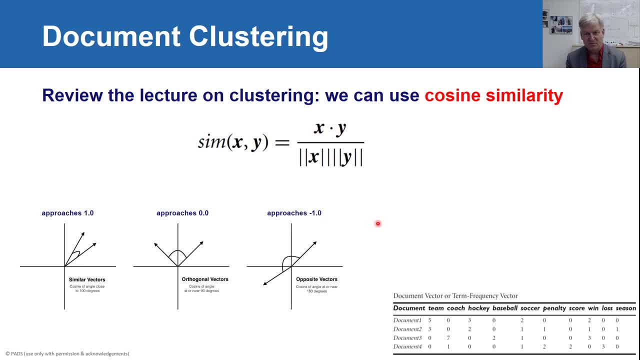 in the context of of text mining, we often use the cosine similarity, and you have seen this notion before, so this leads to so this, this metric: if i have two vectors each representing a document and they point into exactly the same direction, then they have a similarity of one. 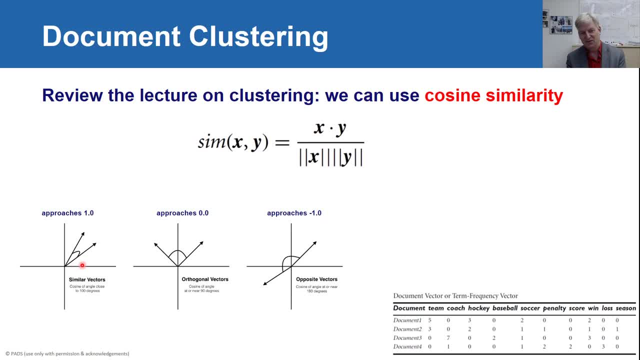 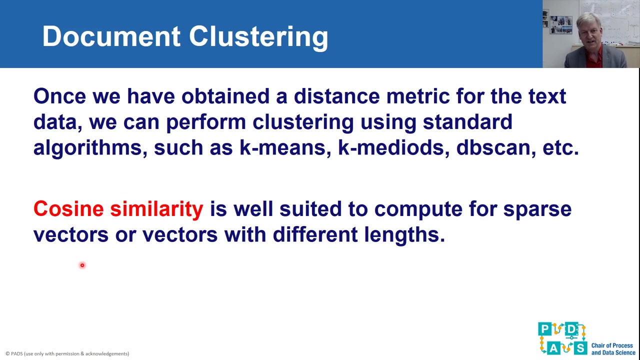 if, uh, they are, let's say, completely orthogonal, if we look at their vector representation, then it's zero. if they are pointing completely in opposite directions, then it would be be minus one. whether that is possible depends a bit on on the representation that you have. so that's why cosine similarity is better suited than, for example, euclidean distance or manhattan. 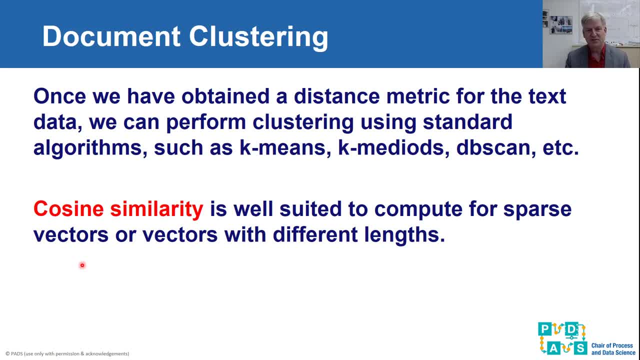 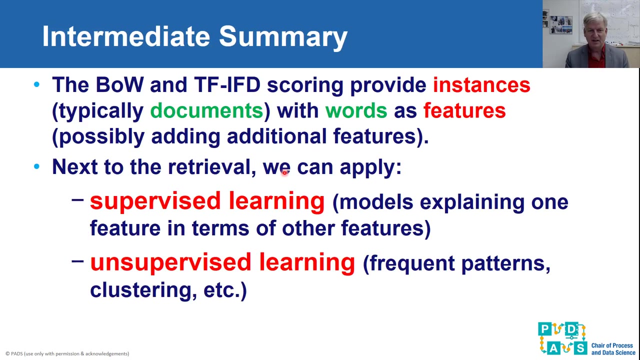 distance. but these are all things that you have seen before and i i'm convinced that you can now see how this immediately can be fed into any clustering technique, because you have the vector representation and you can pick different distance notions. so what we have seen so far, we have seen that we can, from text, generate supervised and unsupervised. 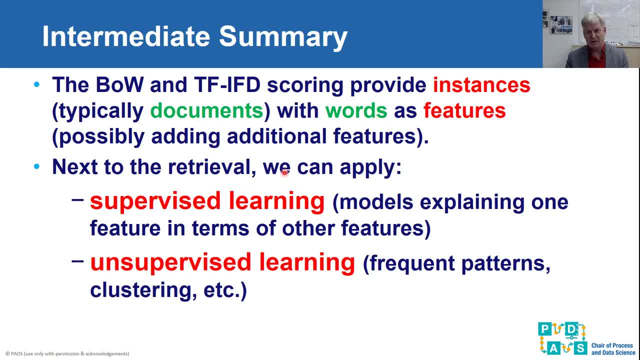 learning problems- we have seen that in the mapping that we did- is that we have a corpus that consists of documents, the documents are instances, and then we have words and the words can be considered as features and there is lots of pre-processing needed to ensure that the collection of words, the collection of tokens that we have, is the right one. 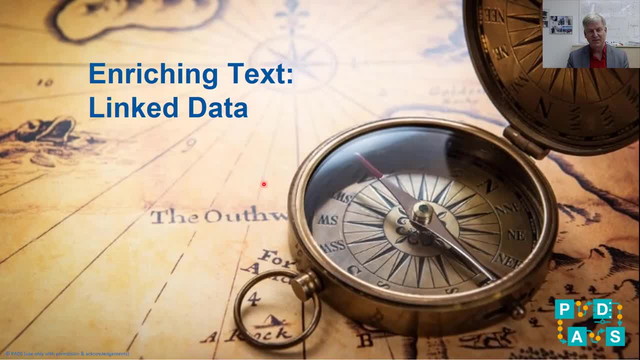 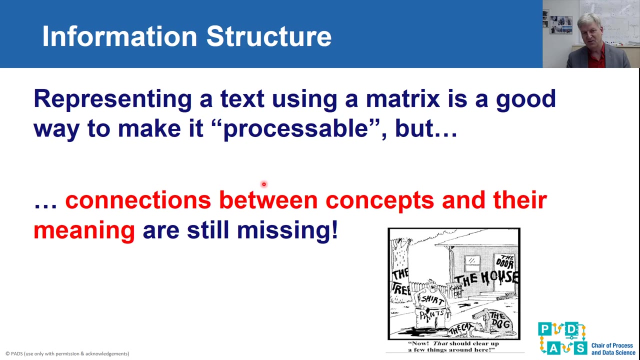 and that's what i have explained so far. but we are not there yet, so we are still have difficulties capturing the semantics of of what documents contain and what they mean. so we have seen that different words can mean the same thing, but also that the same word can mean different things. so 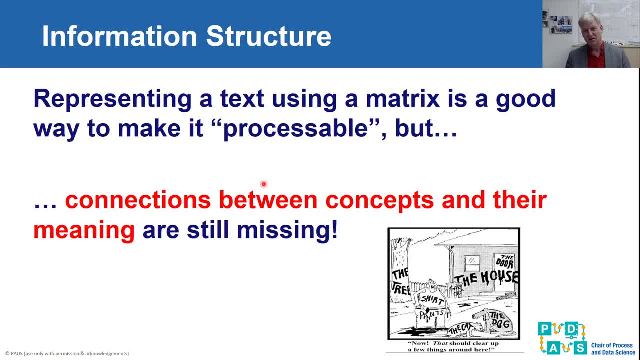 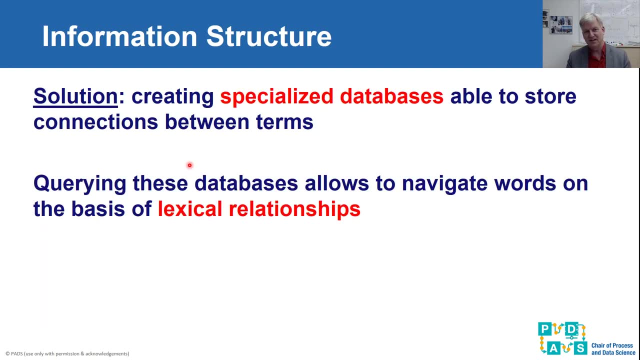 you could try to annotate all these pieces of text, but many of these things are reusable. so this is where semantics come in, and things like the semantic web play an important role. so there are we are. we see a movement towards having databases that are not just storing the syntax. 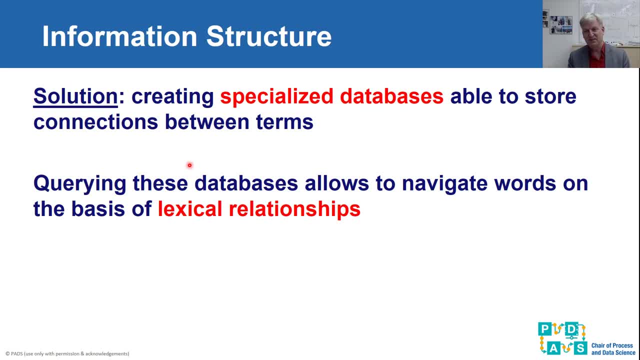 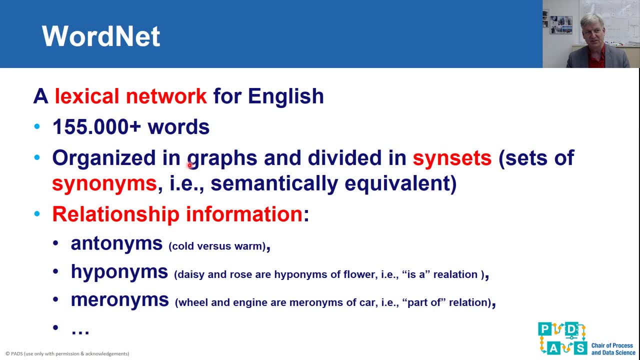 but that are also storing in some way the semantics and the connections between things, and this is what i would like to talk about, let's say, at the end of this lecture. so an example of, let's say, attempt into this direction is a wordnet. it's very famous. so wordnet is a lexical network that contains many words. 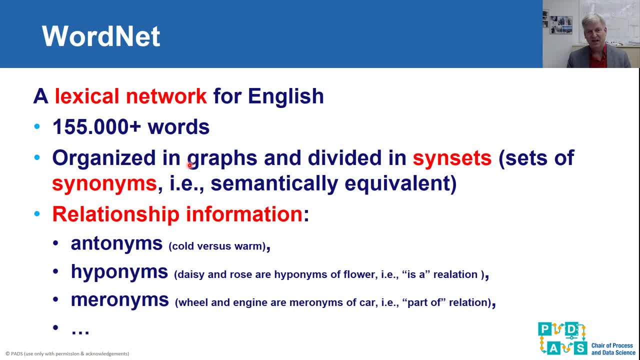 similar things can be found in other languages, and the words are grouped into, let's say, sin- sets, and these are sets of, let's say, meanings of words that are somehow semantic equivalent, and so you try to bring words that can have a similar meaning together into a particular set, and then you try to establish, let's say, relationships. 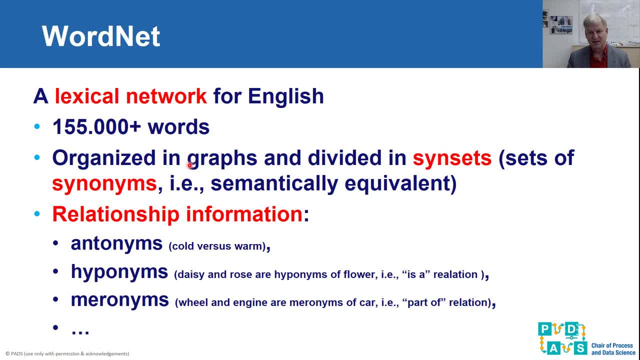 between these different sets and the different words. so there are relationships that say that there is an antonym and so that things have an opposite meaning: cold versus warm, high versus low, big versus small. you also have the IS-A relationship, so you can have hyponyms, as daisy and rose are. 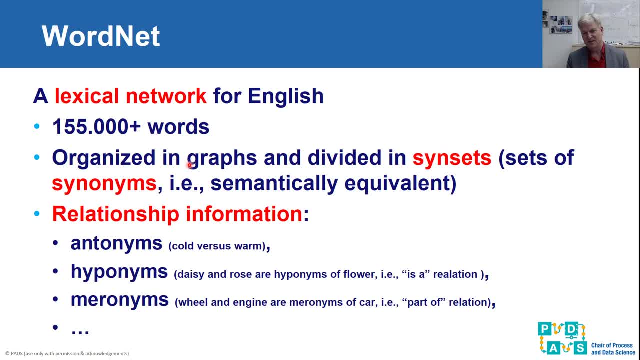 types of flowers. but you could also say: I don't know that Porsche and a BMW are cars. so you can express such relationships that I don't know how to say those things. if you sort of have the same, They are all there in WordNet. And you can also indicate things that are not, let's say, specializations. 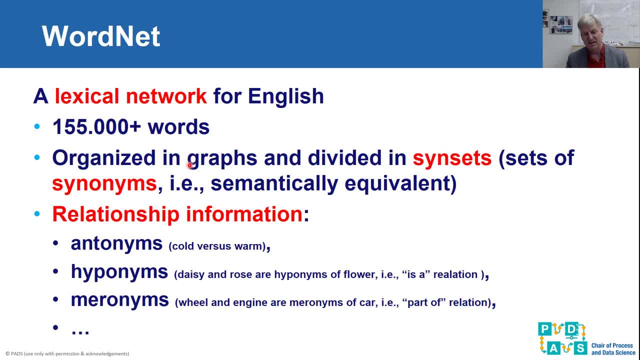 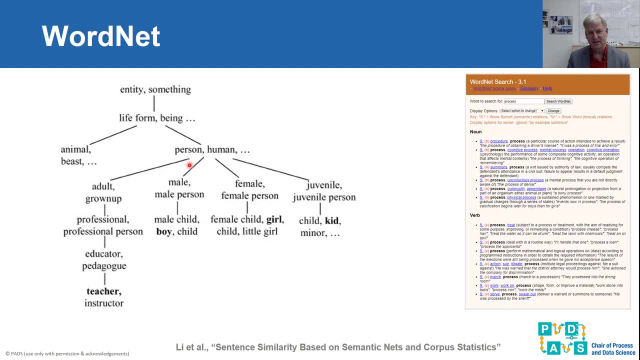 like an is-are relationship, but there are part-of relationships, So that the car is composed of an engine, wheels etc. So in such a lexical network you can basically store these relationships. Here there is an impression, And so here you see a graph at a higher level. 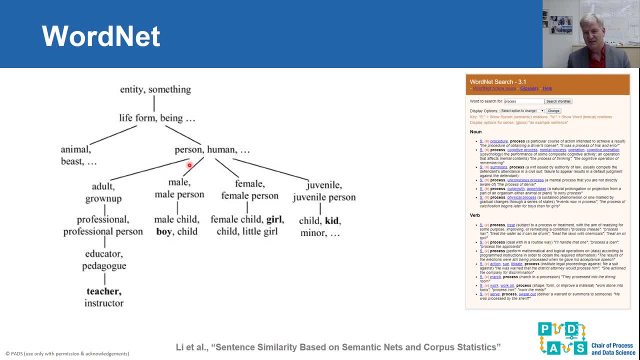 On the right-hand side you can see, for example, the different meanings that the word process can have. So it can be a noun, it can be a verb, but also within noun and verb it is referring to different sin sets. 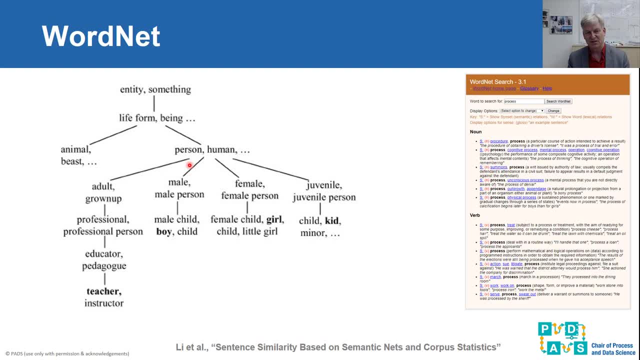 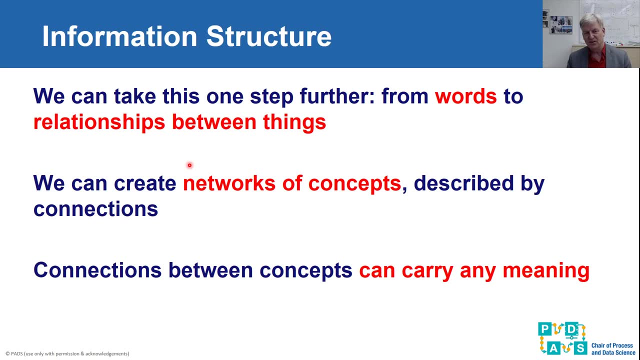 And again these sin sets try to capture the semantics of things. So these are all attempts of storing the semantics of words, with all the problems that I indicated before, And you can organize them in networks, and WordNet was already an example of that. 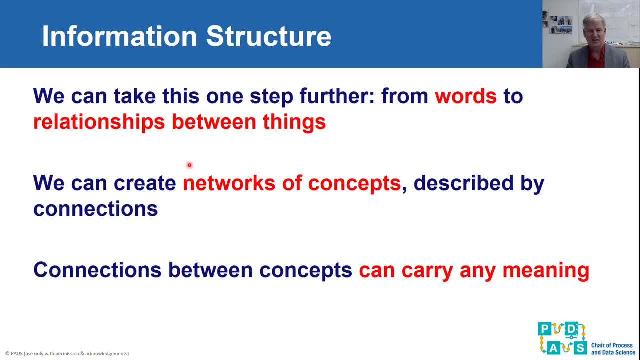 And the connections between these words can again have a meaning. So before in WordNet there is a fixed meaning like two things mean the opposite or two things mean that that one is a specialization of the other. But in principle you can also define your own relationships. 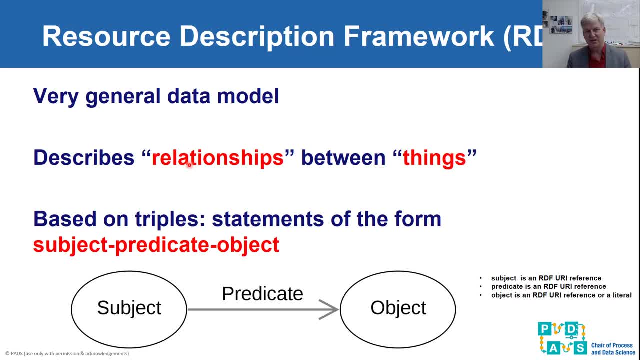 And this is where you end up with representations like, for example, RDF. So RDF, you can think of it as a supergeneral data model that describes relationships between things using a fixed triple structure, And so that is linking a subject to an object through a predicate. 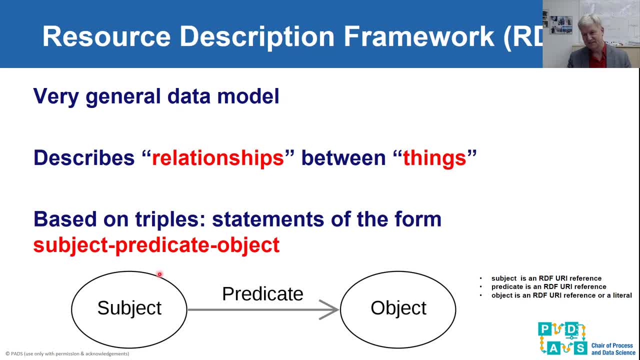 And it's important to realize the way that we will talk about this later. you can think of the subject as a kind of URL, And so this is called an RDF URI, but think of it as a URL pointing to some website. Then there is a predicate. 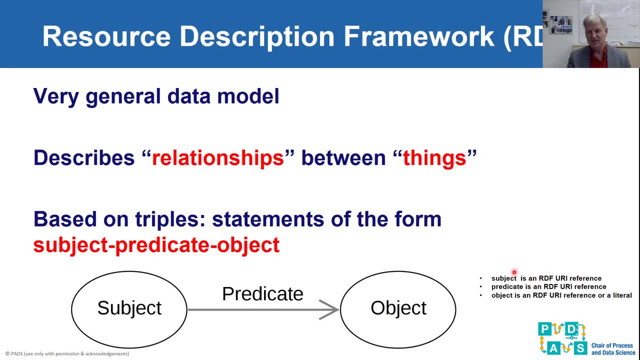 The predicate also has such a reference. And then there is the object, and the object can also be a reference, like a URI, Or it can be a literal, So for example, a subjects could be a will, The predicate could be age. 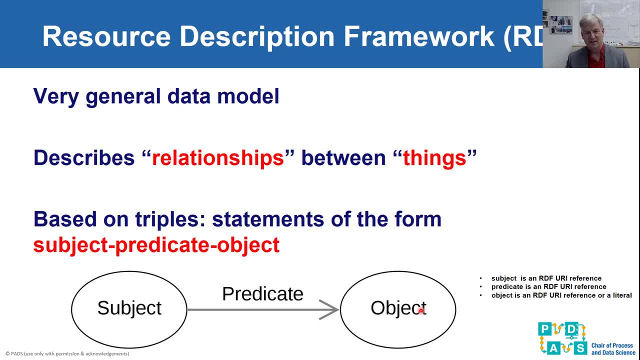 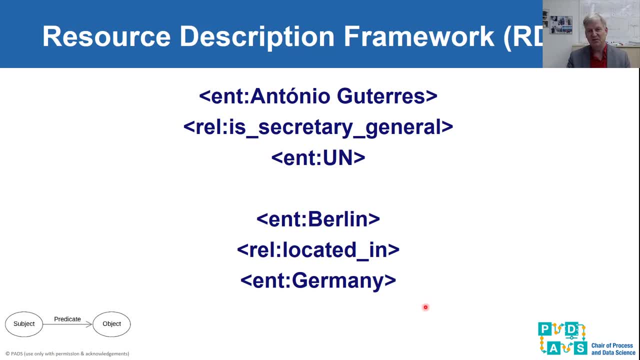 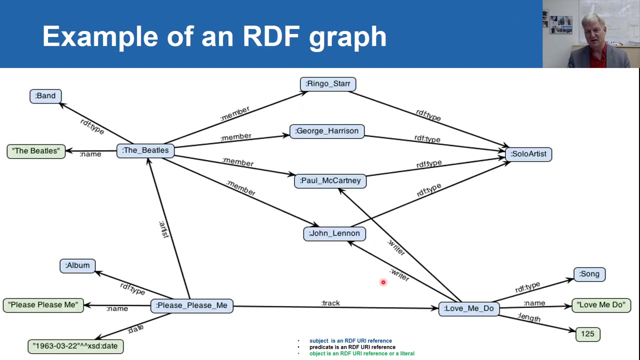 And then the object could be, for example, a literal like my age. So just to provide some examples in RDF, these are two RDF triples that are expressing that this person is the Secretary General of the UN and Berlin is located in Germany. So these are the triples that you normally show graphically. Here you see a whole network and then you can see why people talk about things like the semantic web and often use terms that talk about graphs and nets. 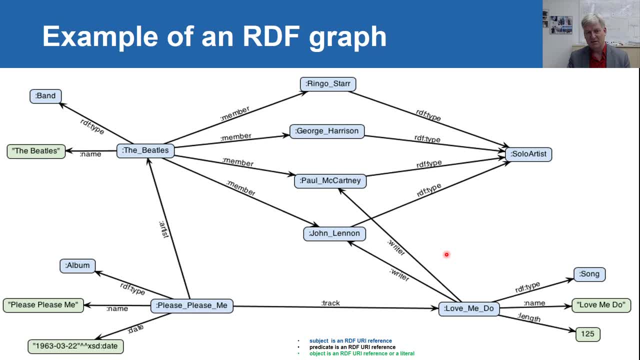 Here you, for example, see an RDF graph about artists, songs, etc. So the things that are in blue are, let's say, things that play the role as a subject or an object that has. but they have in common that the blue nodes have a so-called RDF URI reference. 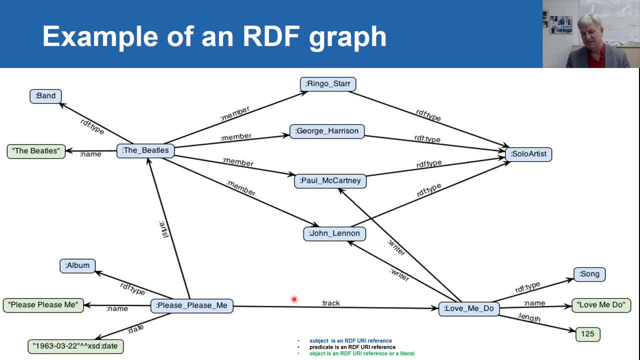 So there are unique entities represented by such a URI, The green nodes. they always play the role of being an object and they are represented by a literal So also. for example, song here is also playing the role of an object in this relationship, but it is a URI. 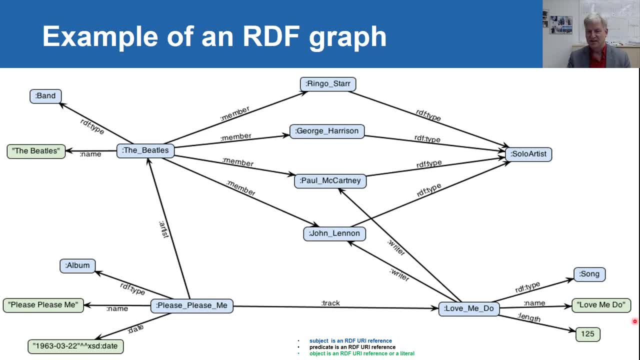 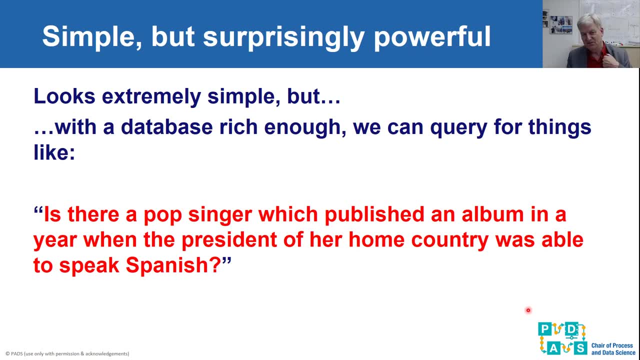 Well, this title of the song is a literal, So you have pointers and values, And this is super simple, But you can. there are all kinds of query languages over such graphs and they allow you to, let's say, automatically answer questions like the ones that I see here. 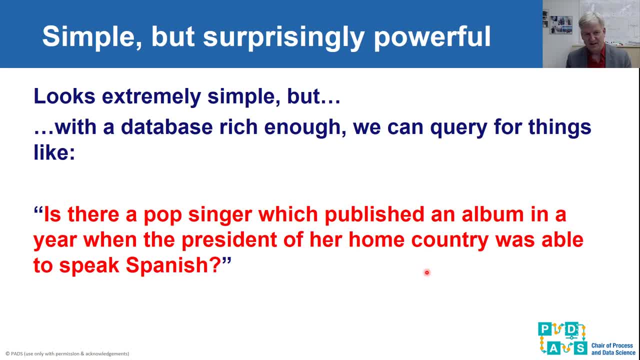 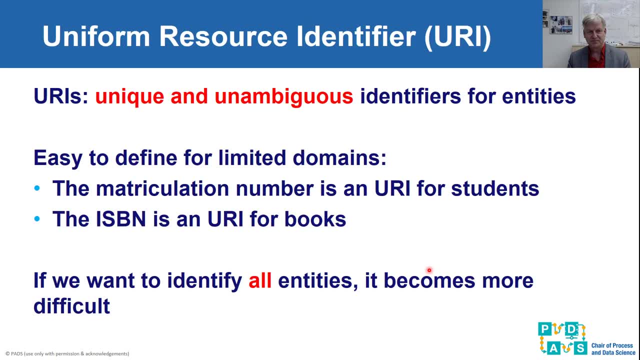 And they are basically answered by, let's say, doing queries over such a, let's say, an RDF graph. So these URIs play an important role. They are unique identifiers. Uh, you cannot just say oh, it can just mean one thing. 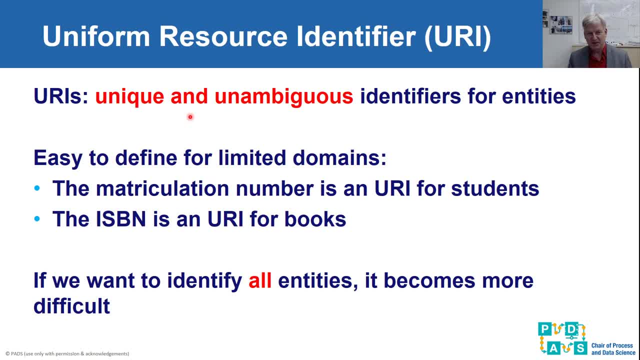 So it cannot be like uh like the word process that we had before, that can have like 10 different meanings. Now, URIs are unique. They refer to something that is, uh an ambiguous. So there is a one-to-one correspondence between the URI and what it represents. 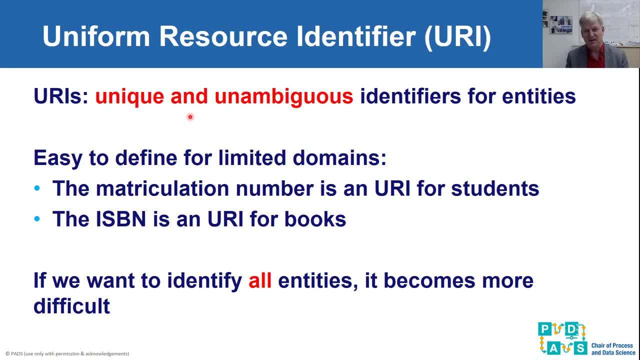 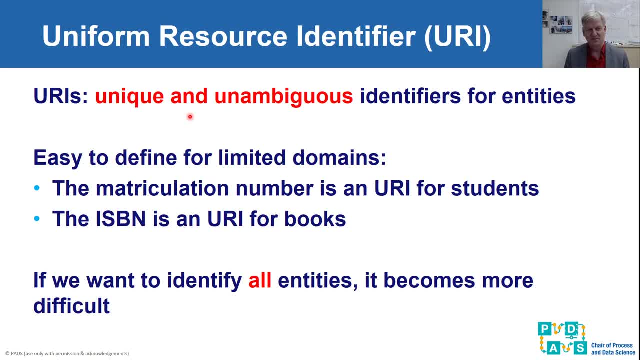 like the things have multiple URIs, so there's a one-to-one connection, And so for some domains this is very simple. So, for example, if you look at books, they have an ISBN number and you can think of that as a unique identifier for such a book. 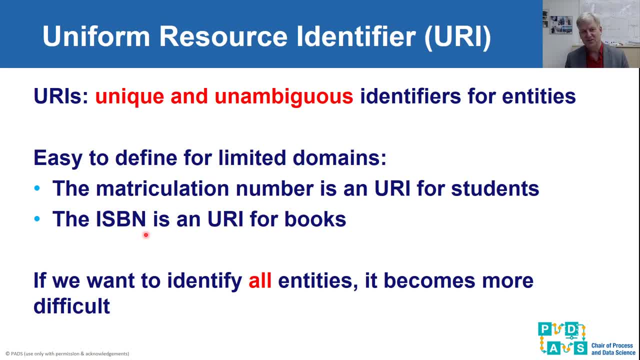 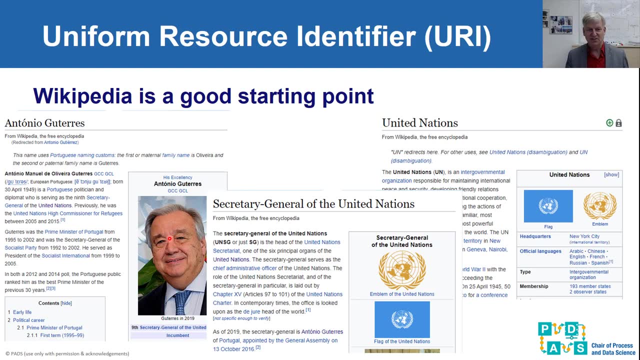 If you're studying here at the university, then your student number is another example of a URI. We, of course, want to do this for all entities in such a way that we can reason about this. Partly this already exists and is there, and the idea of, let's say this part of my lecture is: if you're doing text mining, 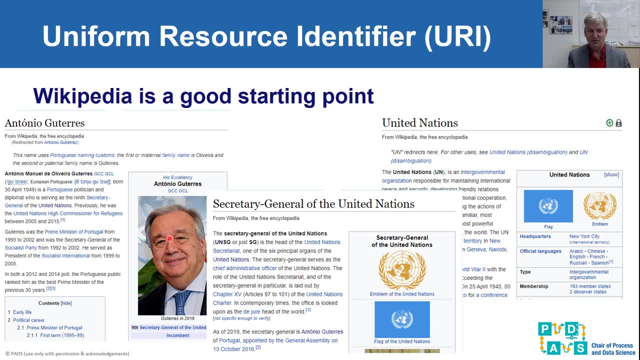 to use the combination of, let's say, resources that are already available and this unstructured text, And this is a very powerful combination And we are still at the beginning of seeing the development of that. So if you look at Wikipedia, then article entries in Wikipedia can be seen as URIs. 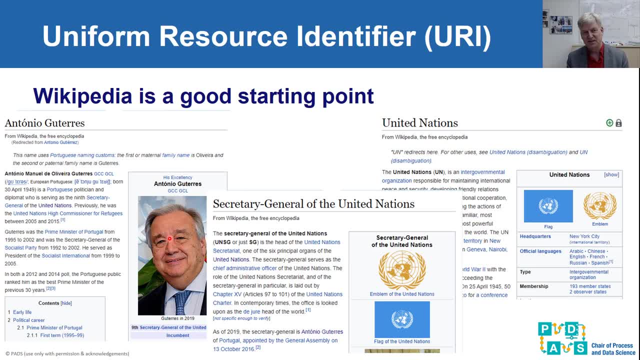 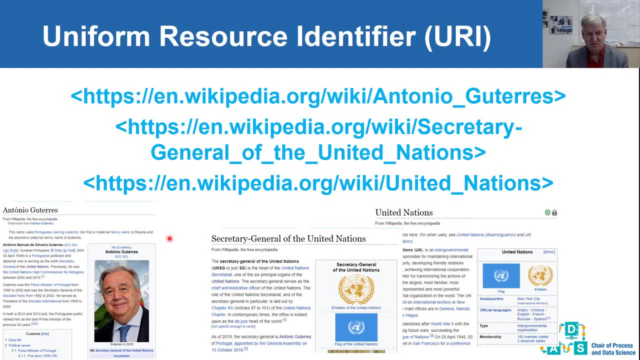 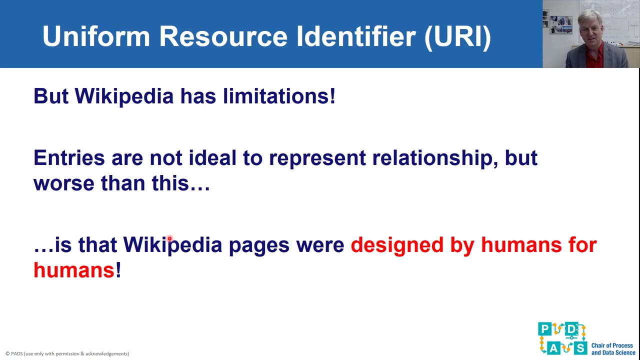 And here I'm using the same example as the RDF triples that I showed earlier. So here you can see the triple that we had seen before, but now I like the URIs refer to Wikipedia pages. Of course, Wikipedia has the problem that it was not made for machines and made for reasoning. 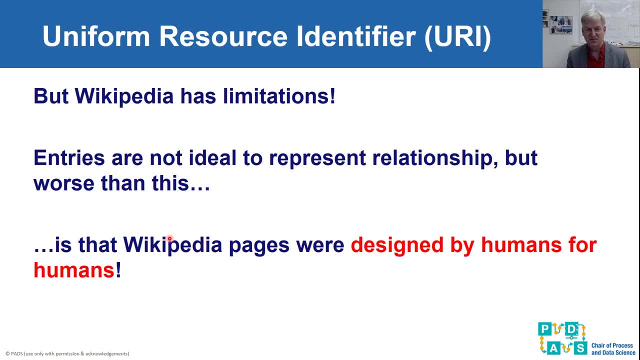 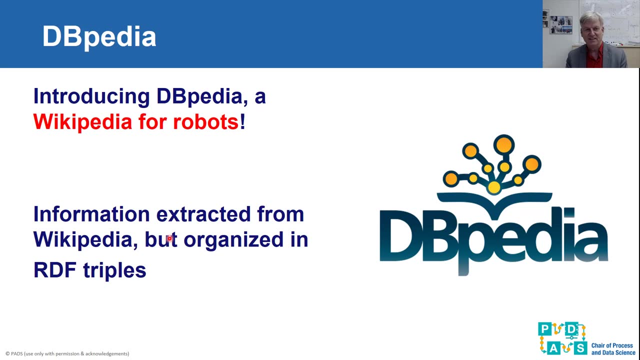 but it was designed by humans for humans. That is why, although it is a very good starting point for, let's say, general purpose knowledge, there are, let's say, variants of the idea of Wikipedia, that is, that are more intended for robots, as a DBpedia, it's like a similar initiative. 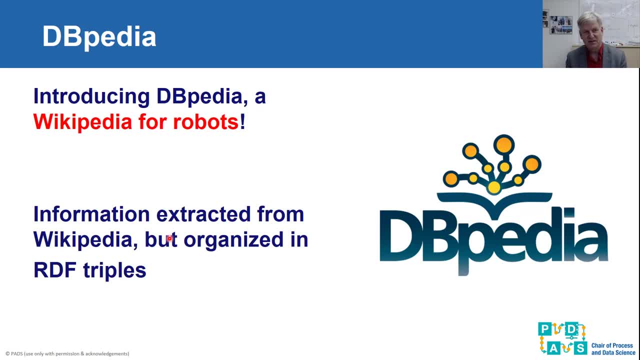 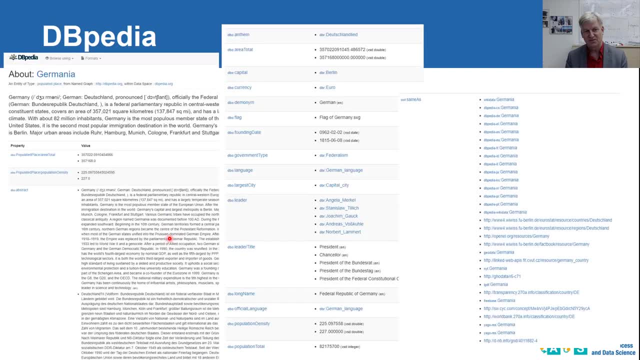 but then organized in terms of RDF triples and intended for robots, that reason, over such networks. So here, indeed here, you see a fragment of this. As I said, it looks the same as Wikipedia. as I said, it looks the same as Wikipedia. 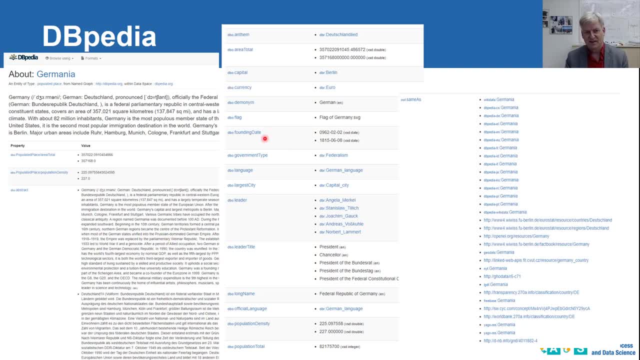 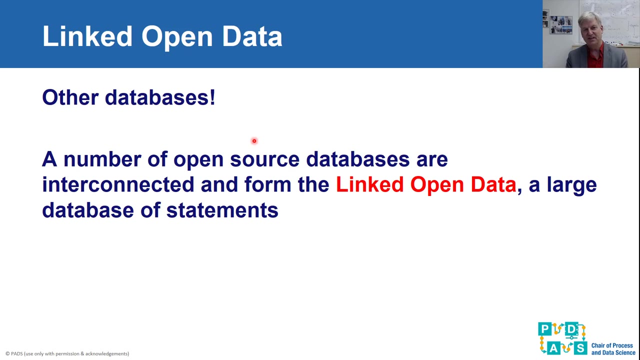 as I said, it looks the same as Wikipedia in a way, but let's say, these links and the objects have now these URIs in such a way that one can reason over this. So the idea of linked open data is to exploit the fact that there are, let's say, multiple sources of such information. 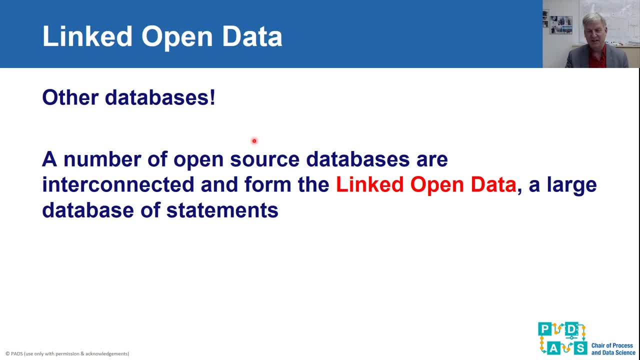 And so Wikipedia is one, but there are many, Let's say, sources of information that, once you can connect them, they are very powerful, And the key element in making this work is that somehow these URIs are maintained over these multiple databases. 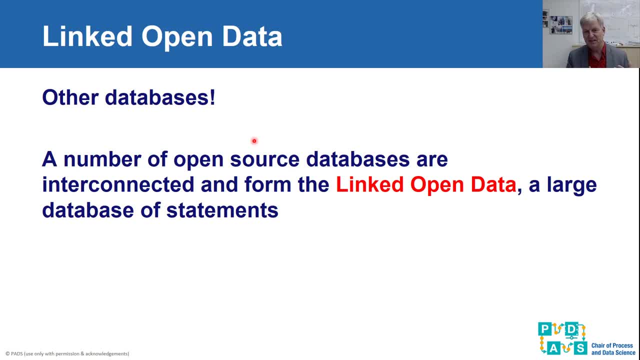 And that is the challenge: that if I have a Wikipedia representation or a DBpedia representation and I have an internal SAP server, I can't do anything about it. I can't do anything about my entire work, And this means that I don't have an internal SAP system. 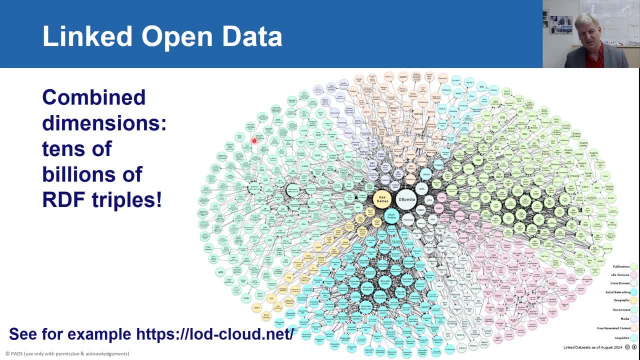 that I can somehow connect them to each other, And this is the idea of linked open data, and this is the idea of linked open data that is, providing data that is publicly available that you basically can reuse. It is in this lecture on text mining. 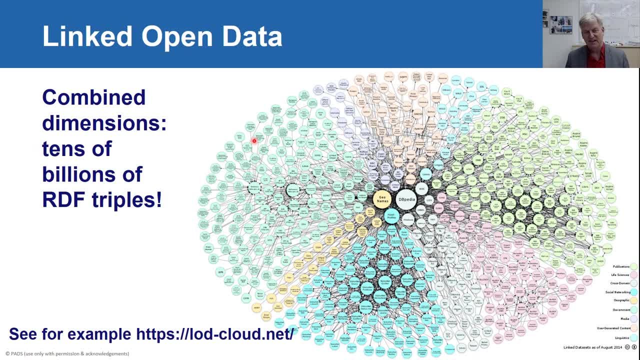 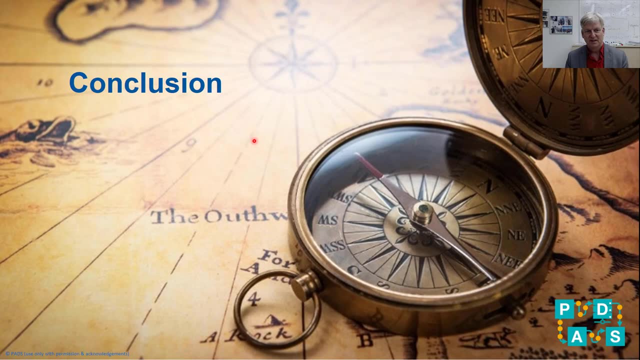 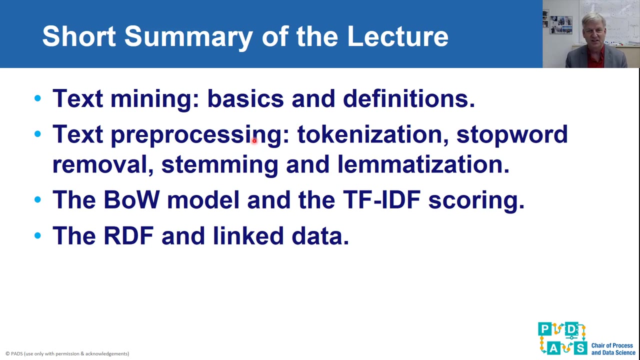 because if we look at the words in a text, They are in principle pointing to things in the space that you see here, And in the future we will see much more, let's say, semantically annotated information sources. So in this lecture we gave like a first initial introduction to text mining. 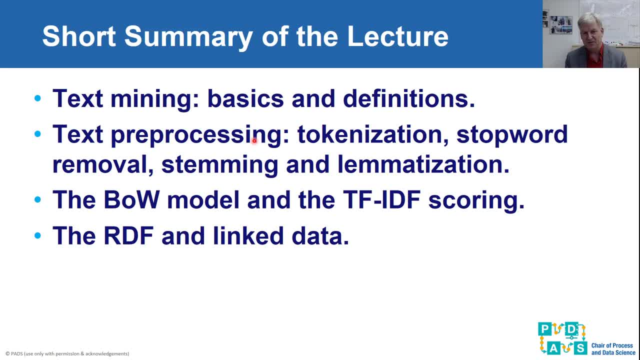 We spent a lot of time on text pre-processing. As I indicated, this is not something where you can say, okay, it has to be done exactly in this way. We highlighted many problems that can be addressed, but there is no optimal solution. 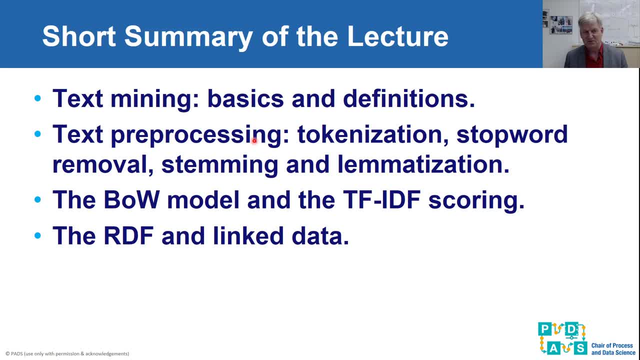 And that's why you always have to realize that you are working with things that are, let's say, not 100% deterministic, But, as I also indicated, they work surprisingly well. So, for example, if we are doing information on a large set of documents and we use the bag-of-words model combined with TF-IDF scoring, we get the documents that we are after. 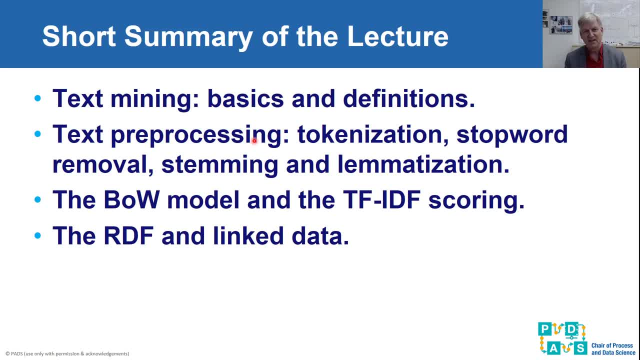 So it simply works, despite, let's say, all the subtle factors that we have. What we have seen is that, using the bag-of-words model, we can represent things in terms of a feature vector, And that means that we can. 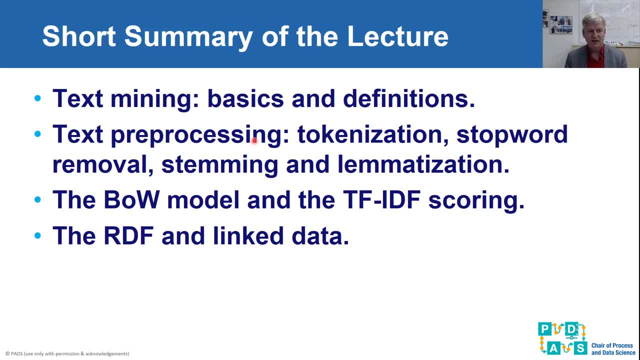 apply all the techniques that we have seen before. At the end I talked more about semantics and that the words that we consider in text mining actually refer to concepts, And if we can link words to these concepts, then that is a very powerful combination. 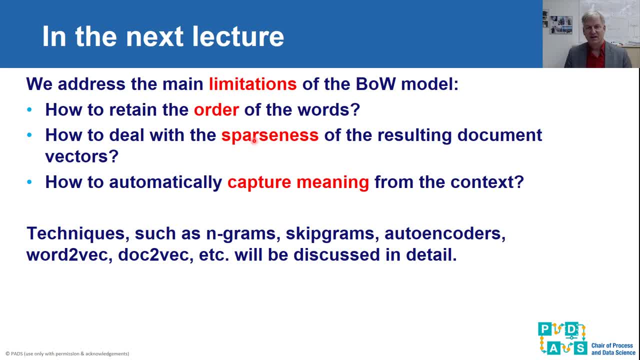 But it depends on the application. So the bag-of-words model, as I already indicated, is basically ignoring the order of words. There is also the problem that if we look at the number of words that can appear in a document, the number of potential words is huge. 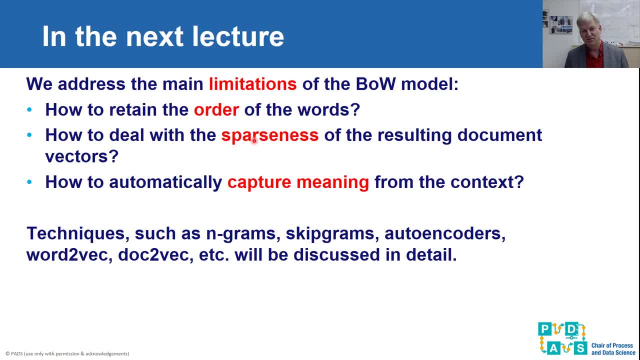 And so, on the one hand, we have the bag-of-words. representation is very big because there are many possible words. We have huge vectors Because the size of the vector is the number of different tokens or the number of different words that we consider.